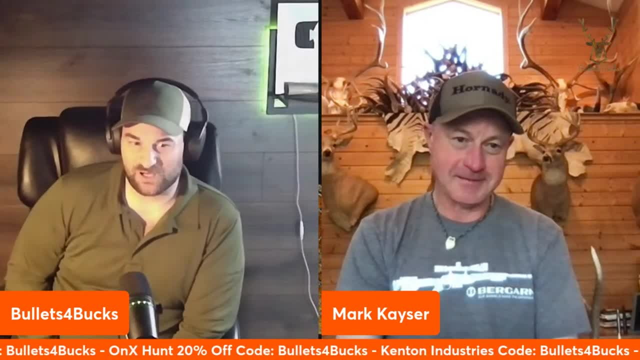 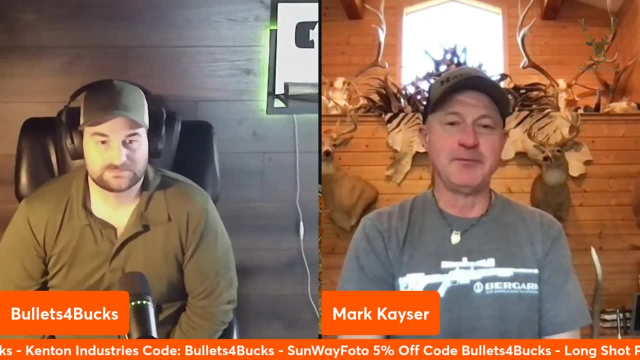 And I saw you were like on or you were the host of Extreme Hunts and some other and I guess maybe on Beretta TV or something. I was just looking at your bio the other day. Is that true? I've been a host of quite a few shows: Extreme Pursuits, I've been the host of 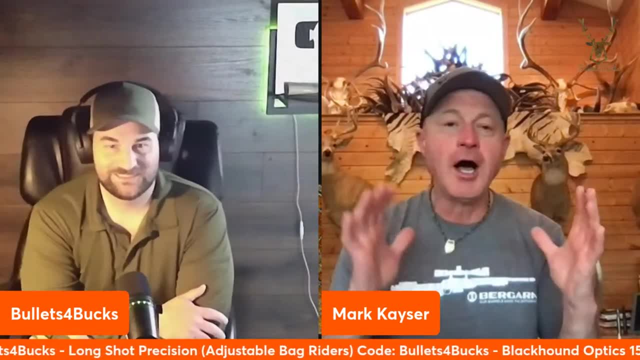 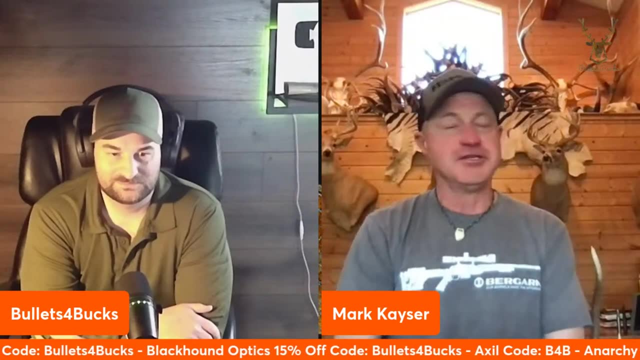 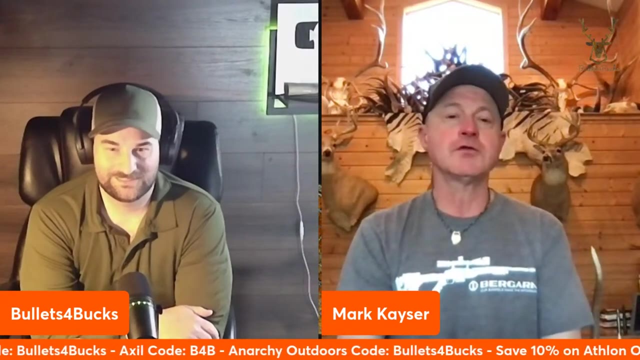 Truck Vault Extreme Hunts. I did a ton of stuff for North American Hunter back when they were, you know, the flagship hunting club And I just loved working with that organization. It was a sad day when they shut down And, as you've mentioned just a little bit ago, I'm also 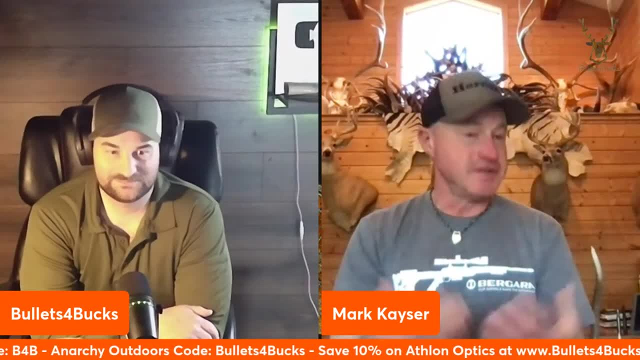 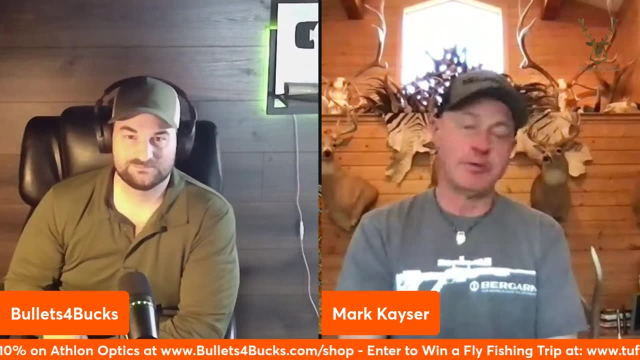 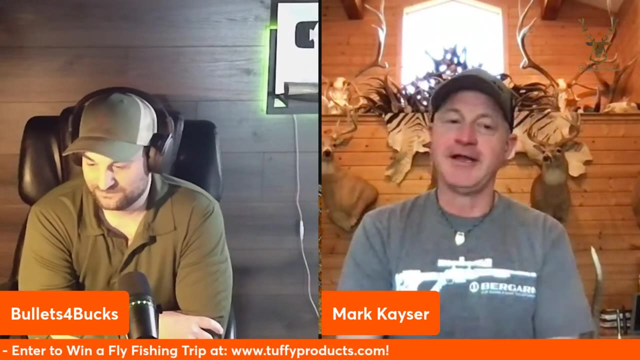 co-host of Deer and Deer Hunting TV, which is on the Pursuit channel. It streams. They have it on their website. You can find it almost anywhere. but I really do love doing that show And I'm a usually do about three to four hunts every fall and pure whitetail hunting, So that really gets. 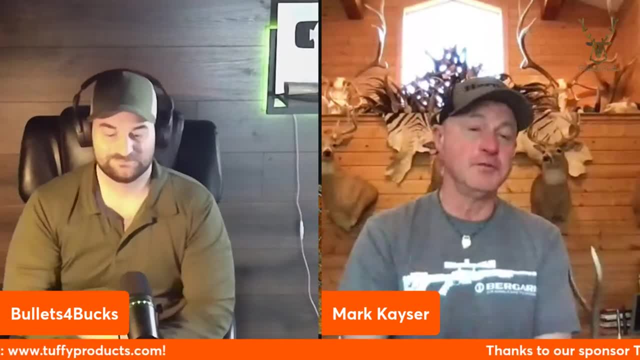 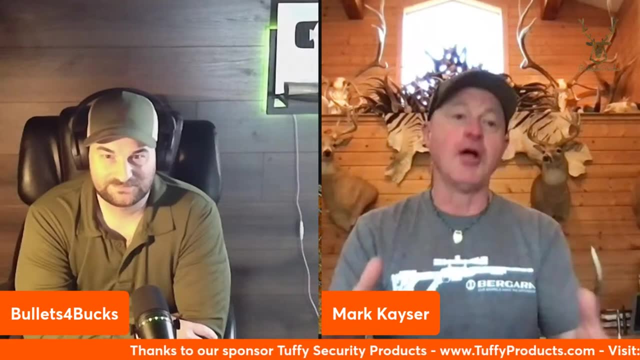 me into the whitetail mood, you know, filming those hunts, Although we do do a few mule deer hunts. They give me some leeway to do that. So that's basically what I do. I write, I blog, I co-host some stuff, do a lot of podcasts like this for different folks like yourself And I. 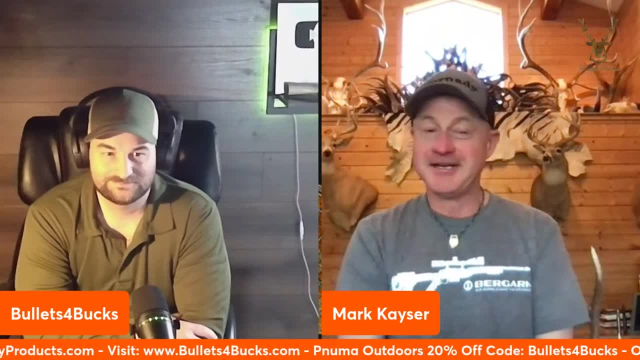 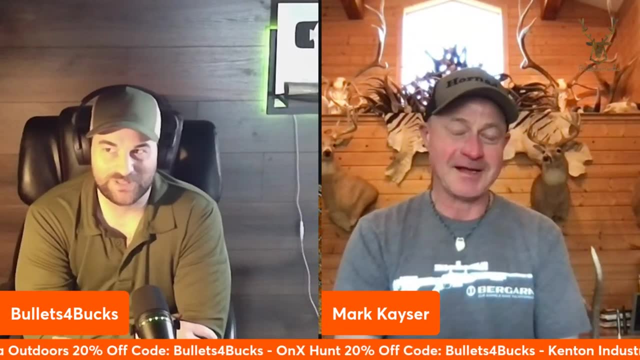 appreciate you inviting me on And I just love to talk hunting. That's my whole life, the hunting life. And you do have a YouTube channel, right, But that's not where. I guess that's probably not where your main energy goes, but you do have one. I just want viewers to know that if they 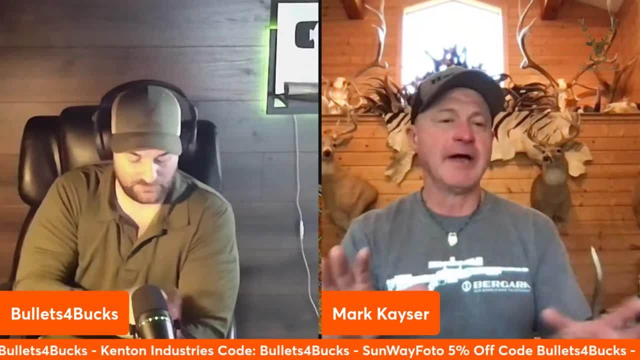 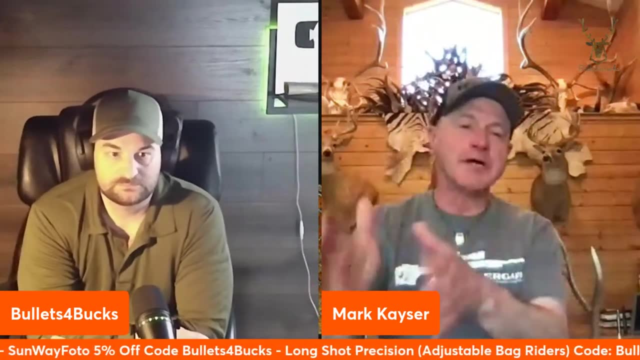 want to subscribe? Yep, They can go to YouTube. They can watch a lot of my old Extreme Pursuit shows, Some tips and stuff I put up there. But if you want the latest little tips, what Mark's doing in the outdoors- and I throw my family stuff in there. I try to do a little bit of everything- Go to 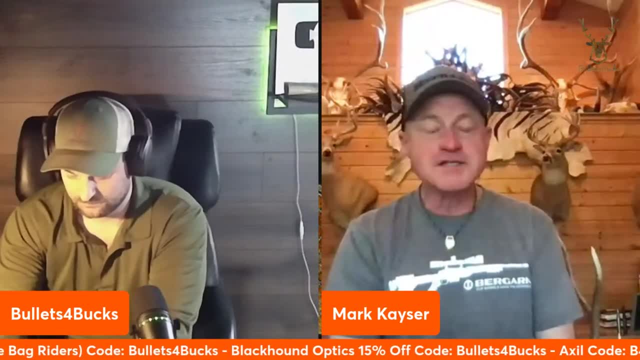 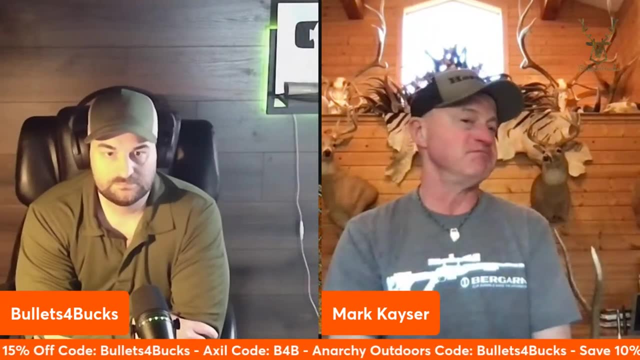 Instagram, Kaiser Mark, or go to Facebook. And if you want to subscribe to my YouTube channel, it's Mark Kaiser. Public Figure K-A-Y-S-E-R. Those two. I put stuff on there every other day, every two to three days every day, depending on what mood I'm in. I also have an account on 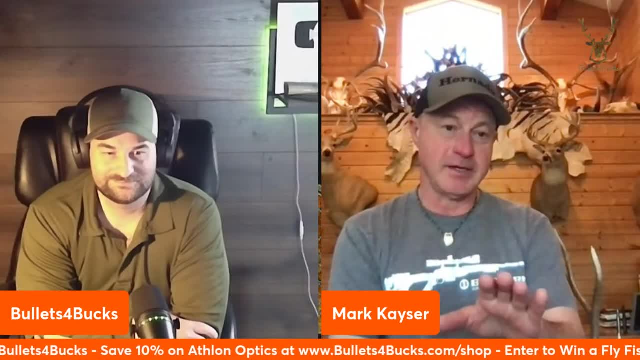 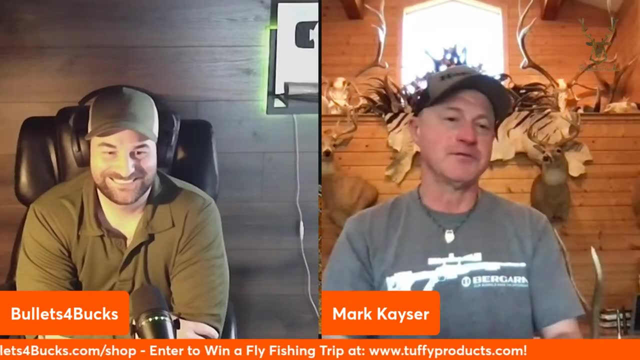 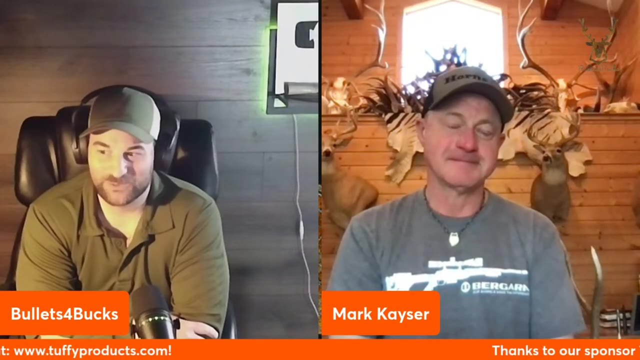 Twitter: Same thing, X- excuse me, Look up Mark Kaiser on X. Basically the same stuff. So if one of those platforms is the one you like, you're going to find almost the same content throughout. Yeah, I still refer to. 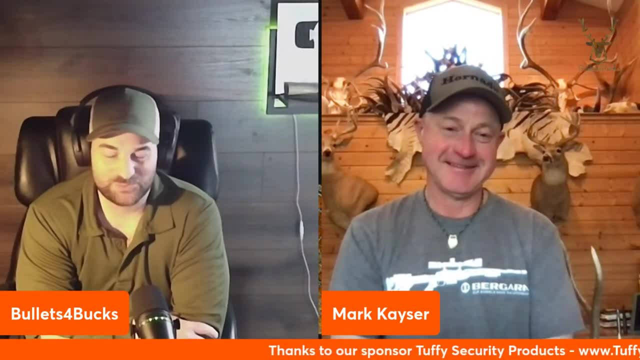 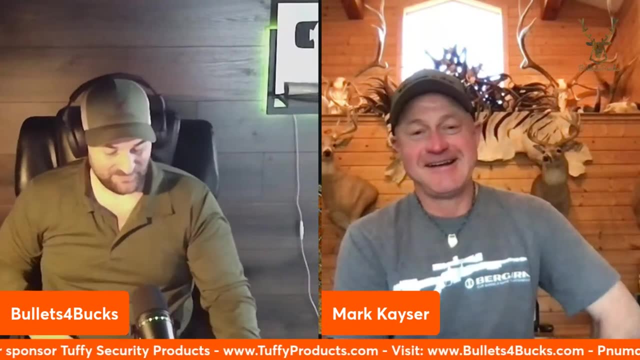 X as Twitter. even when companies reach out to me or something, I think they're starting to be like what is This guy's too old school for us? He hasn't caught on yet. So you're living the dream- or, I guess, every guy's dream, But I know that once you live the dream, it's actually a lot. 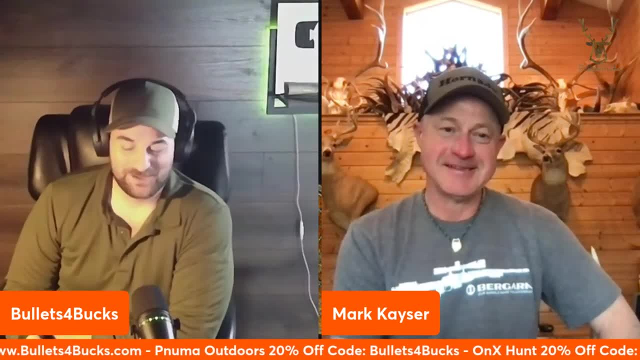 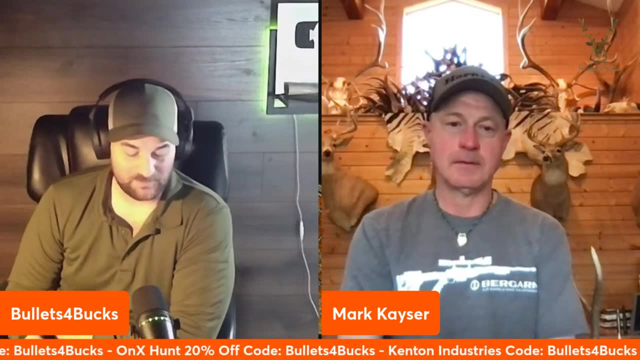 of work behind the scenes And I think people don't understand that. But I guess, to start things off, where did your passion for hunting start? You can say any specific story or it can just be generalized: Where did that start for you? 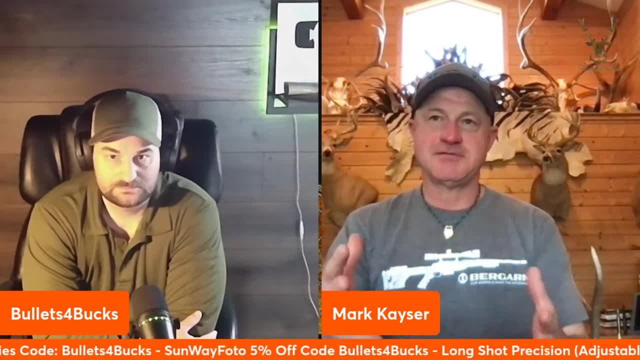 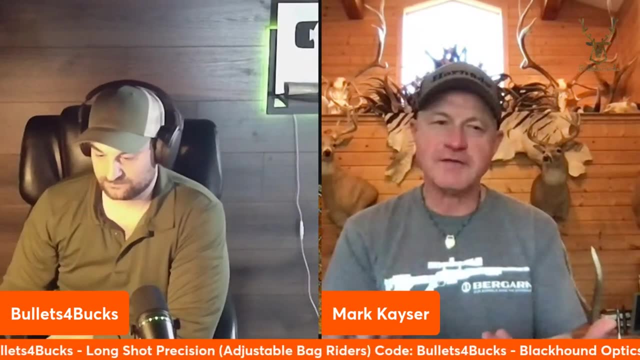 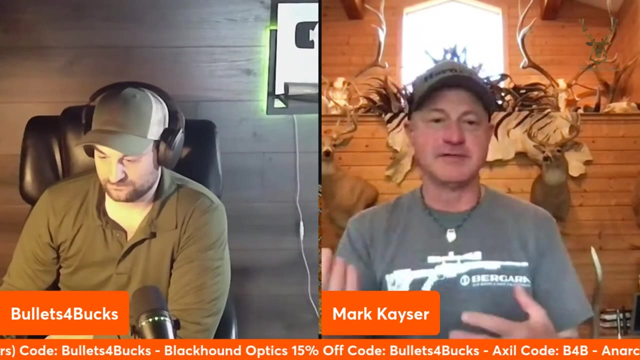 I think, like a lot of people, it's just in you, It's instinctive. So I always had this instinctive nature to be doing outdoor stuff and watching wildlife. I just really truly enjoyed watching wildlife And as a young kid I probably should have pulled some of these out. I've actually 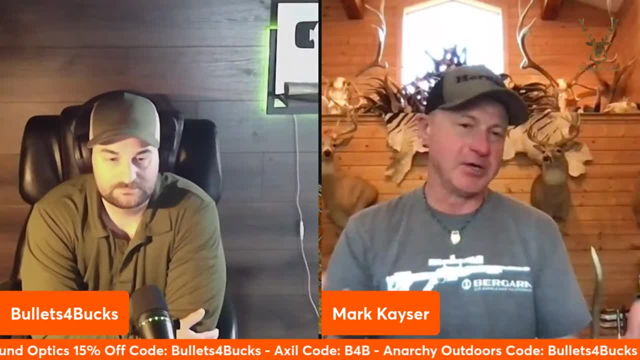 found some old drawings, but I used to draw pheasants all the time. I grew up in South Dakota. as a young kid I lived in Wyoming. Now I've lived here close to 20 years. I've lived in Wyoming for. 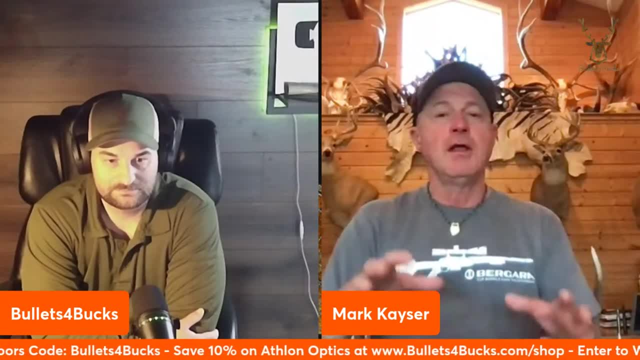 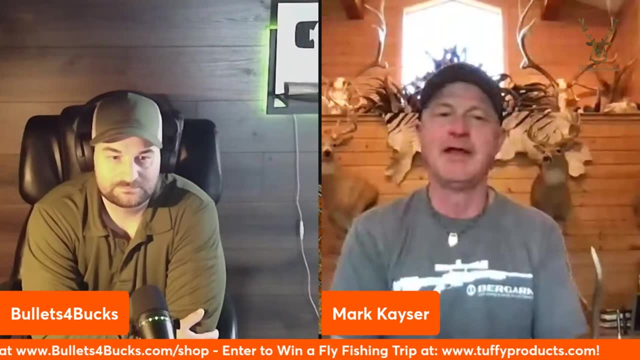 20 years now, Wyoming's home, But I grew up in South Dakota So I just had this instinctive nature. And then my family, my dad, didn't hunt. He did just a tiny, tiny bit, but he didn't hunt. 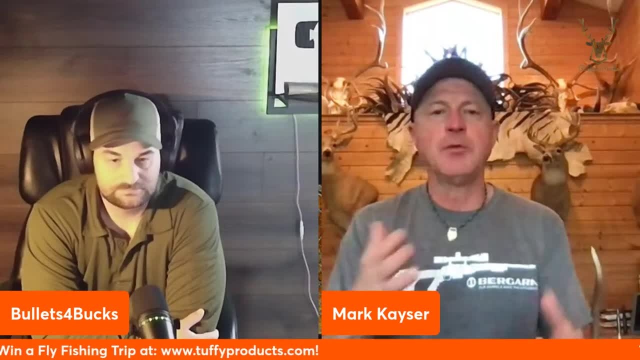 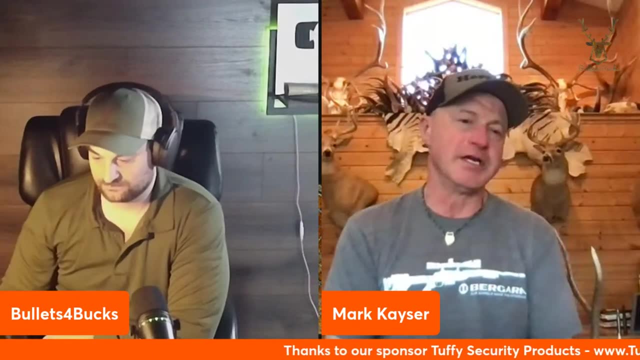 My grandpa did. And my grandpa was somewhat handicapped so he couldn't take me and do a lot of big hunts. But he was probably the big inspiration for me to hunt. But because he couldn't get out in the field and my dad really didn't hunt that much, I didn't hunt that much. 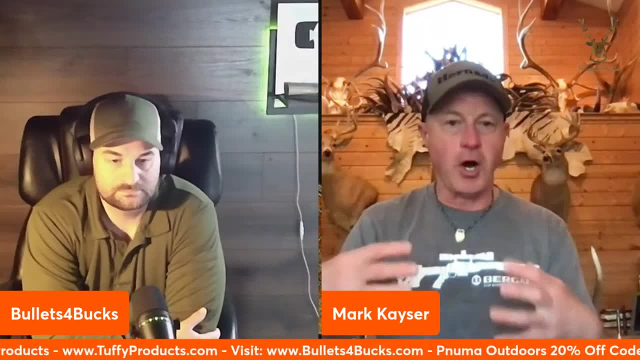 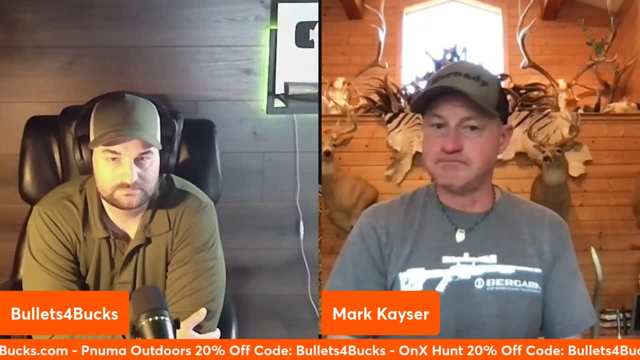 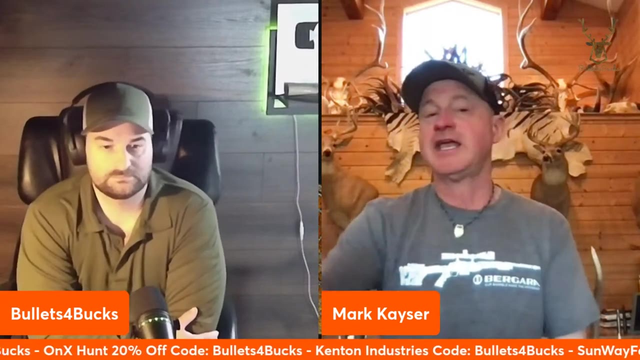 Almost everything I did was self-taught. I just kept trying different things, doing different things. My mom and dad, back in the day and still today, we did it with our kids. You trusted your kids with firearms. It was a tool. It was just like: here's a saw, Go build something. Here's. 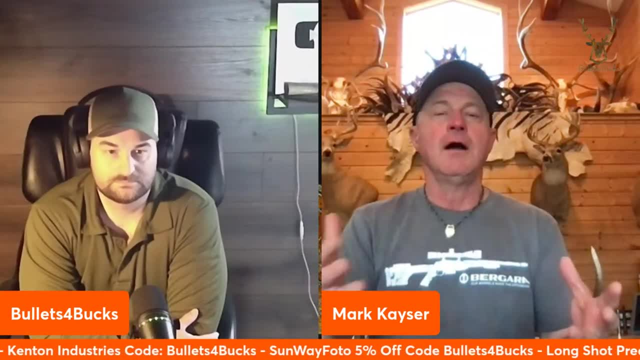 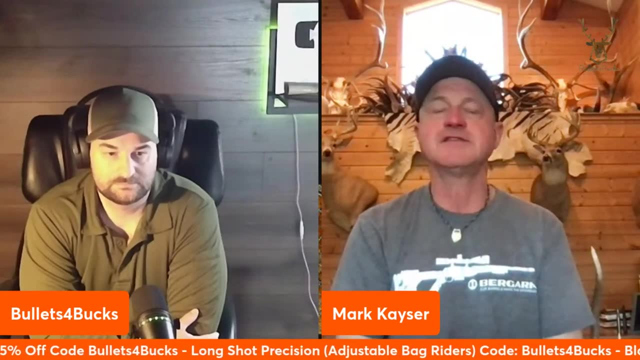 a 410 shotgun Go out and shoot some gophers. So I had a lot of freedom with firearms, although I had good training. I went to hunter safety. My grandpa taught me safety and stuff and just took off hunting. And then what really sparked my hunting? 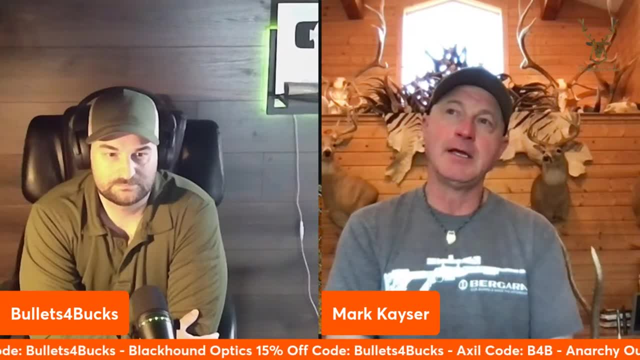 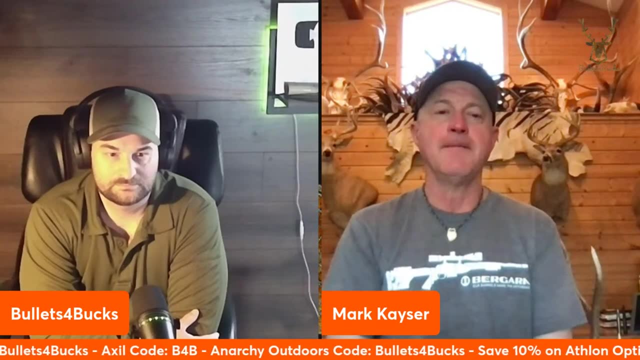 was. I was a freshman, I believe 8th grader, 9th grader in high school And I went to a garage sale and I saw an old Fred Bear compound bow sitting there for sale And I bought it, Didn't. 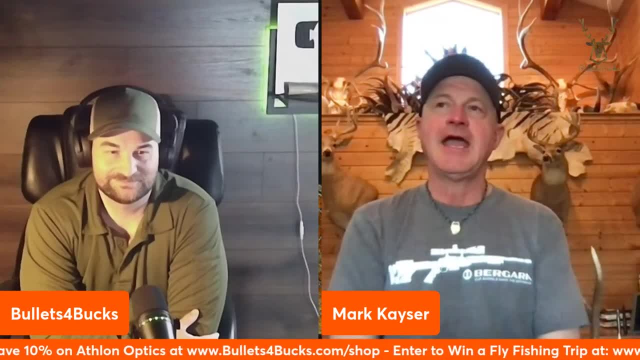 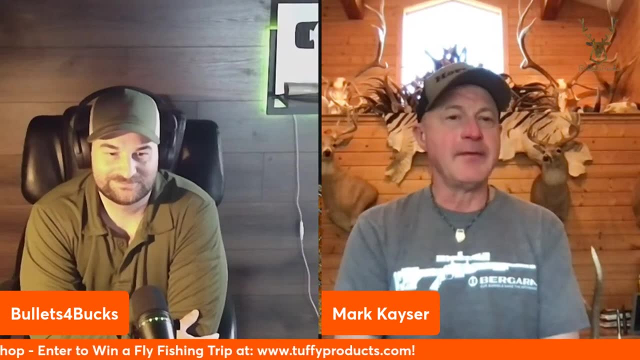 know anything about bow hunting, Didn't know anything about arrows- nothing. And I pieced it together enough and that was it, And I bought it, And I bought it, And I bought it, And that fall- this was in the summer- and that fall I shot my first big game animal anywhere. 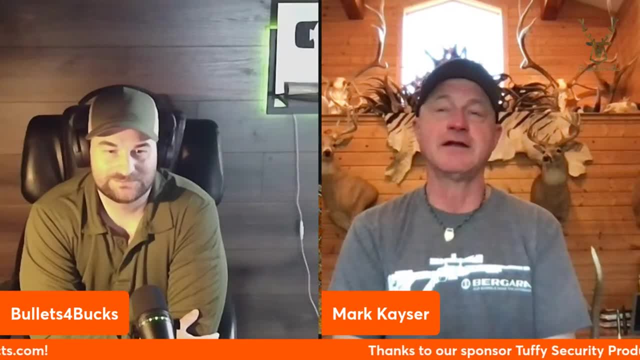 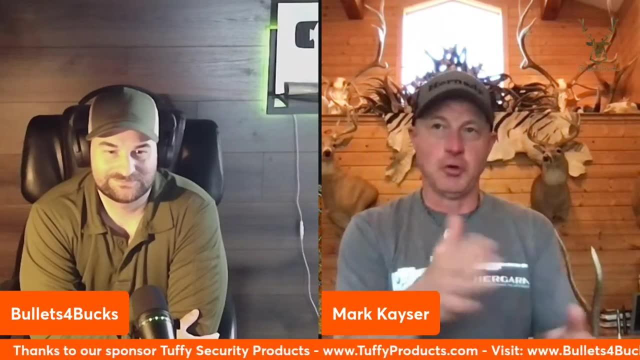 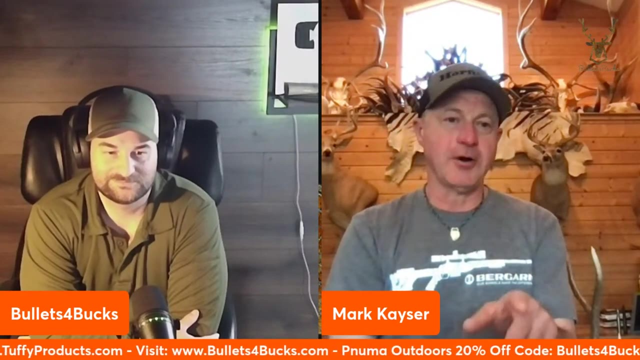 white-tailed deer with a bow And I had rifle hunted a few years, I hadn't gotten one And that really that was it. That mark was going to hunt from then on- And I've told this story before, so if your viewers have heard this- But that night I shot that deer. It was dark when. 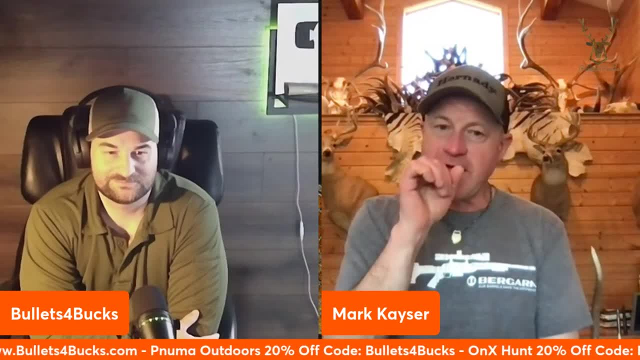 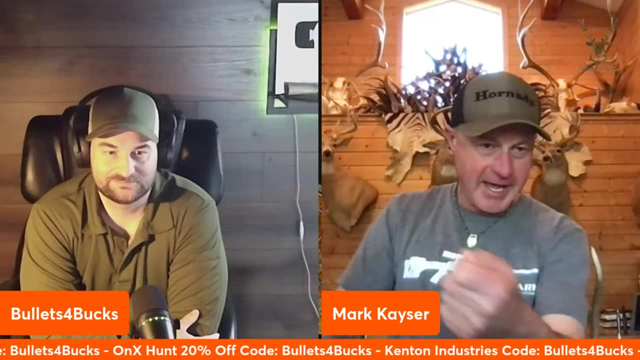 I found him in a cornfield. I drug him out, I put a flashlight in my mouth And I shot him. And I opened up an old, outdoor-like book I had on how to field-dress deer and set a corncob onto that page. 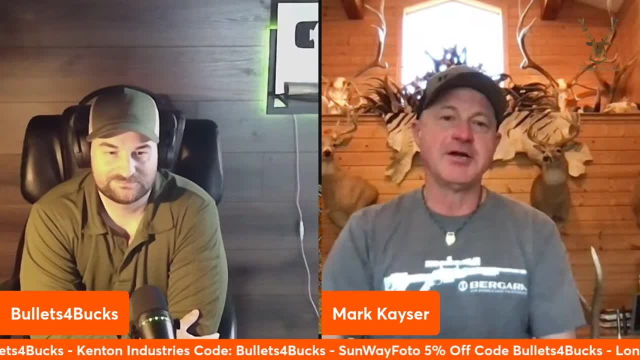 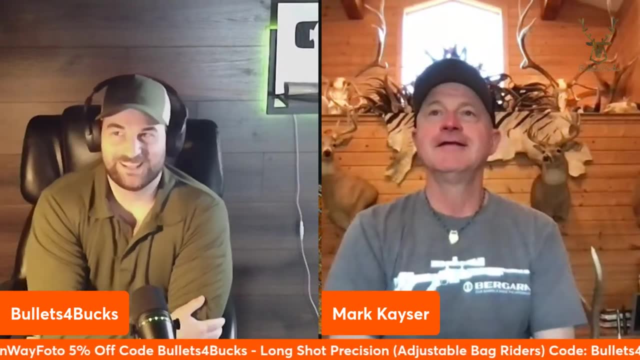 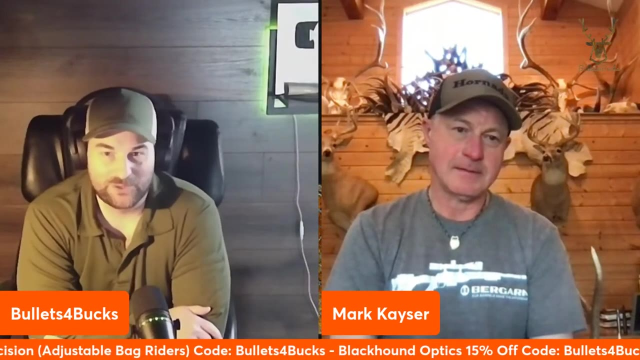 open And all by myself, I field-dressed that deer and got it on the top of my internal scout. by myself. Oh wow, Yeah, Yeah, I mean I can definitely relate to that being essentially self-taught. For me, though, it was more probably off of YouTube videos than books, and 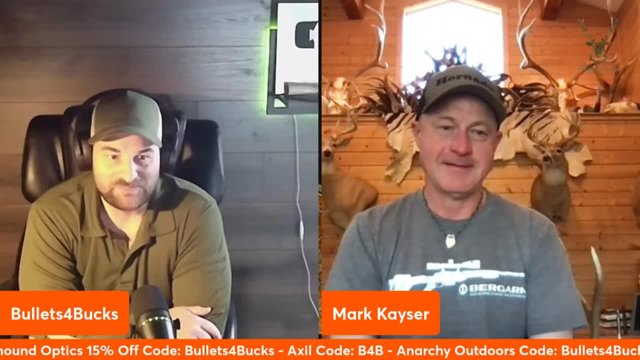 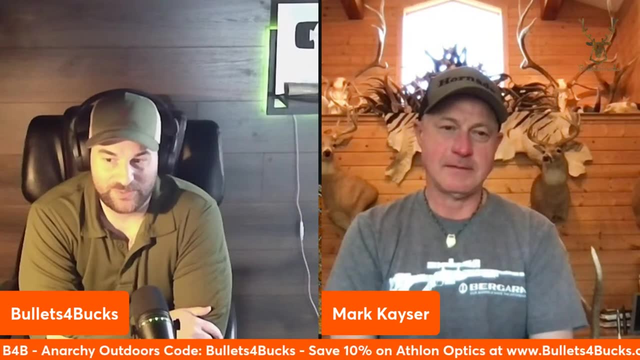 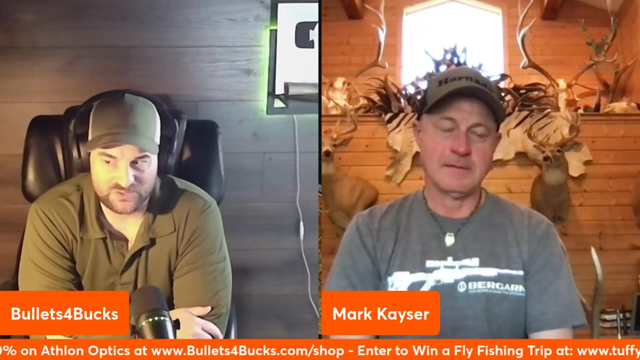 magazines, probably just due to my age, But yeah, I think that's a really cool story about igniting. It kind of sounds like it ignited your passion. That's kind of how I was. The first big game animal I got on my own is really what triggered me into going into it. 110%. 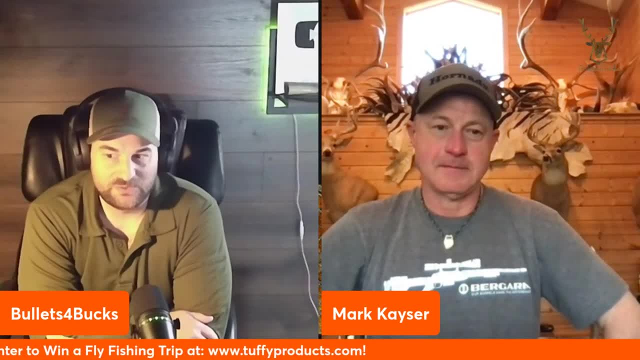 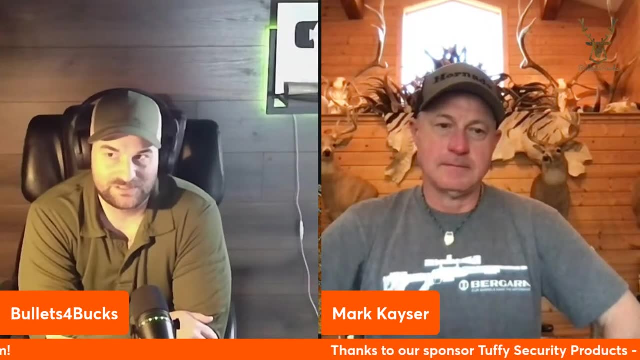 and having that achievement. So I do think that biologically I guess we could say, or I think we all kind of- I think most People have that, like you said, that desire to kind of hunt. I think we have that hunter-gatherer. 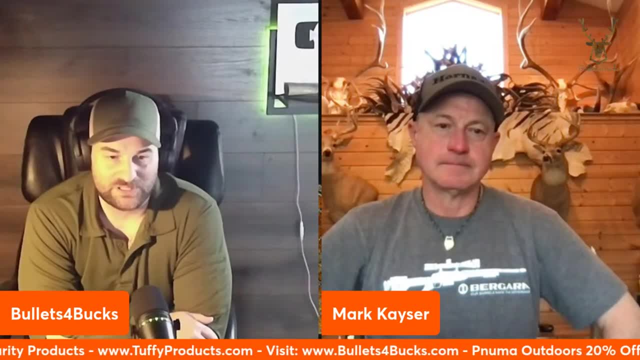 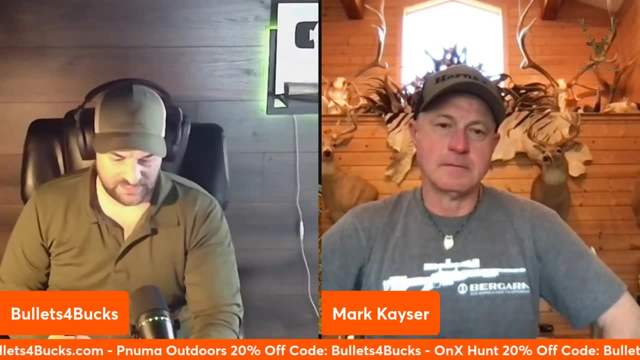 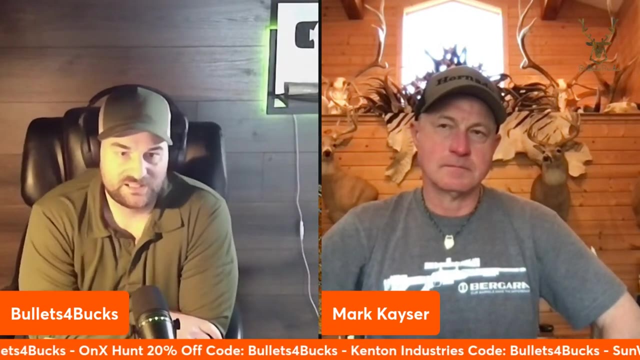 in us, So that's pretty interesting. So what are your thoughts, I guess, on the future of hunting and the next generation, things like that? Where are things headed? Are you concerned about that? Do you think we're going to be okay? What are your thoughts? 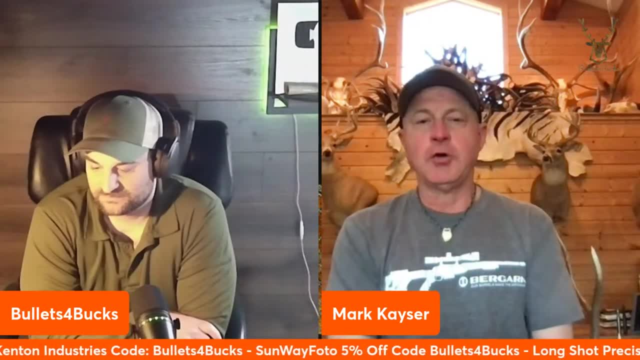 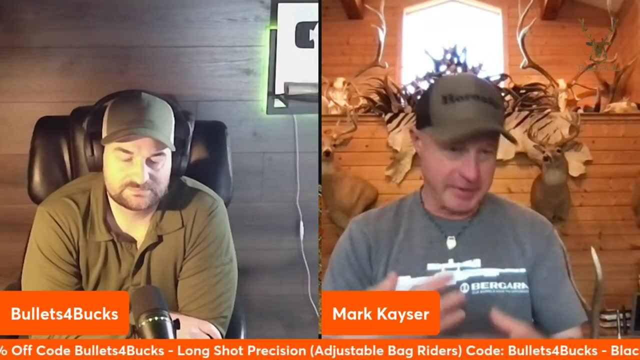 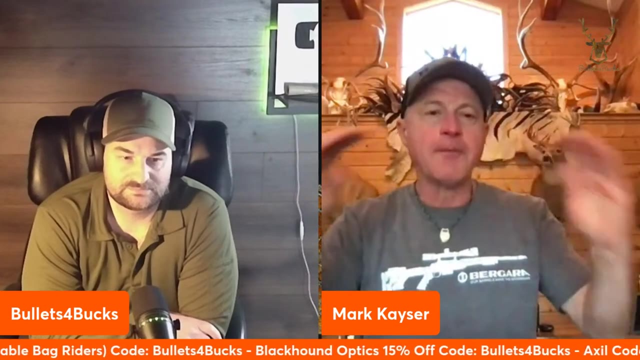 Well, I think, like you just said, everyone instinctively, it's hard to erase that evolutionary process in you to be a hunter or a gatherer. So I think if you would just take people out and they would open their mind up and you would show them hunting, it would turn them on. 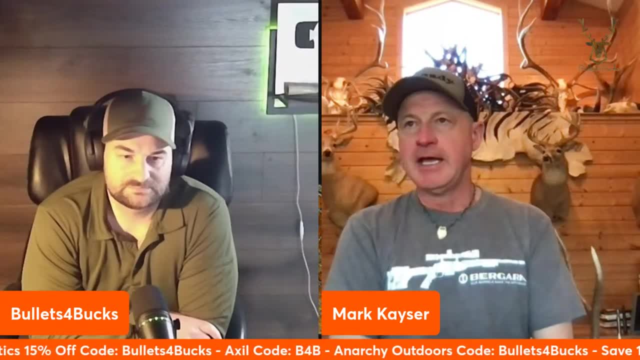 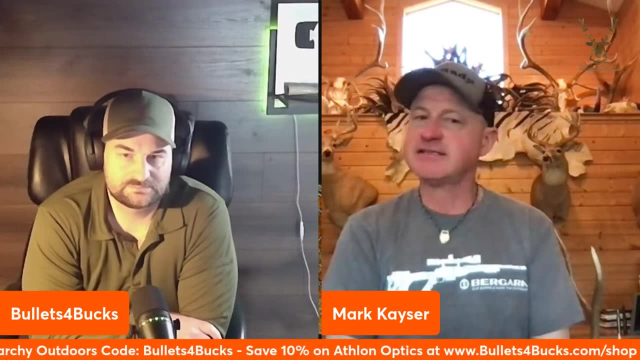 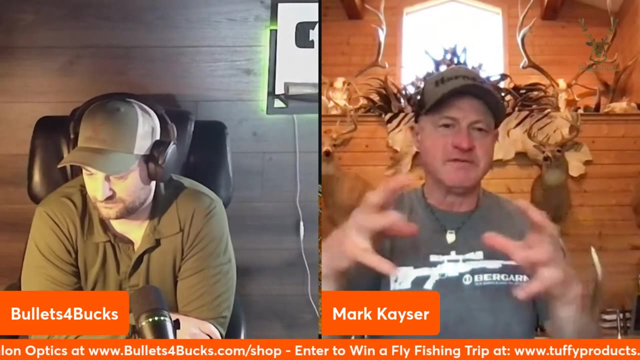 real quick. The problem I see in the future of hunting and that you may have had a little bit of issues with- I didn't as much growing up, but I think it's going to be a little bit more access. Access is changing dramatically and it's becoming a more closed environment. You just 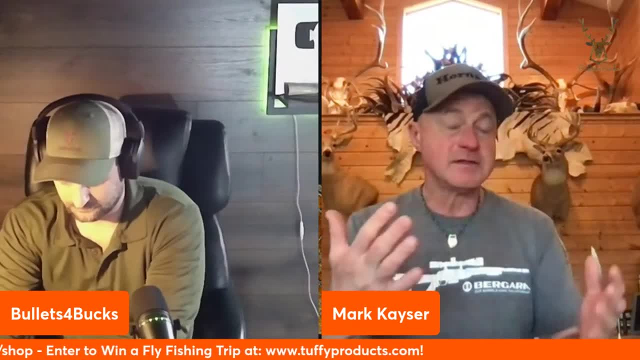 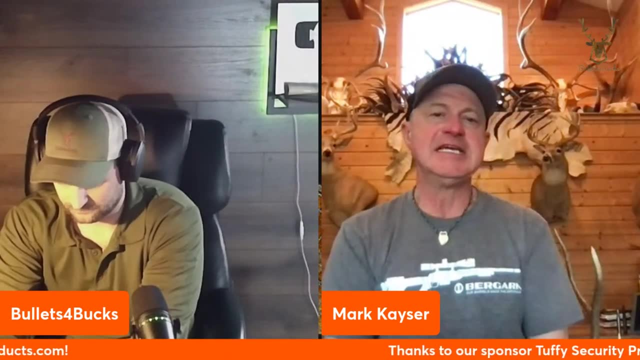 don't have access to private lands like you used to, unless you pay to play, You lease, purchase a hunt, do an outfitted hunt or something. But I think that's going to be the big key to keeping the hunting heritage open. We've got to have places for these young hunters, new hunters. 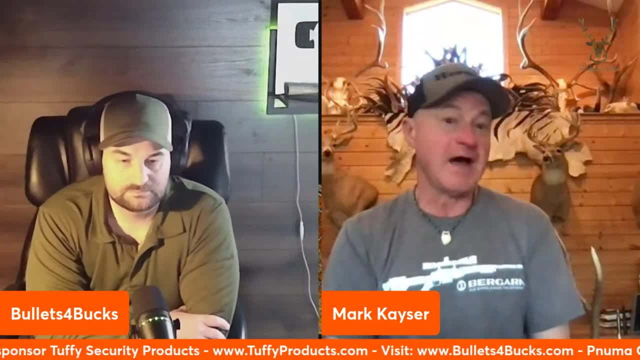 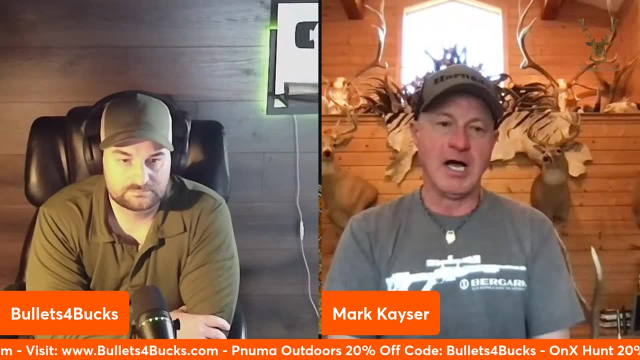 whether it's someone that's 35, years old, someone that's 12 years old, whether it's a young man, a young woman, whoever, We've got to have places that they can go hunt, And these places, which are going to primarily be, 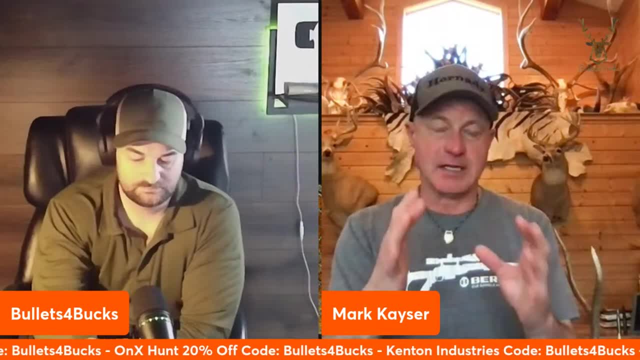 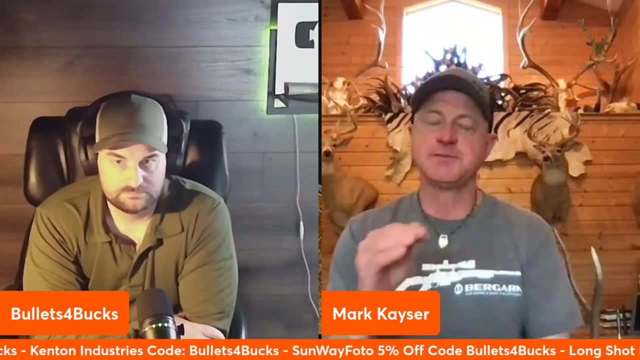 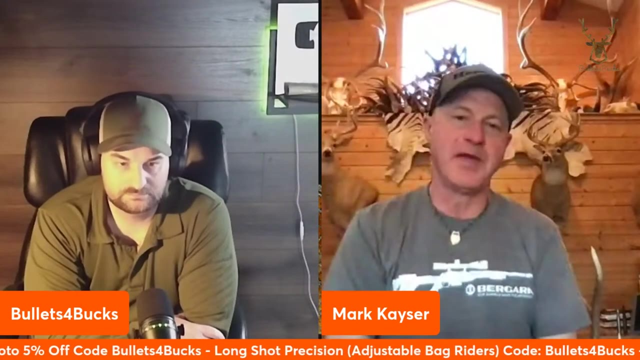 public lands and or leased lands. game and fish will lease lands that are private, open to the public. But these lands have to have some quality to them. They can't just be a bare pasture, a picked corn field, a big sagebrush basin. 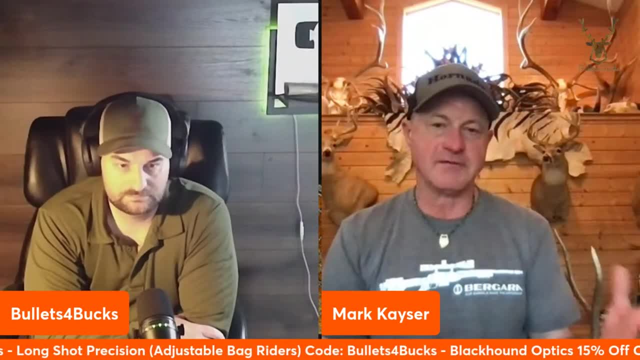 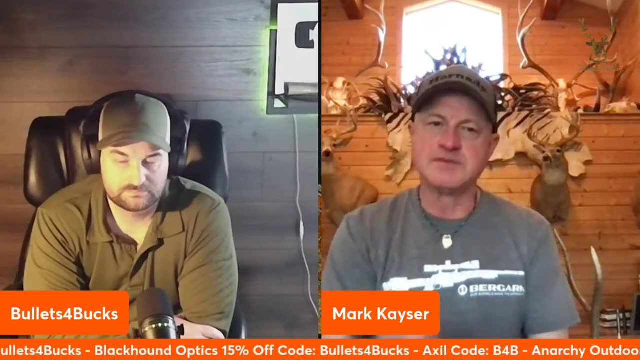 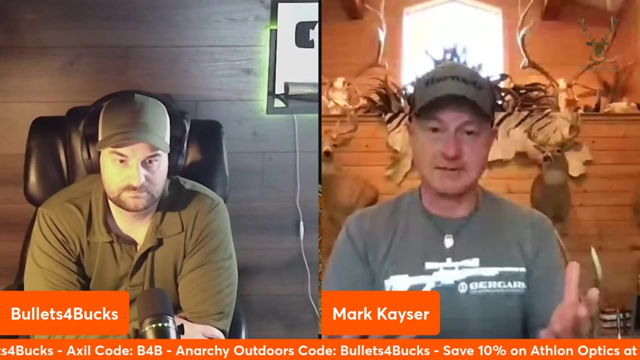 That's had 500 cows on it all summer and there's no grass left. They've got to have some quality to it, because if a person is going to ignite that spark in themselves, the only way to do that is eventually they've got to have a pursuit and they've got to find some success. So if you just 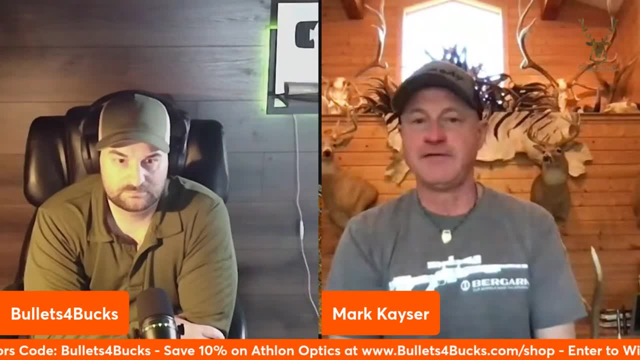 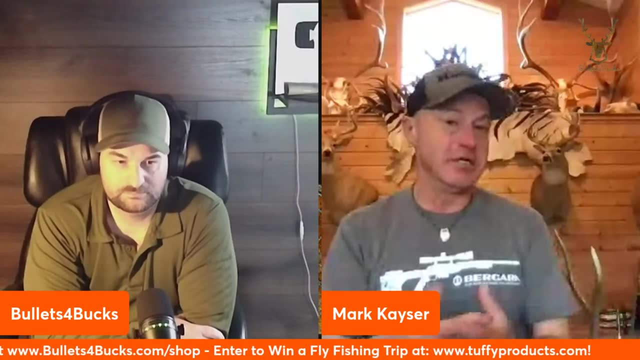 have run-of-the-mill land and there's no wildlife on it for anyone to hunt, whether it's pheasants, grouse, ducks, geese, deer, animal, elk. it's just like going for a hike And eventually they're just going to lose interest because they 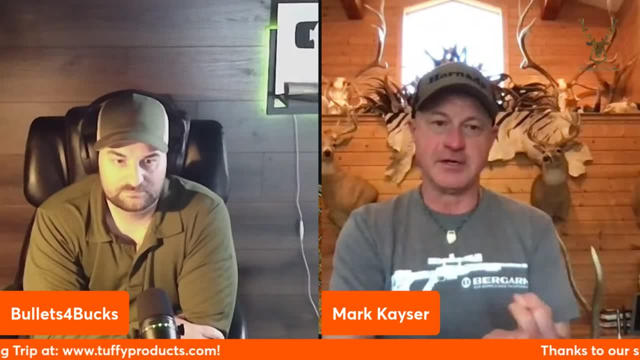 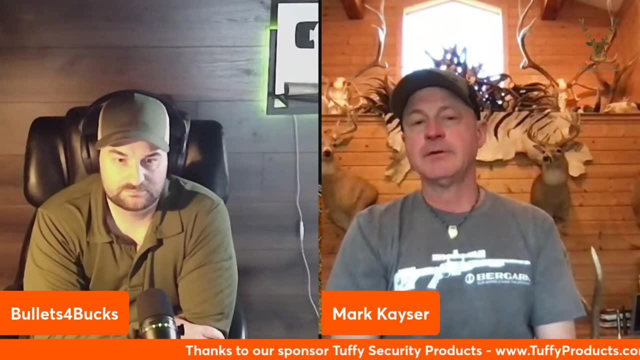 can do that without buying a hunting license, without buying a $700 rifle, without buying a $1,000 bow, without putting fuel in their truck and driving across the country. So I really do think that's the biggest thing, And I see it right here in my backyard in Wyoming. I see it when I go. 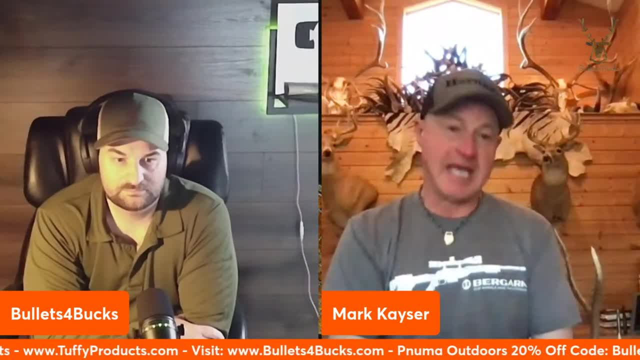 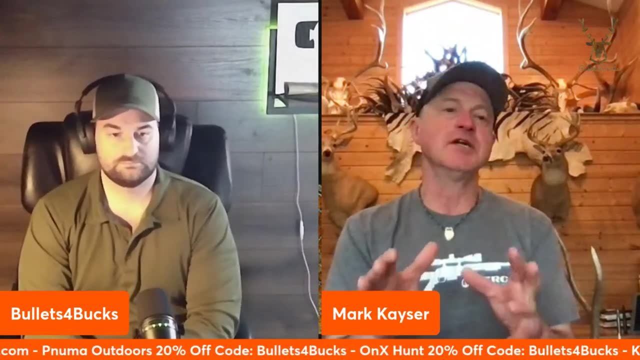 back to South Dakota and hunt. I really see it where I hunt in Kansas. That whole area in Kansas where we hunt has become not so much commercialized As much as just shut down and fewer and fewer people are allowed on areas to hunt. 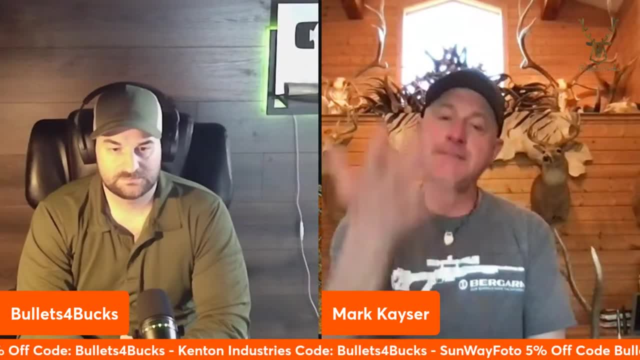 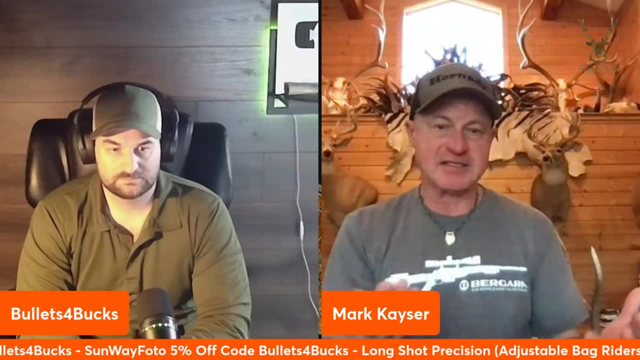 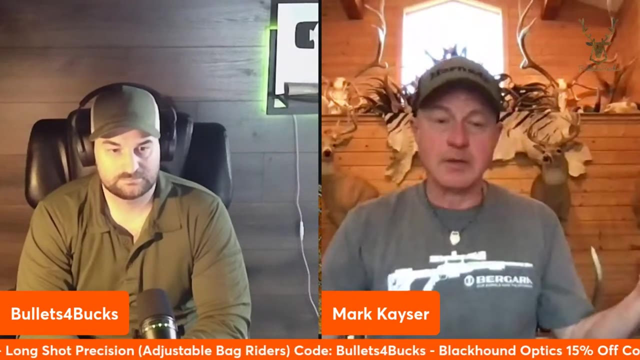 So we got to make sure that that access is there. And then mentor: I really think people help mentor. One of the ways I've done it in the past is I volunteered for 4-H shooting sports, getting kids involved in shooting. And then, of course, Mark is Mark, So I talk about hunting. 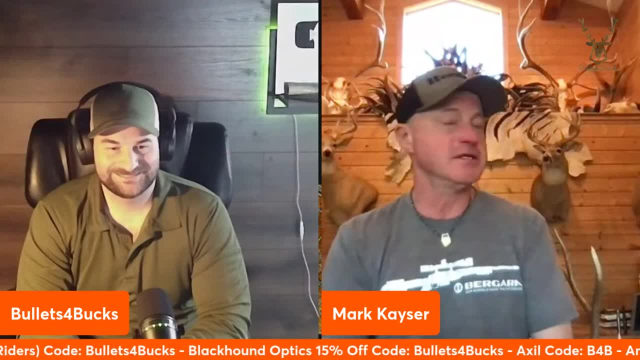 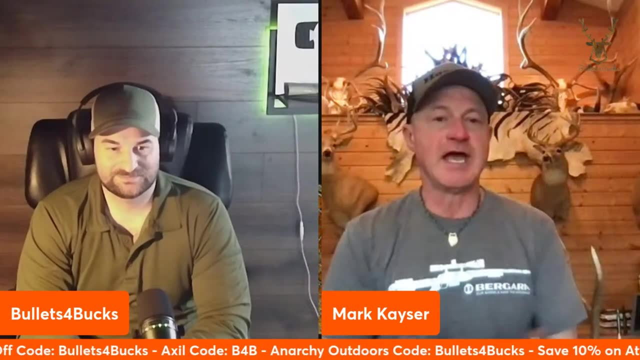 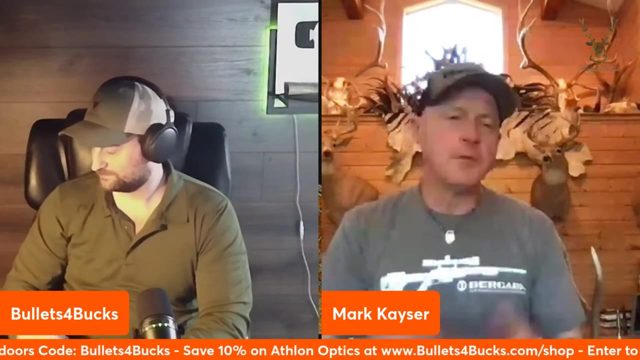 while we're doing that. So when my kids were growing up I volunteered all the time At 4-H shooting sports, even taking kids to the state match doing stuff like that, And the winners we would take them on a special trip to Colorado for another shooting event. So mentoring. 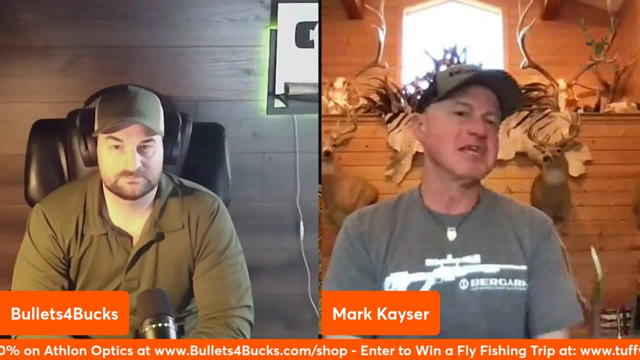 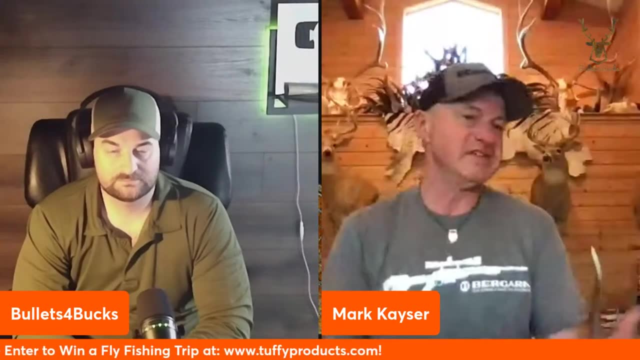 And a thing that I've done lately in mentoring is getting rid of some of my hunting equipment. You know, I've got a lot of hunting equipment that's 20 years old that I'm never going to use anymore. If I see a kid that wants it, hey, here's a couple of turkey decoys, Here's three or four. 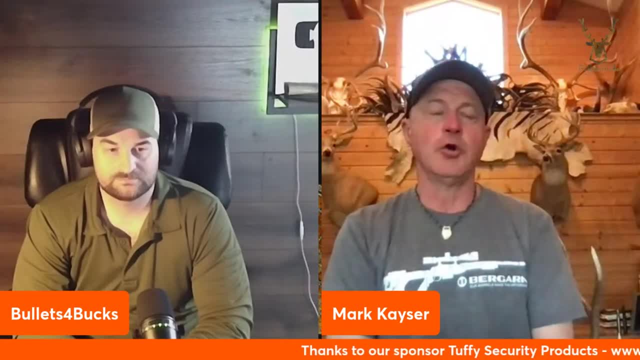 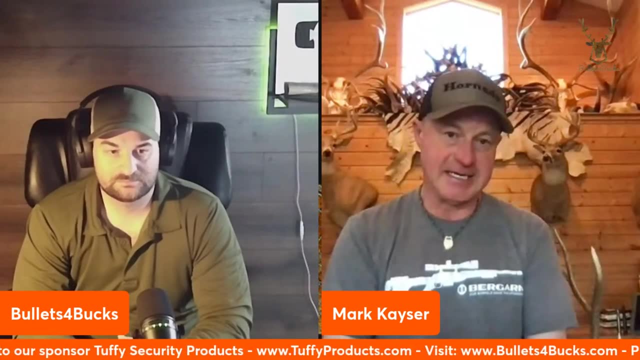 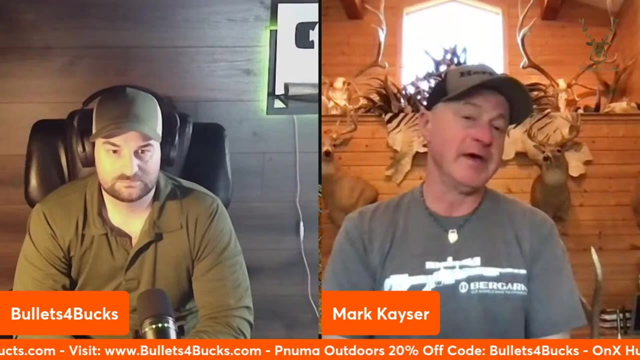 elk calls. Here's an old binocular I'm never going to use. Just simple ways you can get youth and new hunters excited And then hopefully we can keep some of these public lands not only building but managing for the best Right? Yeah, I've started to do some of that. I've been blessed just the last couple of years And so 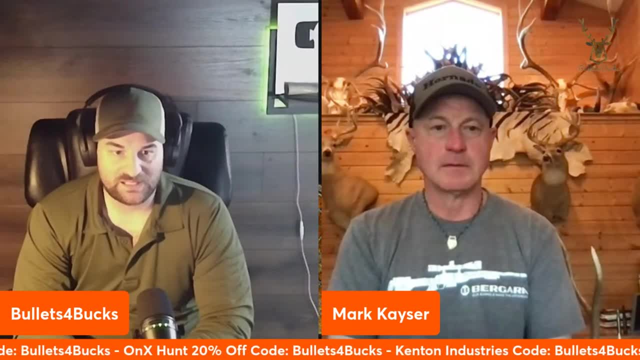 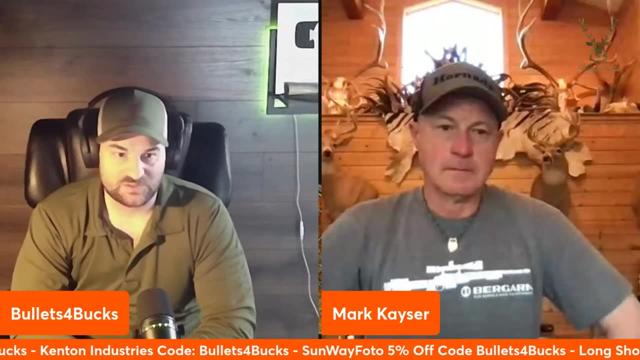 I've outfitted a couple of people essentially with just like. I guess once I've upgraded gear I've just outfitted other people with my older gear. That's still very good, Just, you know, not the newest thing I bought, But that's interesting I do. 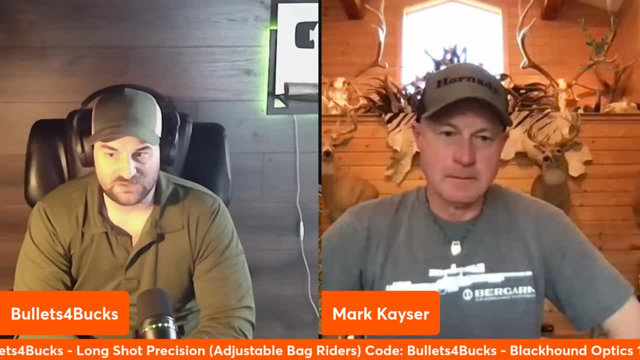 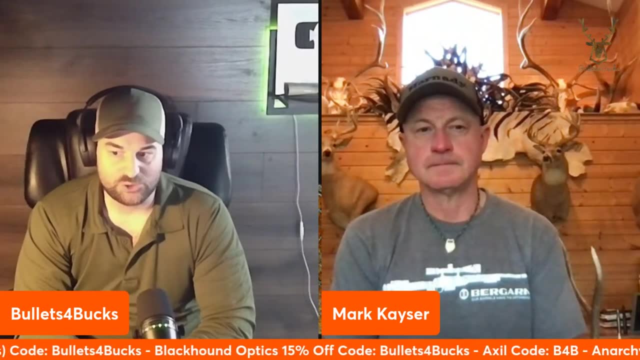 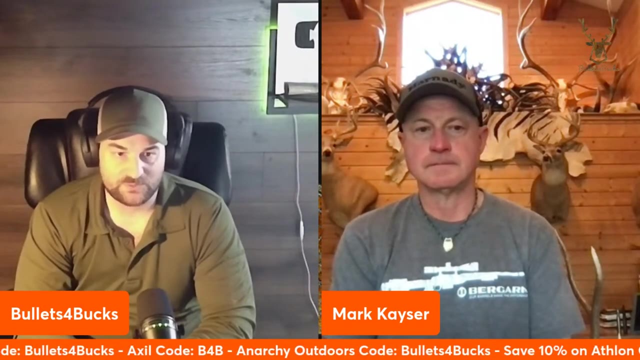 think there's definitely issues with land access and like land that's being acquired or open to the public maybe being not really good lands and people taking or ranchers or different farmers taking that to their advantage, maybe in land swaps or whatnot. I think. 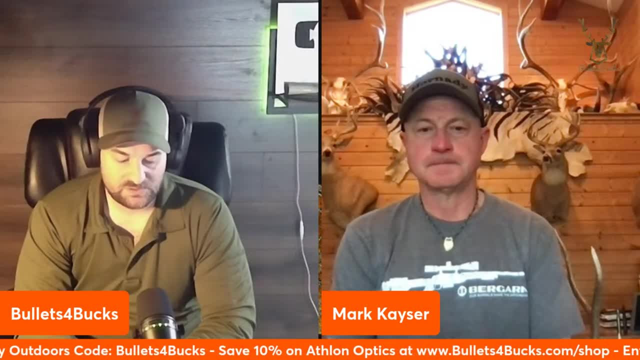 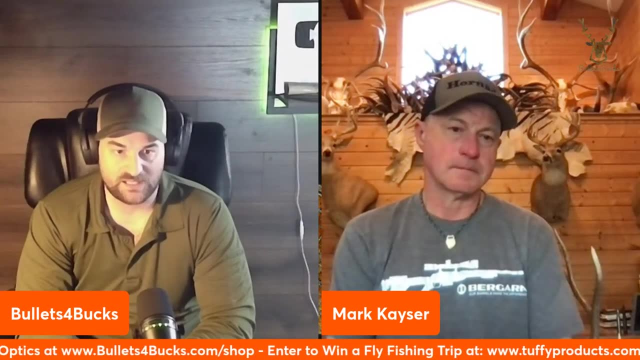 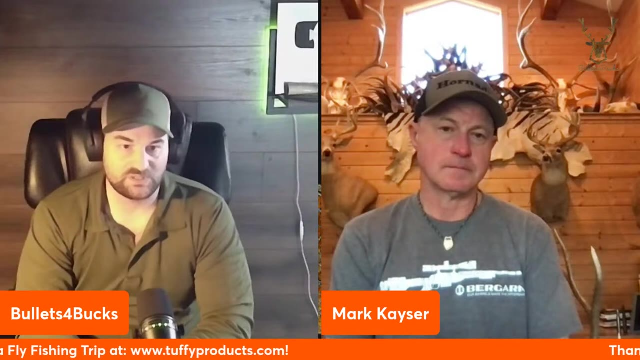 I think that one of the biggest hurdles new hunters have in- even more so in states outside of Wyoming- is public land access. Like the eastern side of the country, it's like they almost feel like they have to own land or lease land, And so that's a really big financial barrier for them. 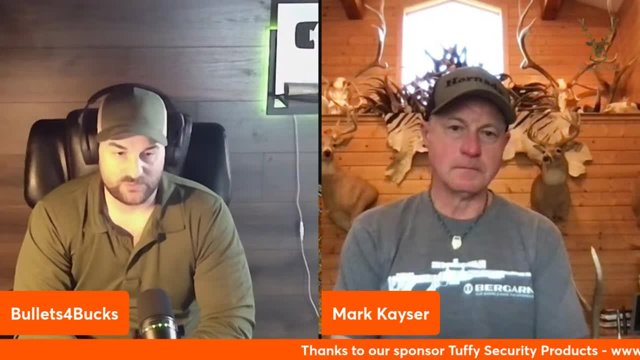 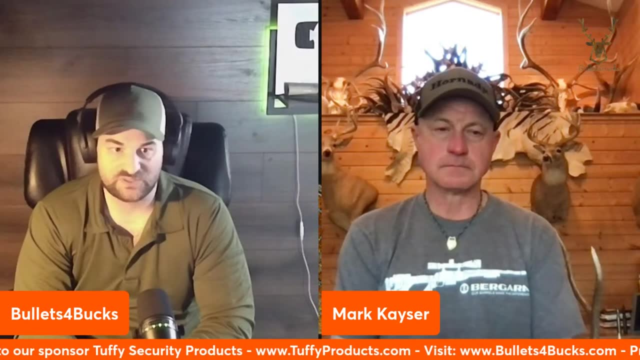 And I do think also, if the land isn't is fruitful, then yeah, I mean, most people aren't going to go out more than 10 times, probably more than three times a year, And so I think that's what now they think is very important: Just the fact that the lands are built on land. 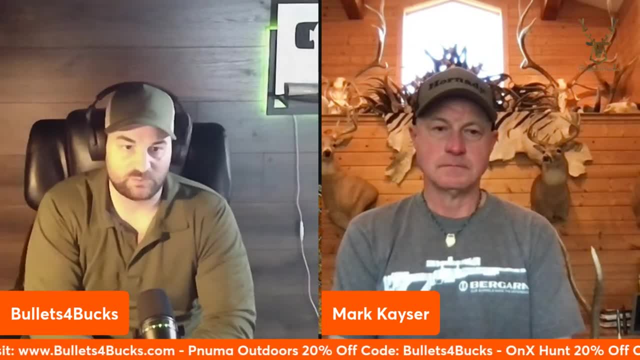 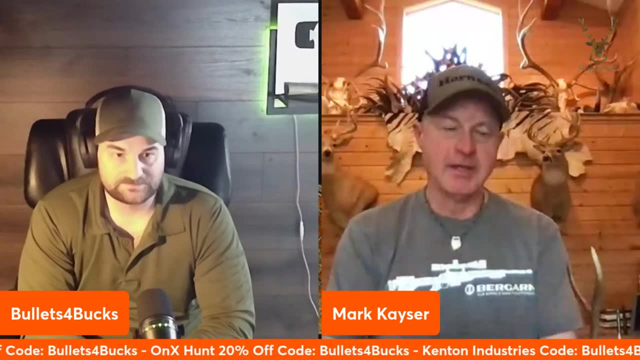 It's not just in the highlands, but it's also being ushered in more than 10 times as a home, or maybe not even three times as a young adult. if they don't get something, Or at least maybe you have an encounter- maybe they don't have to have success, but maybe they need to have. 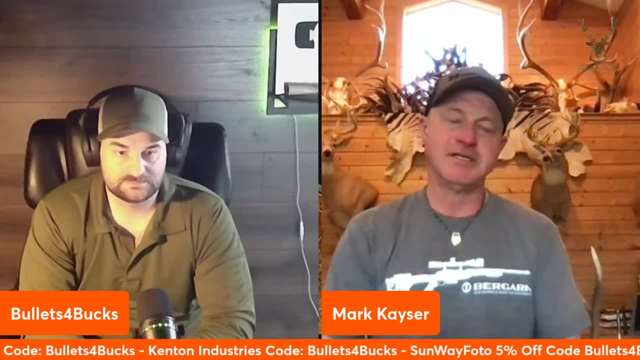 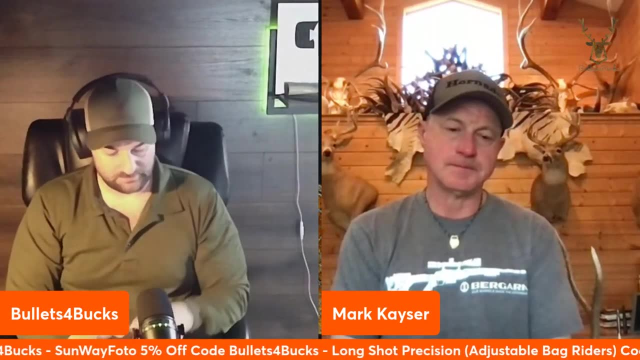 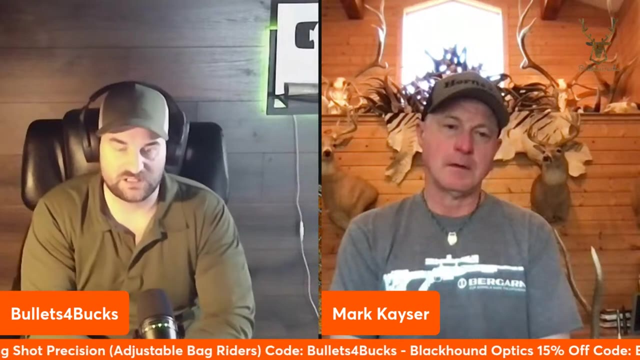 encounters with, with whatever game animal they're targeting. In the case of adrenaline rush, they got to have that right. If it's just again a walk in the park carrying a rifle shotgun Hunt Foundation, I think that's one of them that helps young adults and teenagers get into hunting. 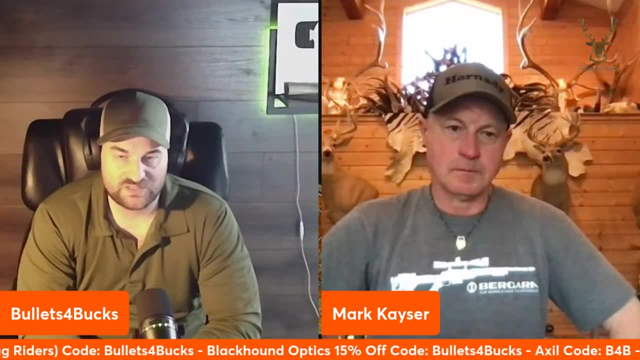 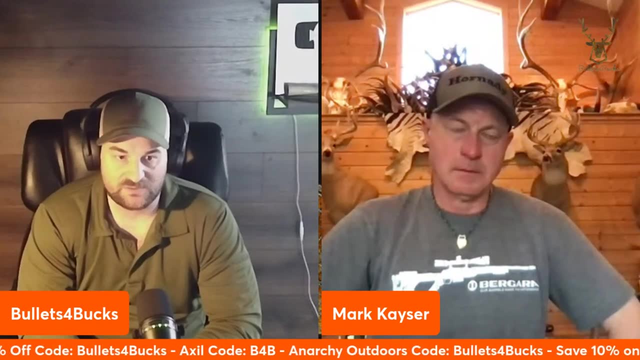 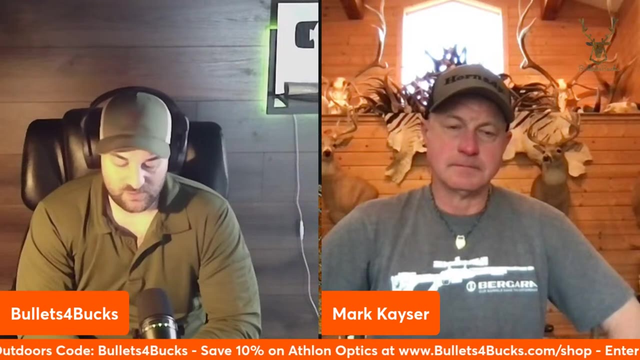 and offers basically locals to take people on hunting. I want to say it's First Hunt Foundation And then there's a whole bunch of first responder organizations essentially that offer, you know, first responders, military, police, blah, blah, blah opportunities. But what are your thoughts? 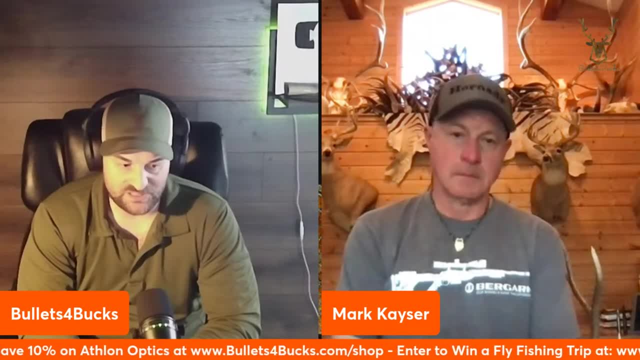 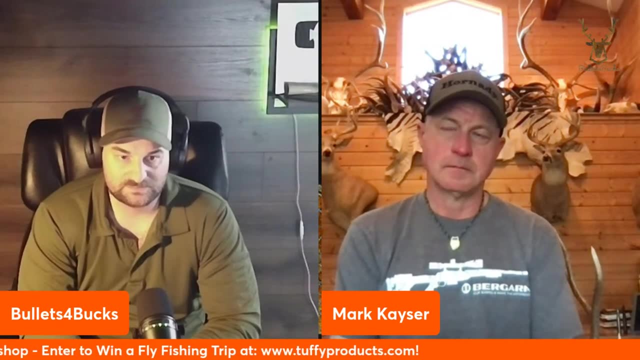 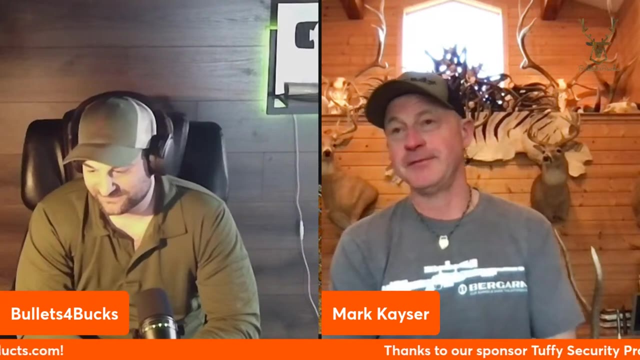 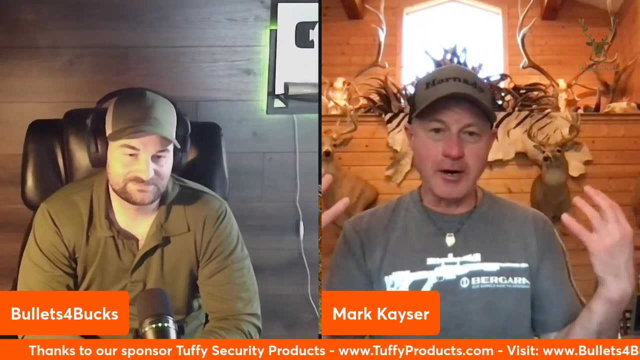 also on I mean like CWD and the health of mule deer in the Western United States or areas like Wyoming. I do have a huge concern about mule deer in Wyoming And people have maybe seen that on some of my social media now and then, You know, in my backyard if I look out that window, right? 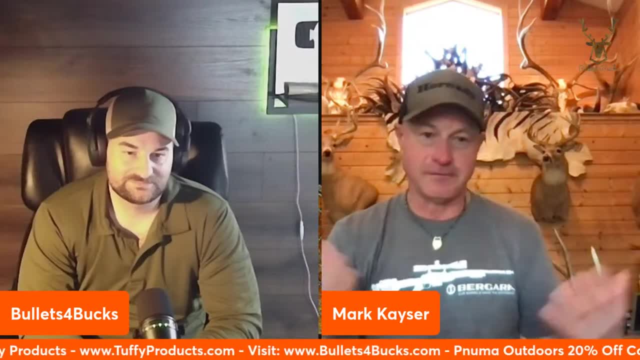 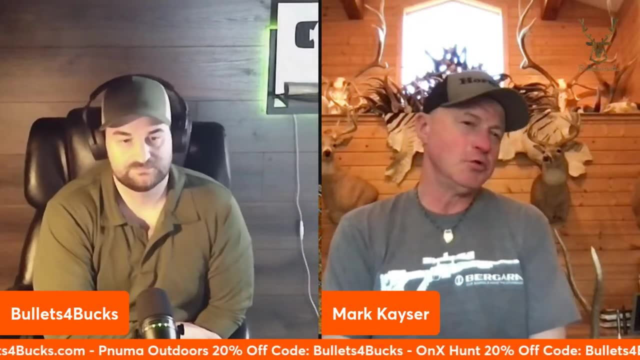 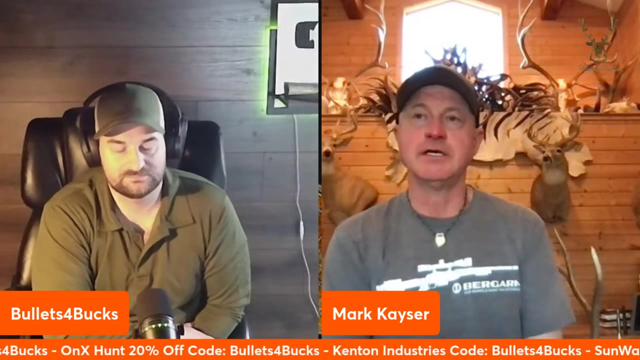 up there I bet you can probably count 20 or 30 deer right now just out feeding. It seems like in the private land fringes, mule deer seem to be doing okay. You see plenty of them. But I spent a lot of time in the back country in the mountains, And I have been just recently. 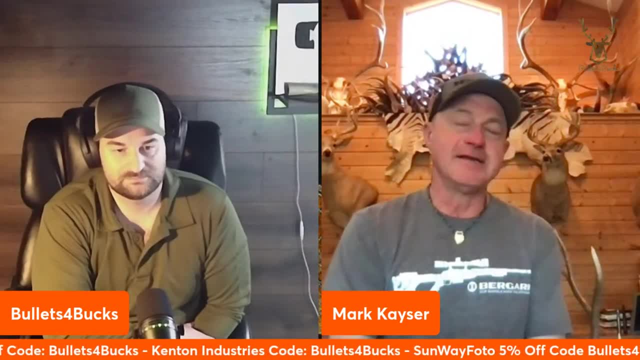 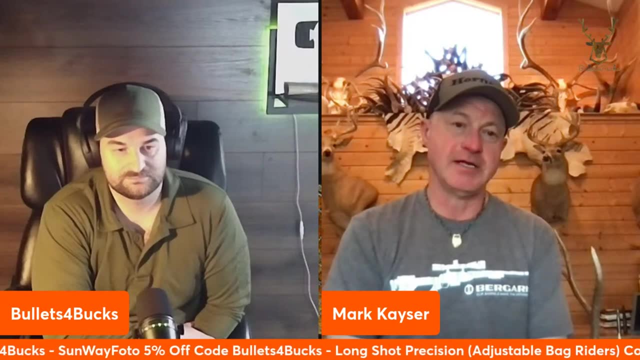 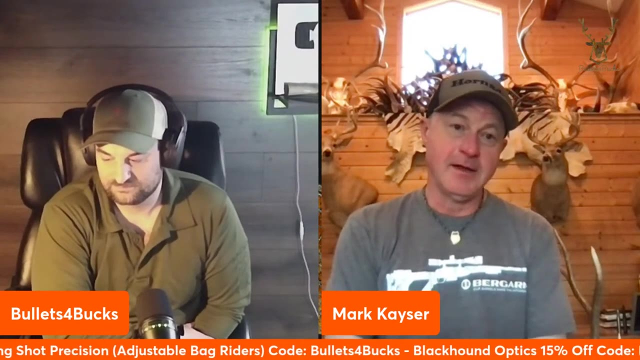 shed antler hunting. To date, I have only found two or three fresh mule deer sheds, And I have not found one on the mountain, And I've found several backpack loads of elk sheds Already. it just there's just no mule deer up there to speak of. It's just a shame, And I don't. 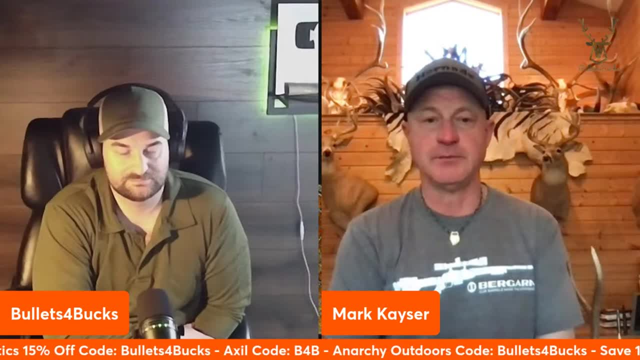 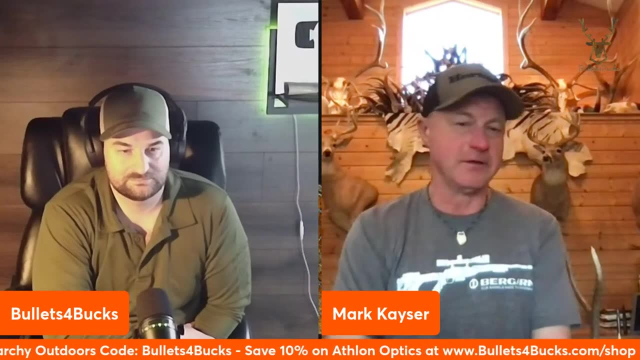 know why. I mean, I do know some of the reasons why. I've studied the mule deer working group, read a lot of their research and stuff. There's a whole combination of factors that just come together for the perfect storm on mule deer. But I really I am worried about mule deer in the future. I see it in Montana where I hunt Wyoming. i hunt some in south dakota, but mule deer just don't seem to be doing very well on the public lands, especially as compared to, uh, elk, elk, elk, man. they're just exploding everywhere, it seems. 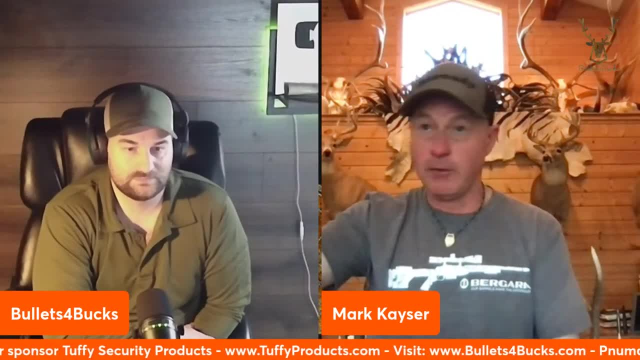 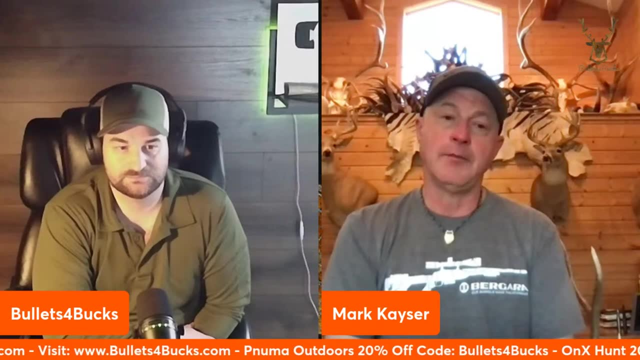 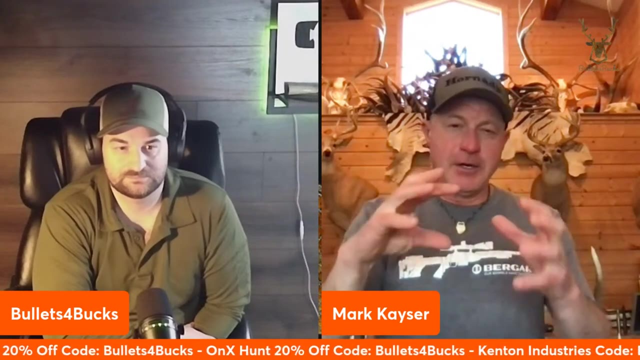 yeah, you see elk. i once in a while we see elk right out my window, right here. you know where i live, a few miles out of town and uh, shared in wyoming. so uh, but mule deer, they're very niche species, like pronghorn, they, they, they rely on a very precise environment and if anything changes. 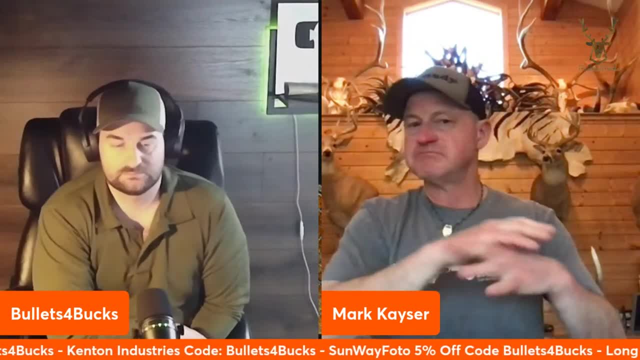 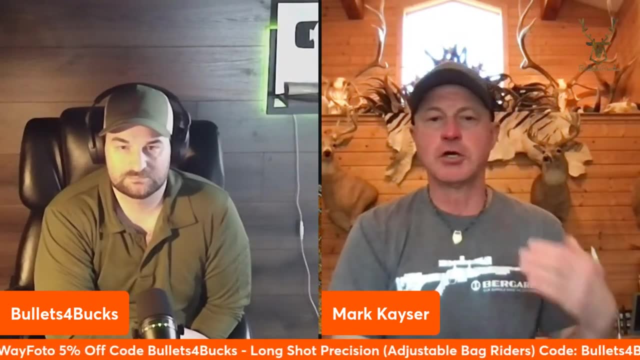 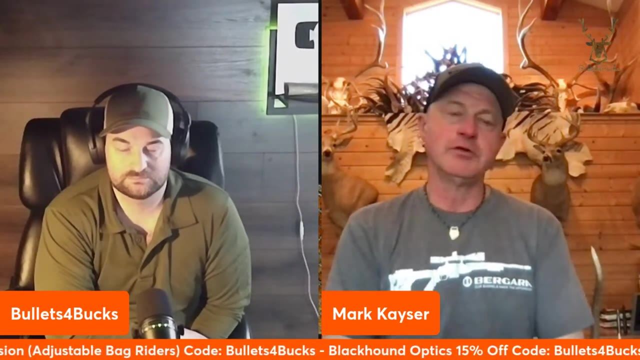 in that environment. it really affects them. elk, they, they lived all across north america, all the way into mexico, all the way, you know, almost the arctic circle, uh, pacific to the atlantic. they were able to adapt. white tails very adaptable as well, mule, deer, pronghorn- not so much they. 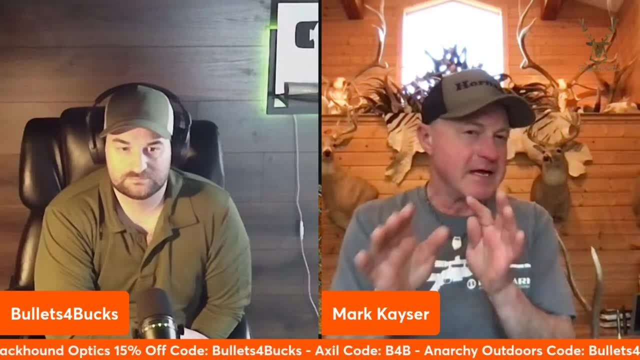 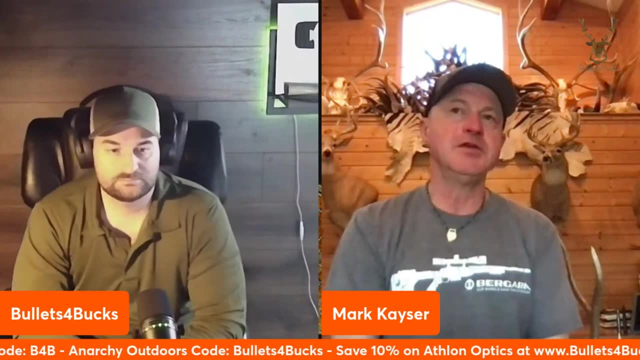 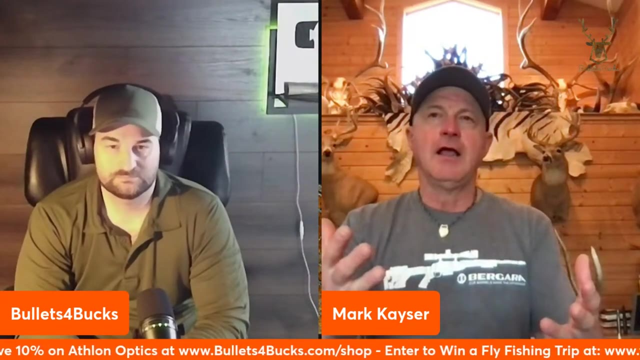 they really have a targeted little world that if anything changes it can really dramatically affect their outcome in life. and as far as cwd is concerned, i've just never really gotten on that bandwagon. i i just as a whitetail enthusiast early on and now i spend a lot of time in 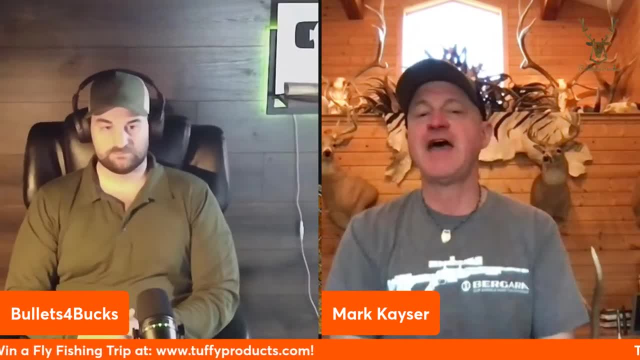 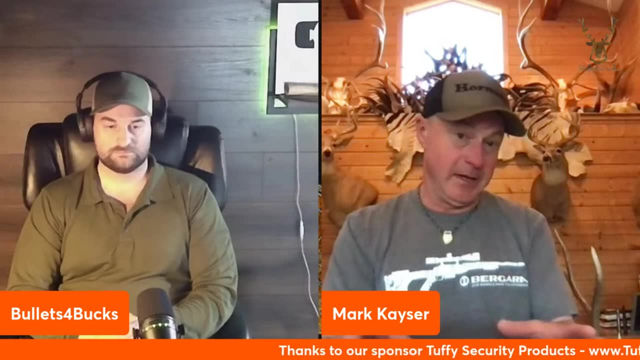 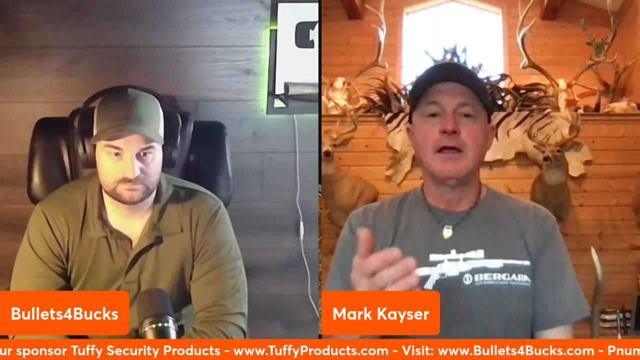 whitetail woods too, and i truly see the effects of epizootic hemorrhagic disease, that that when that disease comes in, you see it, you smell it, see it. uh, i've stumbled across a lot of deer, you know, dying of it. i just really don't see a lot of deer deaths, mule deer because of cwd or elk. 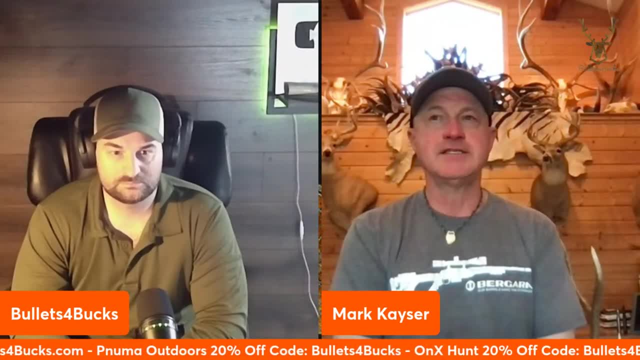 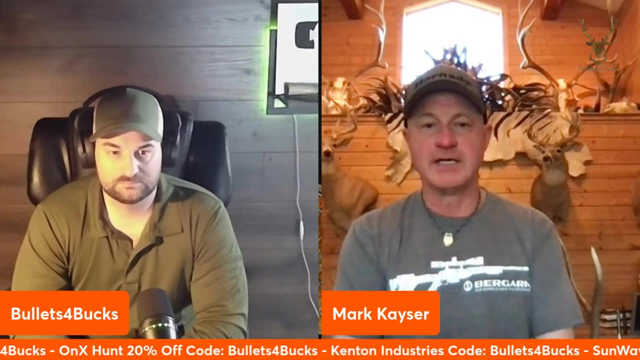 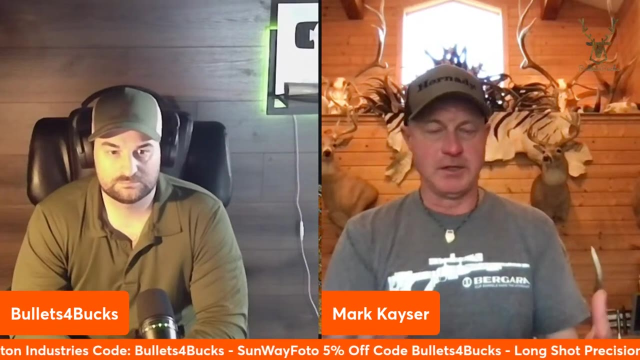 you know they say it's an elk too. but um, i just, i, i know, i know it's there, i know it's real, i know the biologists, researchers, you know they, they feel it's a threat. but when i've been just immersed in epizootic hemorrhagic, you know, over the years and seeing ranches, just 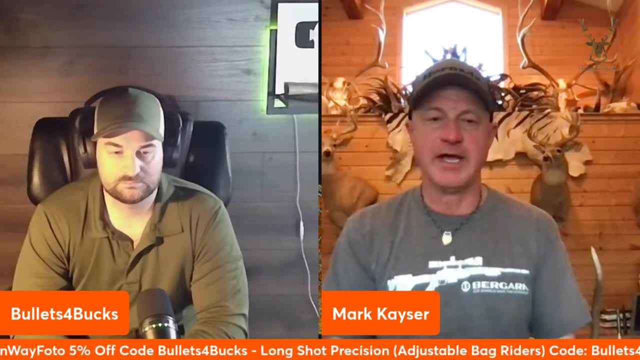 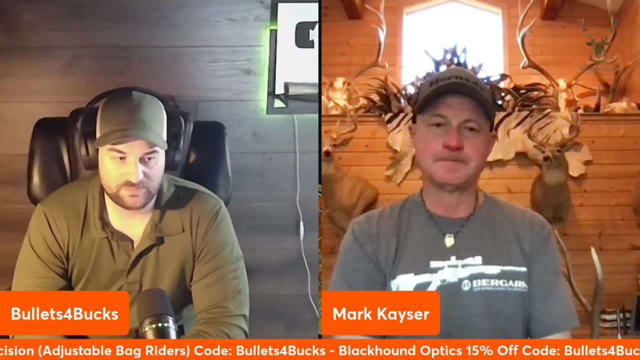 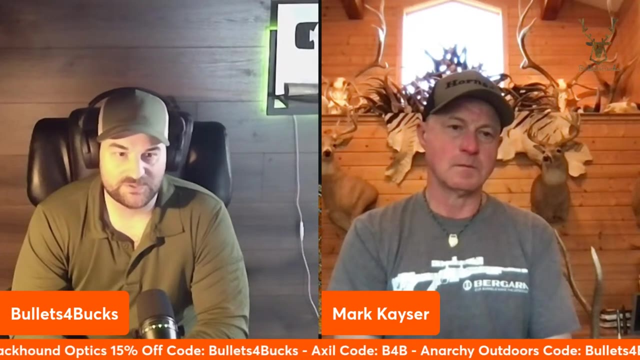 fall apart and farms, just you know, get wiped out overnight. i just don't see that with cwd, do you? i mean, what's what's your? no, i, i, i. i don't know that much about either one, um, but i kind of take the stance you do i. i don't buy into it a hundred percent. i kind of think maybe it's been there. 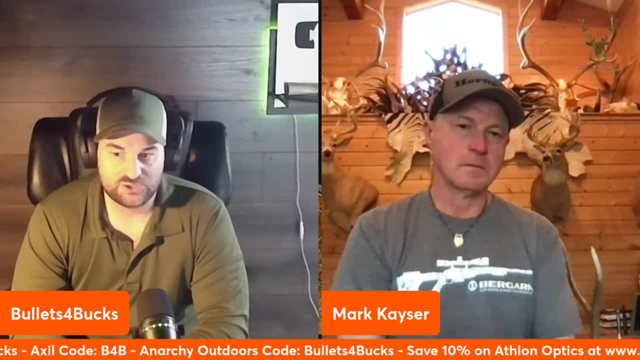 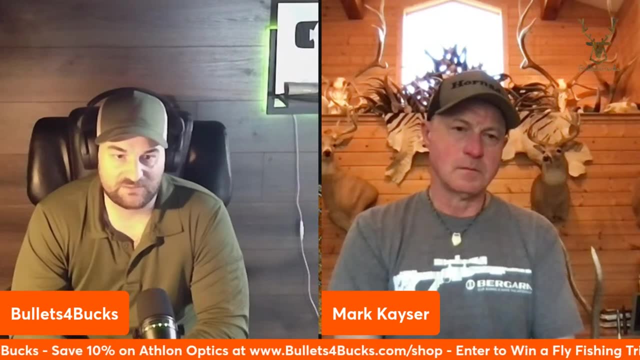 longer than even they have known, and i don't see it as a huge threat, that's. that said, i don't believe necessarily should be ignored. um, i just haven't. it hasn't seemed to have a have a large effect on my hunting at this point and i don't know that. 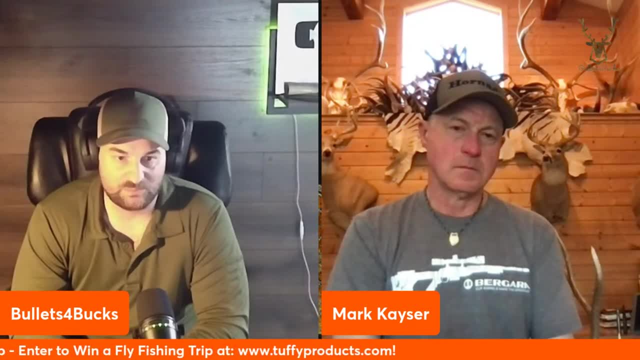 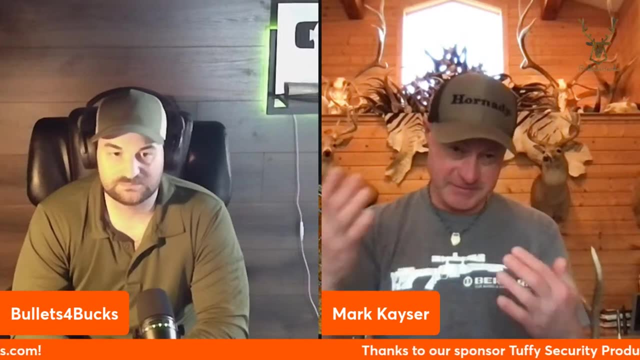 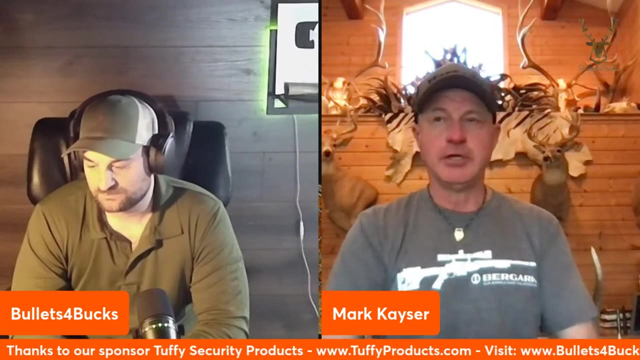 it's as big a deal as some people think, but i'm sure that's a non-popular stance with many. i just you know. i believe there's bigger threats out there, personally for mule deer. but again, i i'm with you. you know it should be monitored. you know, i don't know if it should be. you know one of these. 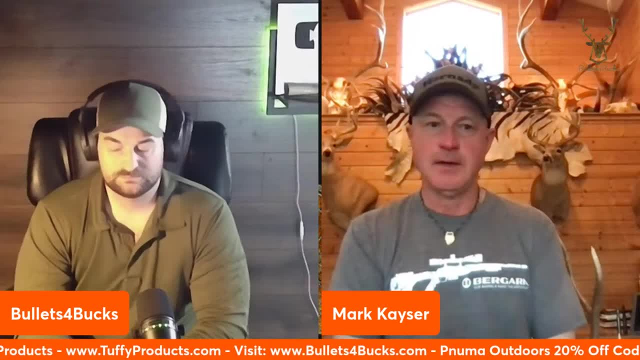 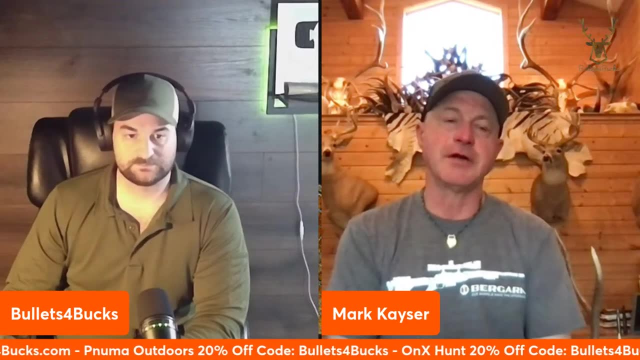 things like wisconsin, saskatchewan, you know they would, these big kill offs and stuff. i just i don't see that as the answer necessarily. but uh, definitely monitor it and i'm not so sure too. like you said, i always kind of thought that in the back of my head, you know, i think could have. 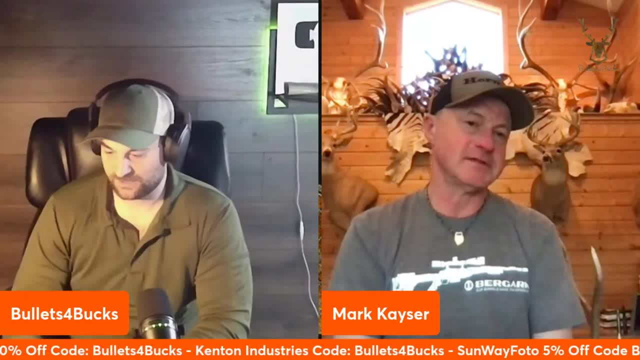 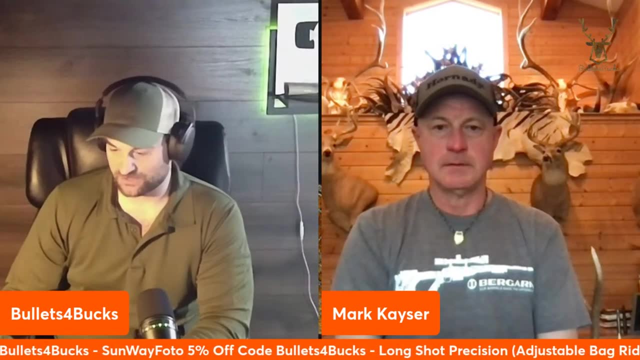 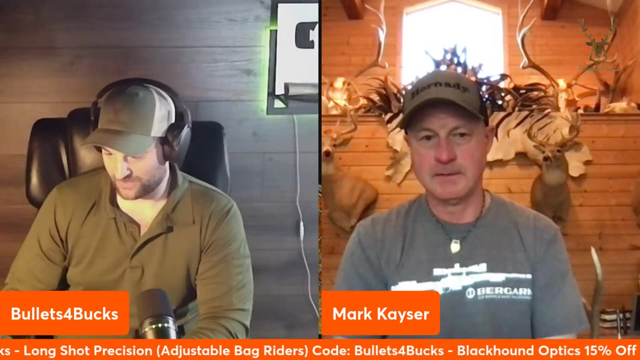 been here since caveman. right right, i see we got some people watching. um, just a reminder to the folks watching, we will get to your questions. make sure and go ahead and ask those, we'll get to them. so we got buckwells devin. uh, steve from wyoming, he's got a fishing youtube channel. that's really. 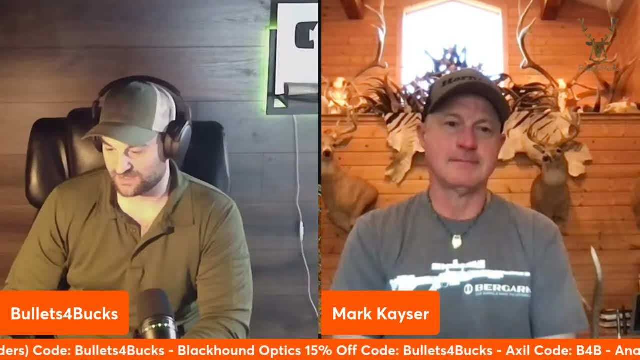 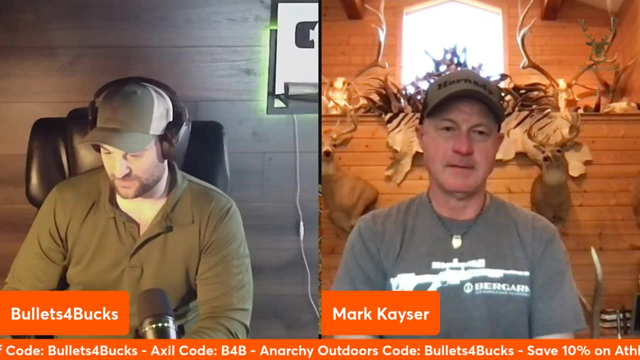 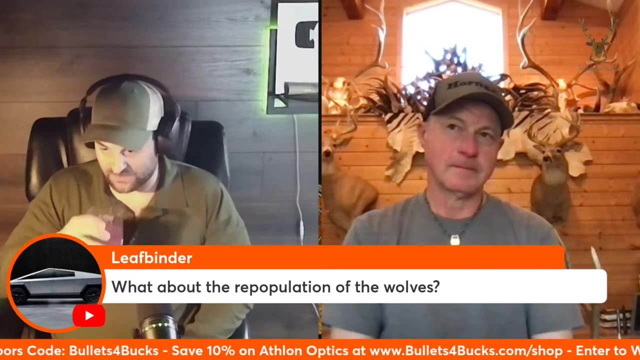 really well. there's fishing guns and hunting, but really good fishing content. um, leaf binder, good to see you here, you're a regular. um, i did see one question. this is a good question for us to answer right now. what about the repopulation of wolves? i wonder, uh, what your opinions are on those on that. 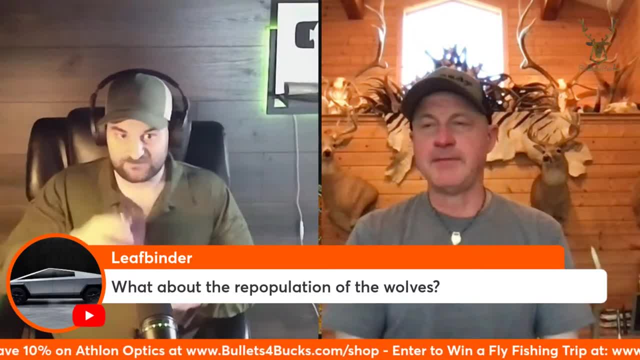 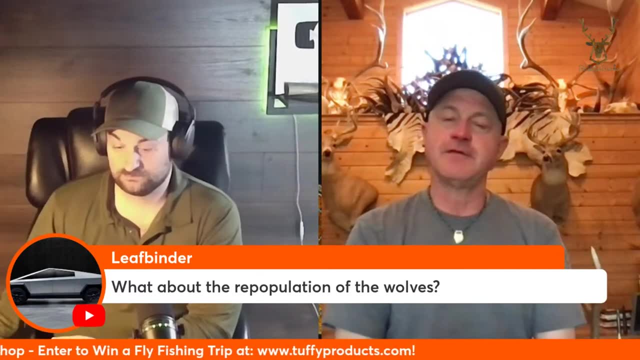 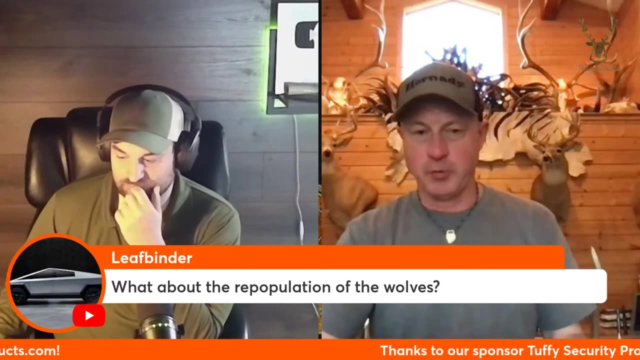 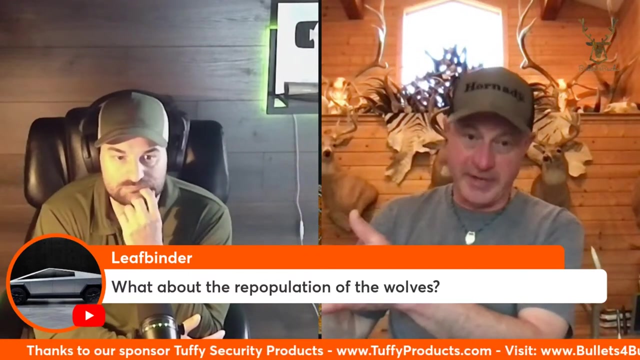 subject there. i you know i'm not a wolf expert, i do. i read research all the time. i believe the wolves are going to repopulate themselves. they have all, just like colorado, you know. now it's just you know- dumping wolves into their state and and they've got the biggest elk population in the country. and we know what happened in wyoming. 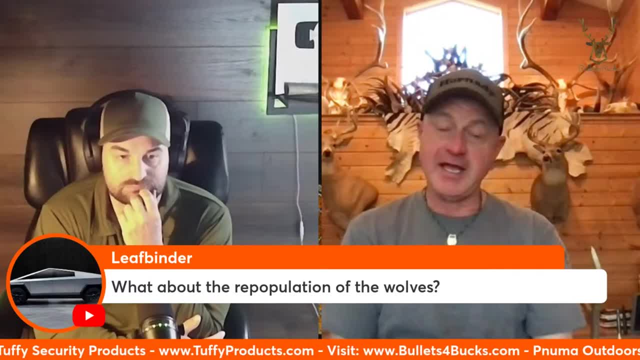 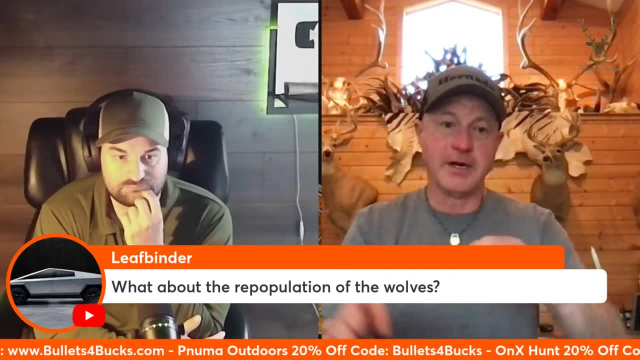 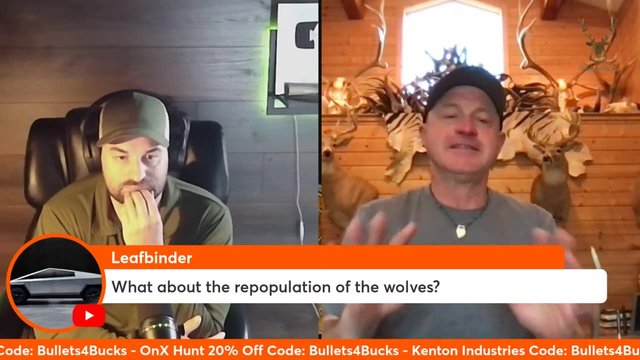 in northwest wyoming. we dumped wolves there, you know they. they ate them out of house and home. there they the elk. there's no doubt about that. but there was a spike in a plateau there. you know, once they ate a bunch of elk, then the wolf packs started going down as well. i just think at this point. 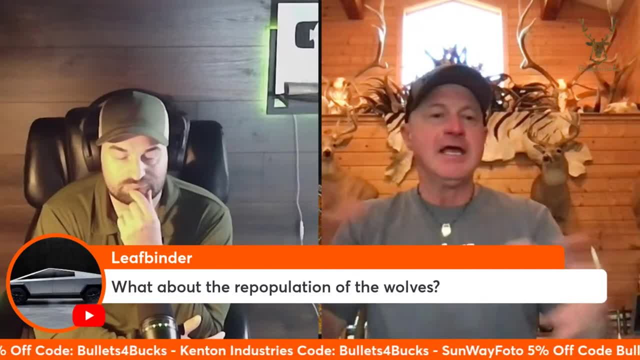 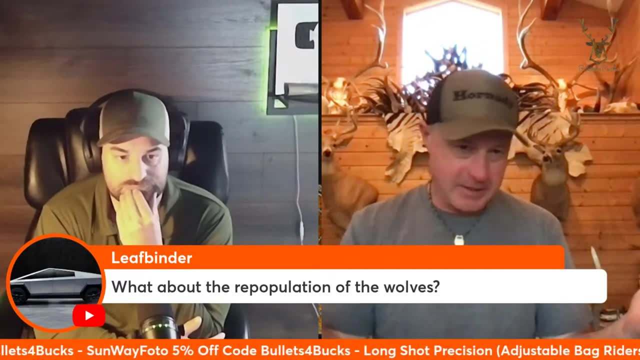 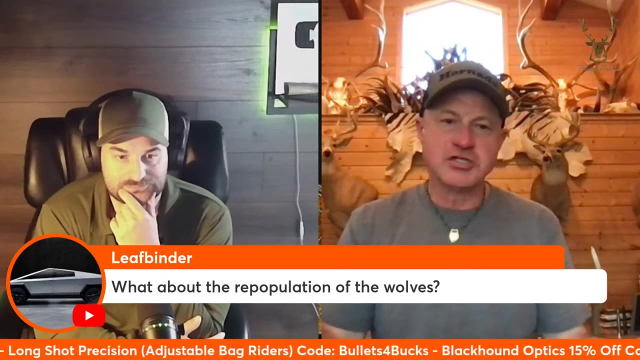 you just let these animals repopulate, just like they're gonna do it, let them spread and then manage them, but of course everything becomes political. you know, it's just like we're bears. we could be hunting grizz. they kill. i think the number is 20 to 25, 26, 27 bears a year in wyoming. 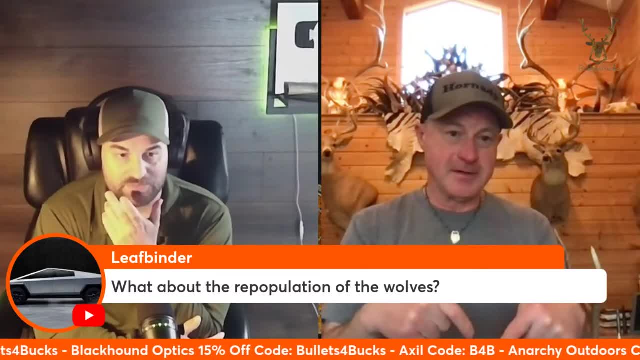 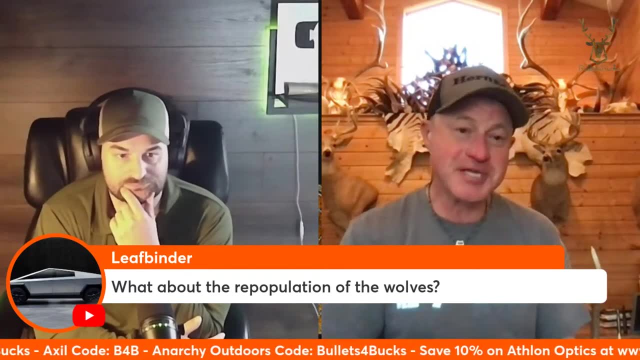 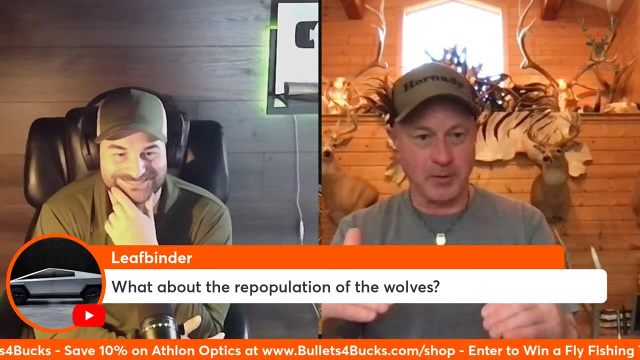 my goodness, you're talking about grizzly bears. yeah, problem grizzly bears. they're killing a dozen or more. let's just say that a year. someone's getting paid to shoot them. why, why are we not managing them better, so those bears won't come down and get in trouble in the cities or going into ranches? 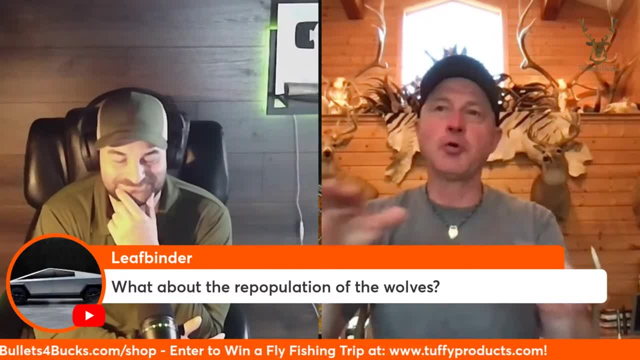 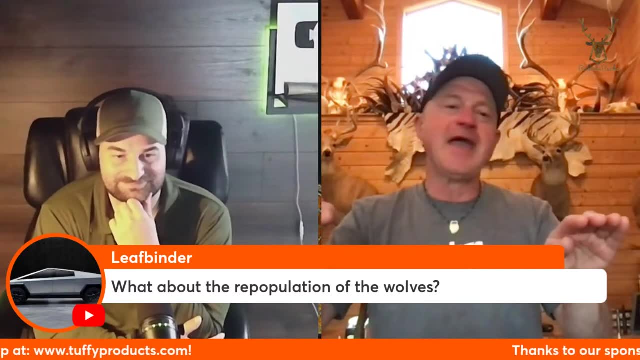 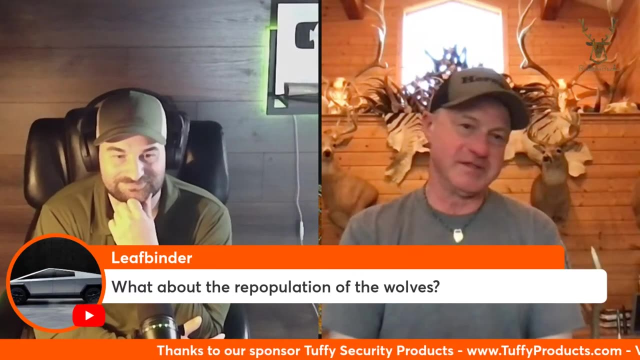 and such. if you just do a little bit of management and then they're worried about the genetics not being able to meet, from the northern grizzly bears to the to the yellowstone bears, and it'll happen. grizzly bears wander, it's just like the big horns here, right out my backyard. there's going to be a. 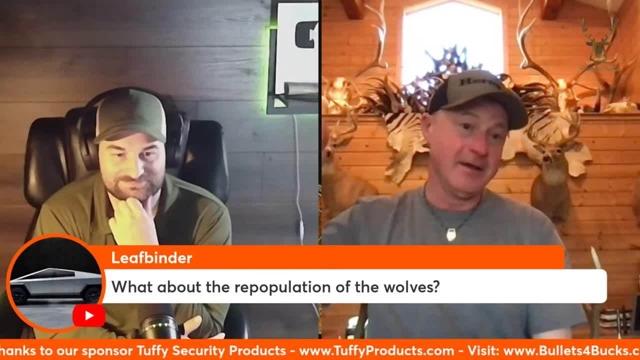 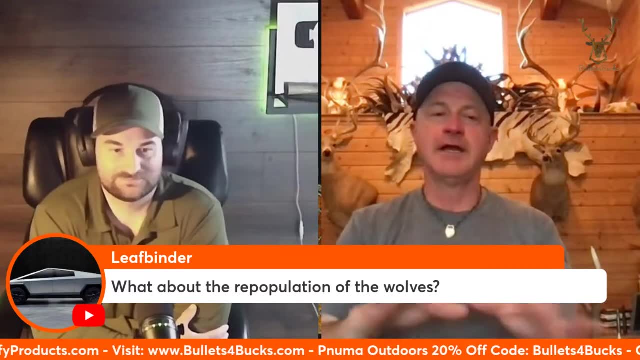 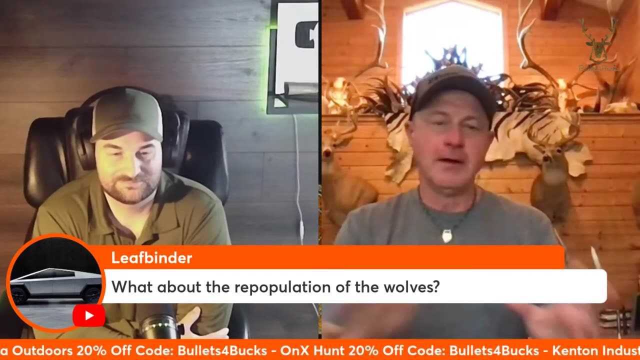 grizzly bear. show up there soon. there's one in montana, not that far away. you know it was recorded here. what was it? last summer or within months ago? so i think it's wolves. let them do their thing, let's manage them and let's all live together. i i've got no, uh no animosity towards. 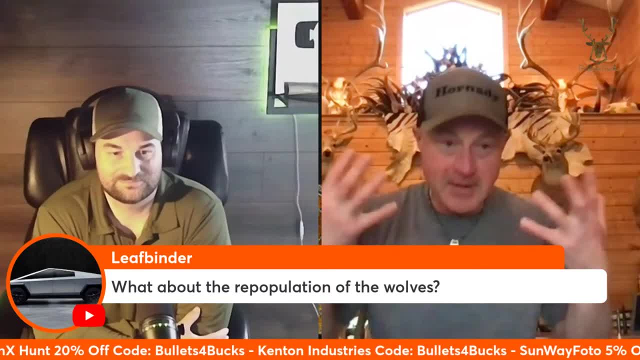 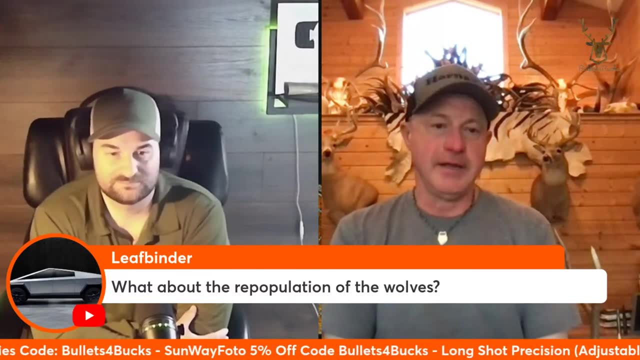 bears, wolves, whatever. i think it's great. you know that's what kind of makes you alive when you're out there, knowing that i- i, several years ago in the big horns i came across a wolf kill, that it killed an elk and it was uh, it was kind of just neat looking at those tracks. 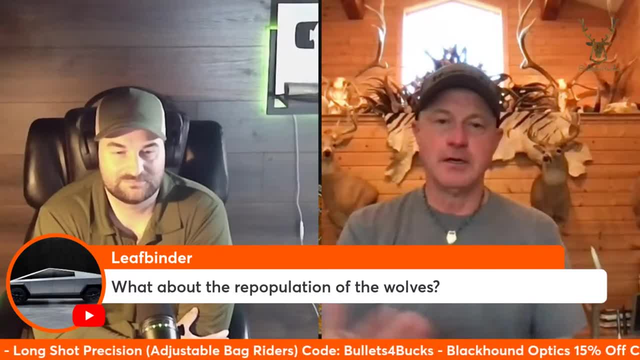 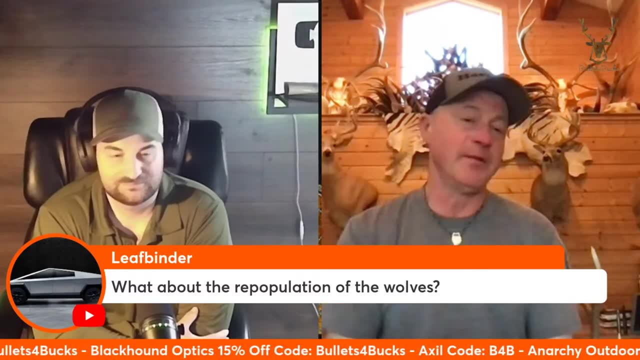 following the story up to where they'd killed a yearling- or it was the calf of the year, uh, elk and uh and same thing with mountain lions. almost every time i'm up in the mountain, uh, mountains. now this spring i cut across the mountain lion track because they're following the elk and deer herds. 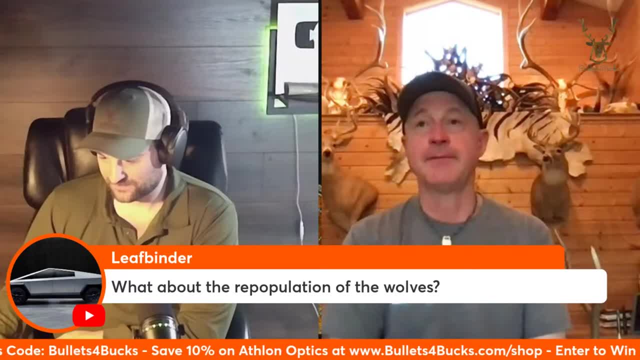 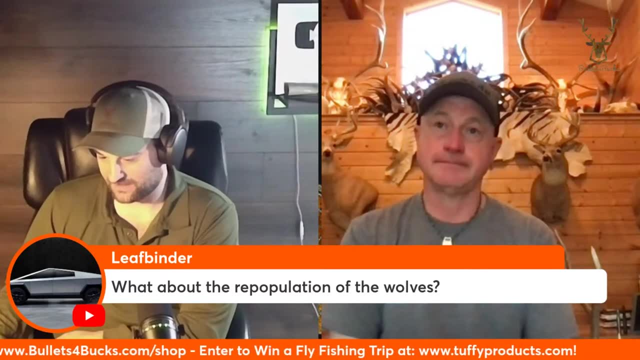 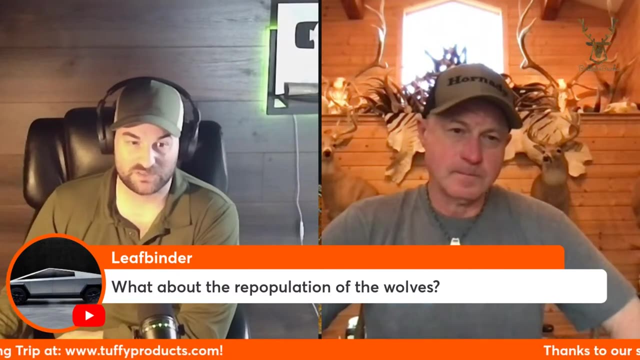 yeah, yeah, there's a lot of them up here. yeah, we got a lot of mountain lions. i run into tracks all the time. a lot of black bear too- at least that's my opinion, but i, i, uh, yeah, black bear is right around the corner. at the end of this month is, uh beginning of legal baiting, i believe, where you can. 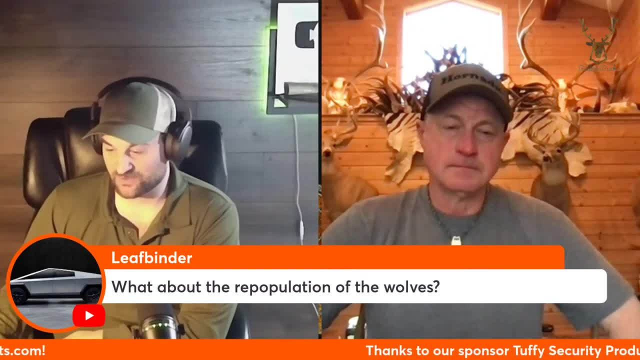 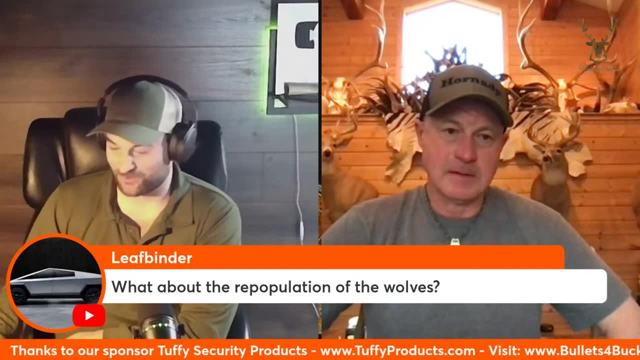 set your bait out if you bait hunt and then, uh, turkeys. right now i haven't even been out yet. i i? i've been just talking about how i got to get out and find some turkeys. i need to find a place closer to where i live to get some turkeys. i go all the way up to the top of the mountain lion. 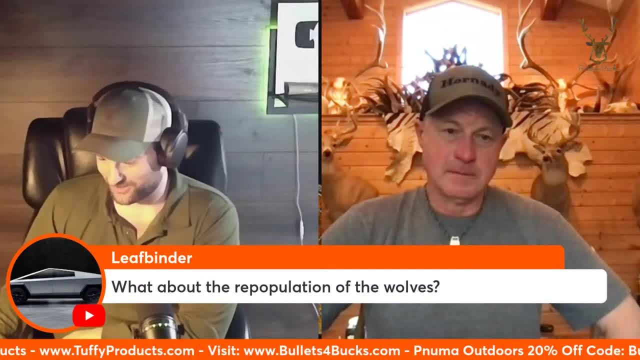 i've been out and find some turkeys. i go all the way up to the top of the mountain lion. i've been out and find some turkeys. i go all the way up to the top of the mountain lion, so he knows what i'm talking about. but uh, let's see. here we got some more comments, thanks for. 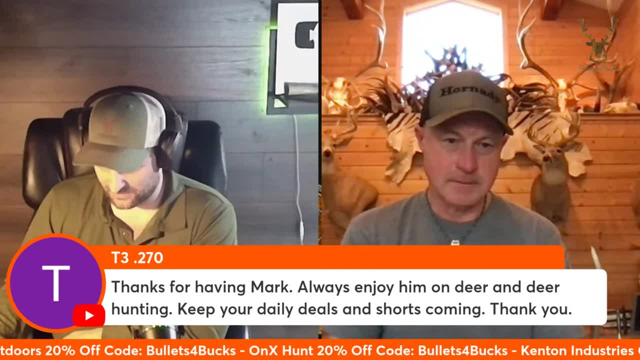 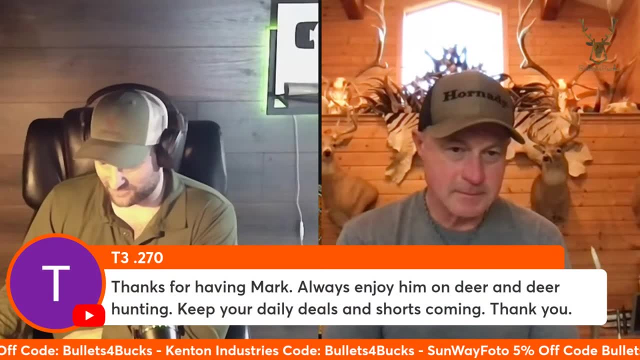 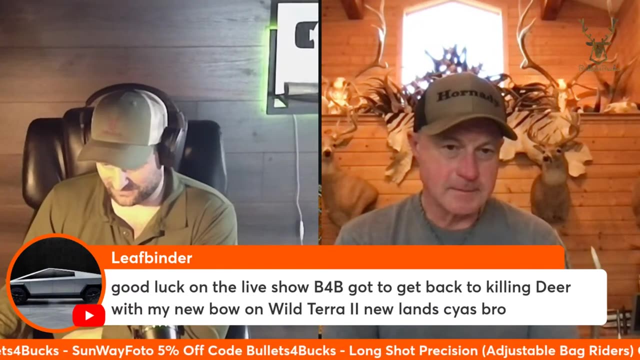 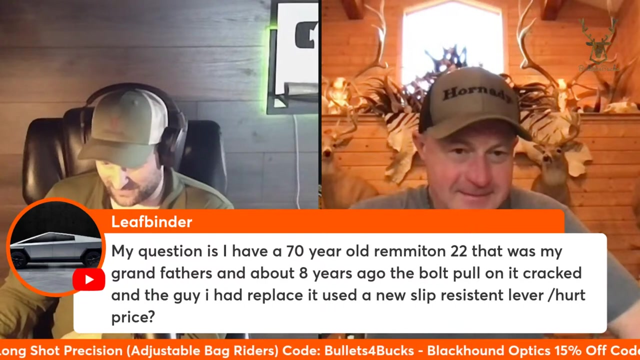 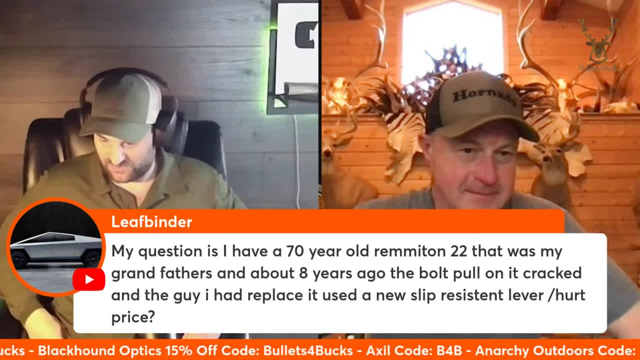 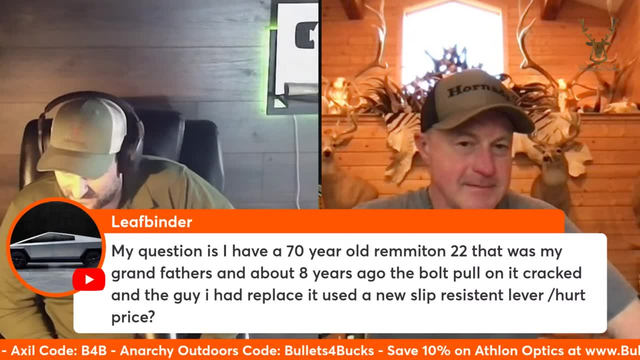 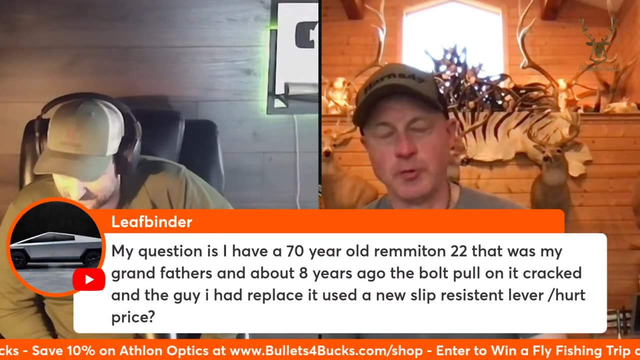 my grandfather's, and about eight years ago the bolt pull on it cracked and the guy i had replaced it used a new slip resistant lever. hurt price it proud. understand this? i do. he just had the rifle. he had a gunsmith fix the rifle and they didn't replace it with the original equipment. 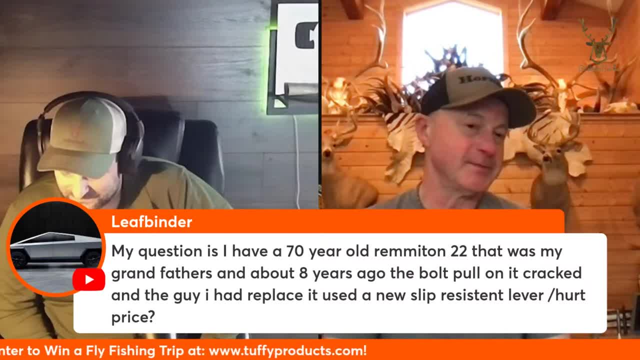 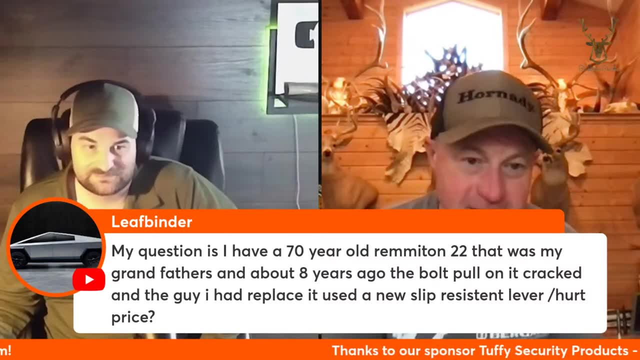 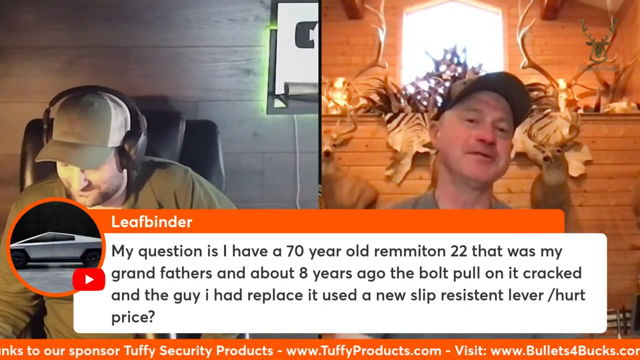 and typically that will hurt the price, but at the same time do you want to shoot the rifle. you know, and maybe there there was no way to get the original- a 70 year old um remington. it's not like there's just parts everywhere that you're gonna find. so i i would say 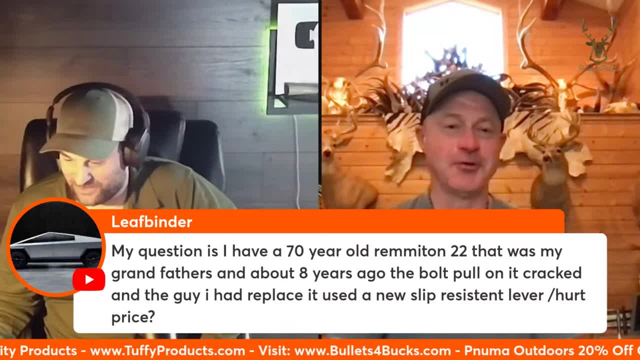 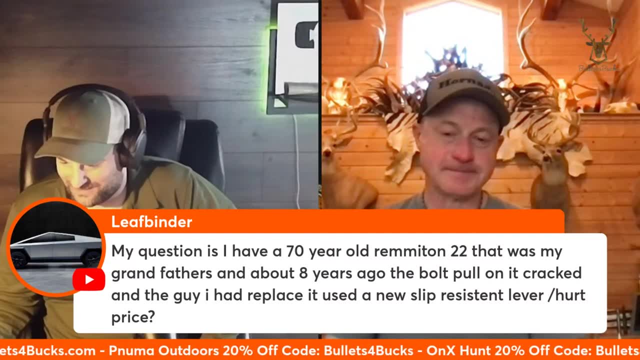 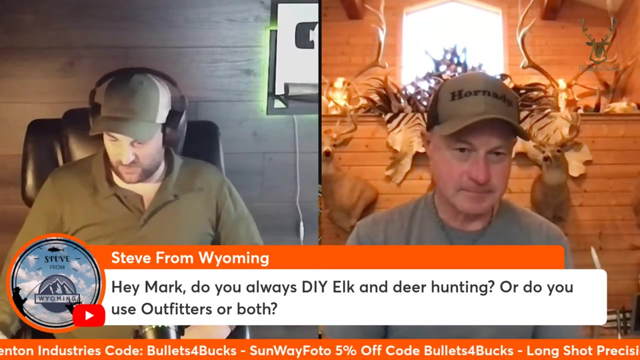 enjoy it, take you know, don't even worry about that, it's an heirloom. go out and have fun with it, enjoy it. i agree with that uh assessment there. i'm looking through here real quick to see if i can find some more. we got steve from wyoming. do you always diy elk and deer hunt or do you use outfitters or both? 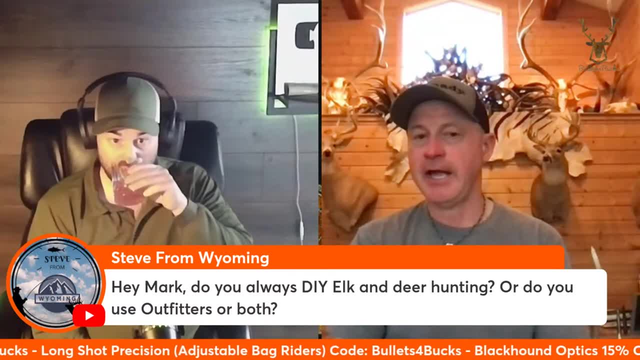 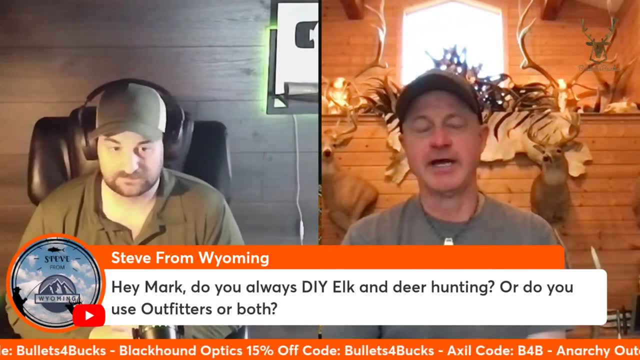 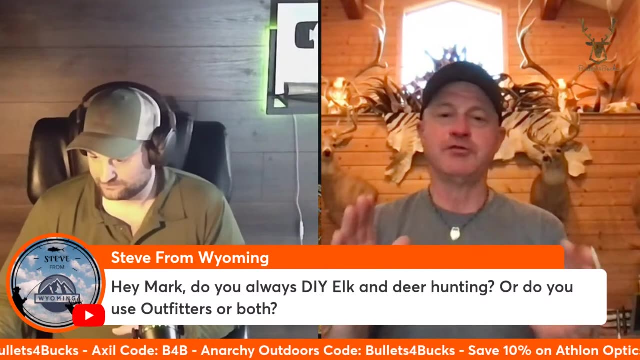 i almost exclusively diy elk hunt. last fall i did hook up with a guide in arizona because i drew a tag i'd been waiting on for 18 years, so i i actually believe i could have killed an elk there, no problem, it was just, it was just i. i work. 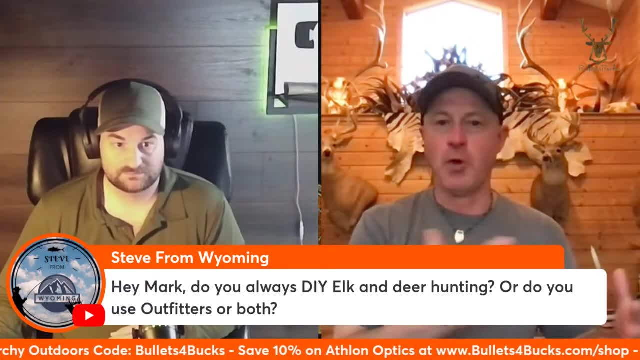 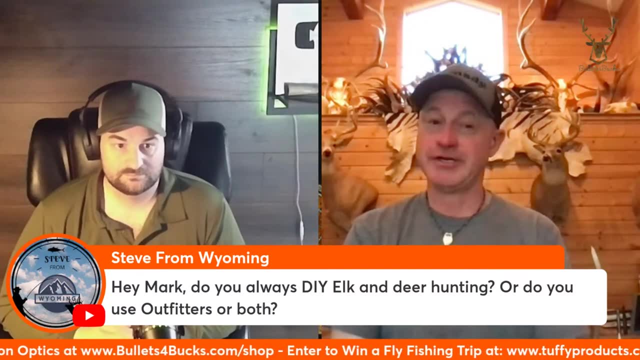 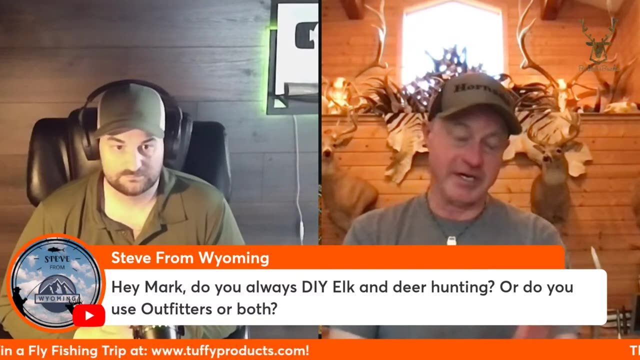 with a company called worldwide trophy adventures and they wanted me to team me up with this guide. so that's the first time i hunted elk with a guide in over a decade or a dozen years or more, so i really don't need one, but it was fun and i actually had a leg injury last fall going into. 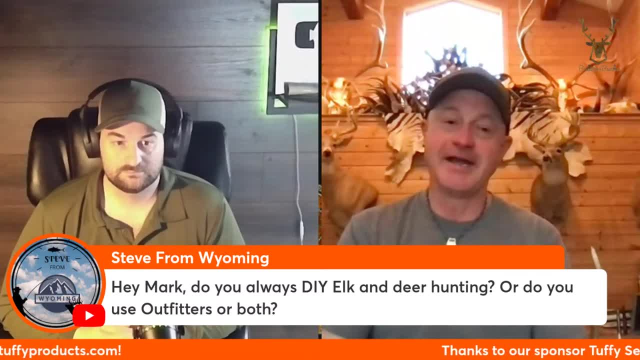 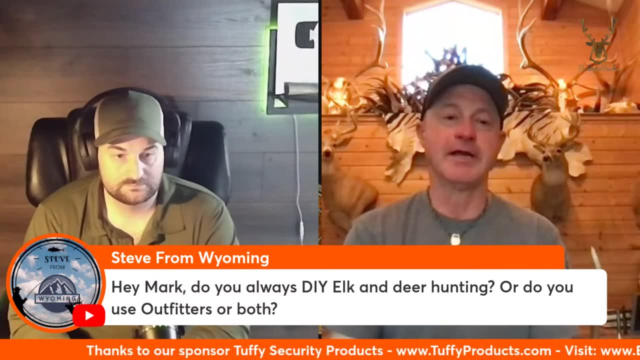 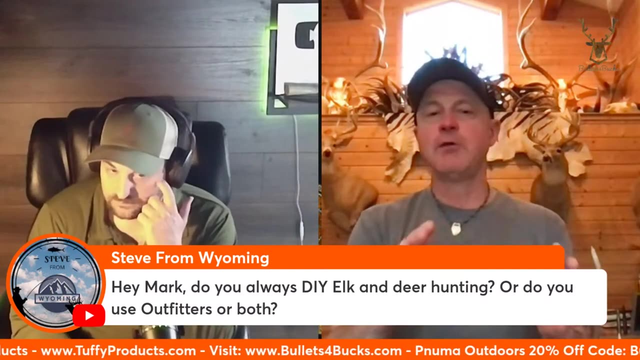 that hunt and i was a little nervous about, uh, packing an elk out by myself. every everything came out okay, worked out okay. my legs: 90, probably right now 95, but um, but deer is almost the same thing every once in a while when we're doing tv, though it does help to team up with an outfitter. 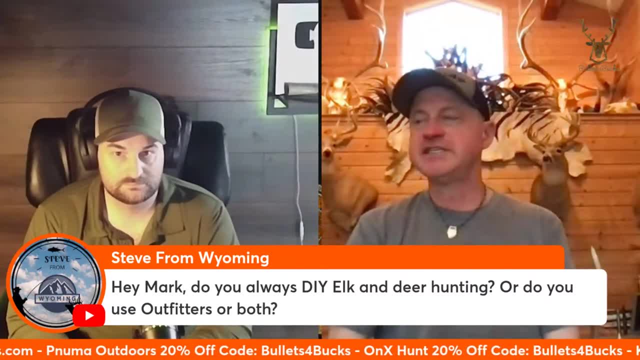 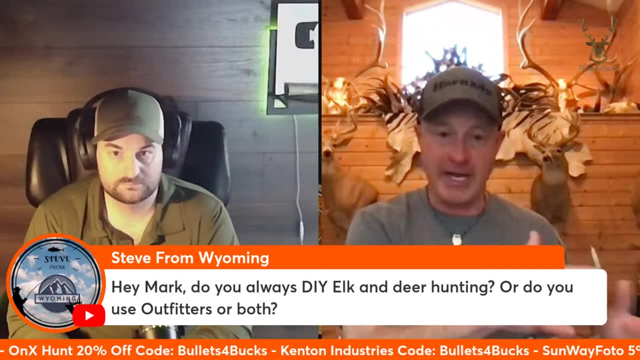 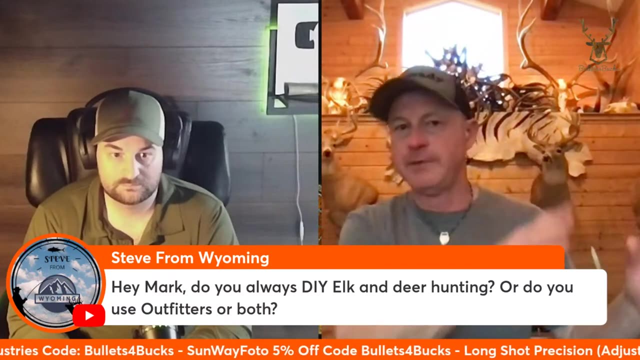 just to speed it up, because when we're filming tv, usually my window is four to five days- is what? uh, the company gives me to have a cameraman beside me. so we want to be efficient in hunting. it's not like going up here on the mountain or up in the mountains of montana or wherever, and trying to knock out a deer because 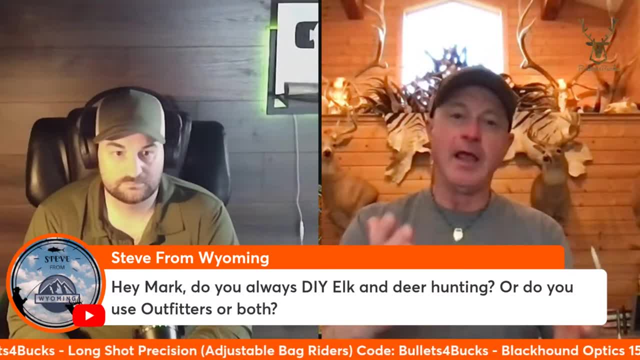 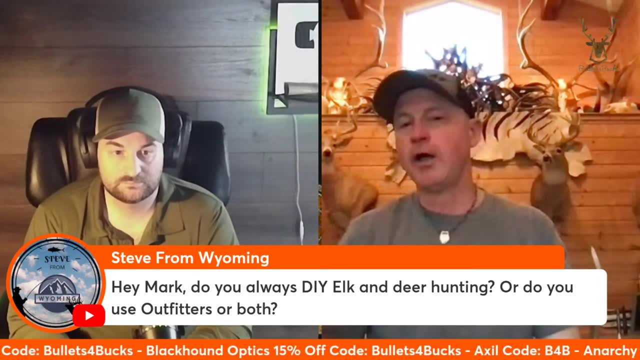 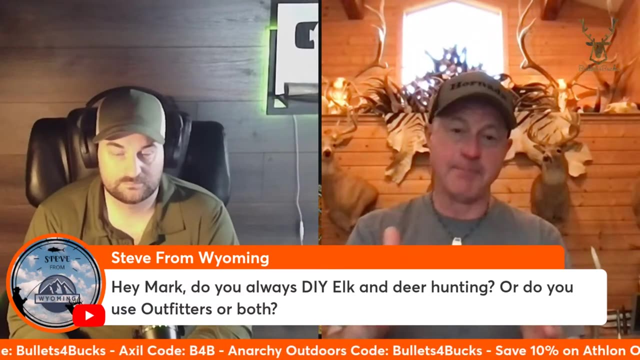 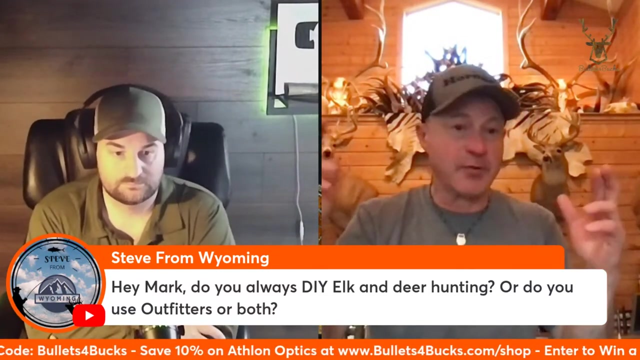 i do a lot of diy elk articles and the figure i use all the time is it's approximately 8 to 12 to 14 days on average is what it takes me to kill an elk diy public land, mostly in general units. not always, but even if i draw a permit here in wyoming, the permit's not like these hot permits. 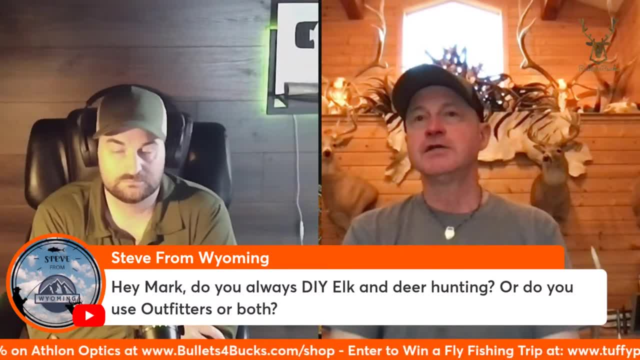 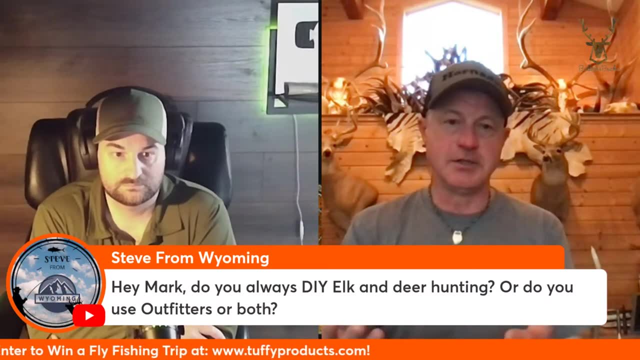 like i had in arizona. that was a good permit, but um so it's just hard. it'd be about the same, i figure, with the deer. you know you're gonna spend six, seven, eight days trying to get that deer killed and i don't have that much time with the cameraman. so my deer hunting mainly i'm going to. 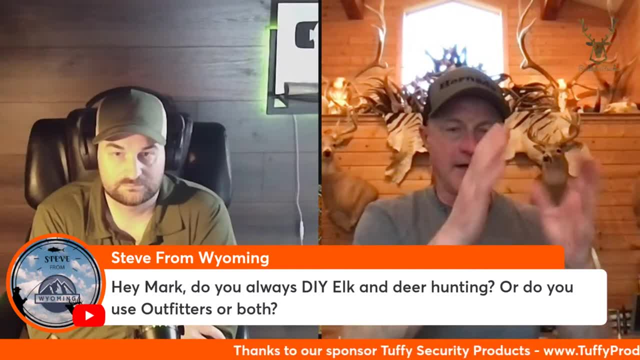 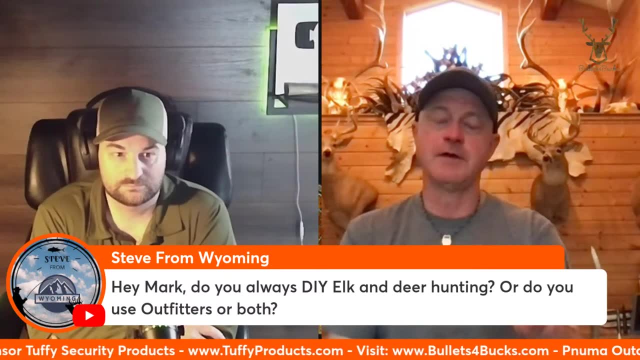 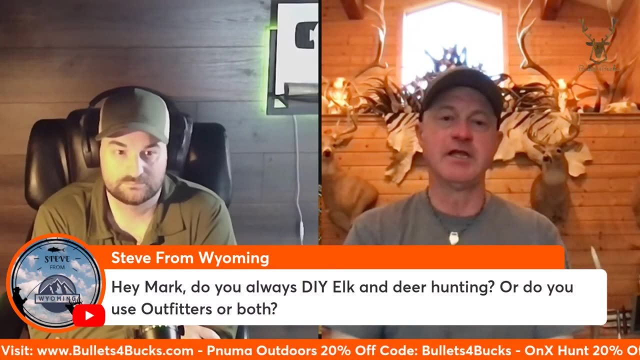 do is with buddies who have land and uh. i. i've got a really good friend in kansas. we team up with and film some hunts there. when i can draw a tag, that tag is getting harder to draw. and same thing in south dakota. i meet up with a buddy. we hunt land. he's got some of his family land and uh and. 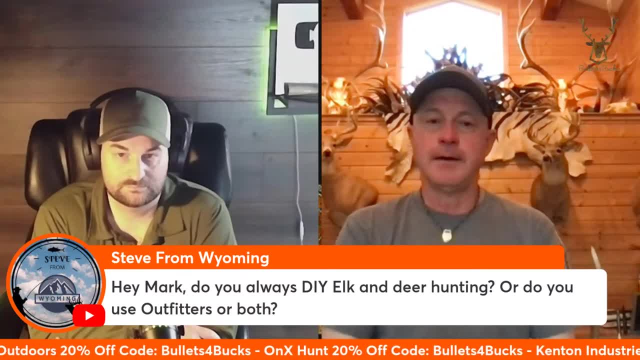 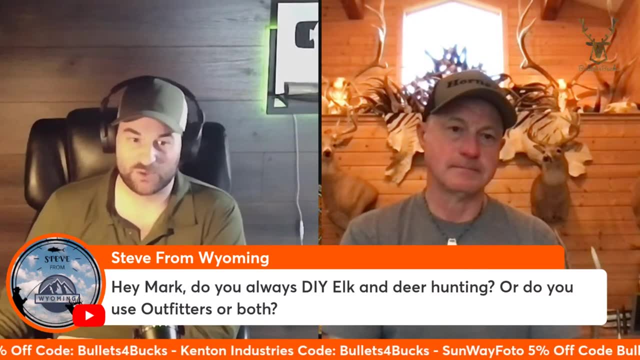 then occasionally we'll team up with an outfitter. so uh answers: yeah. yeah, i know from self-filming man it is so hard to do that, but i'm going to do it and i'm going to do it and i'm going to do it. 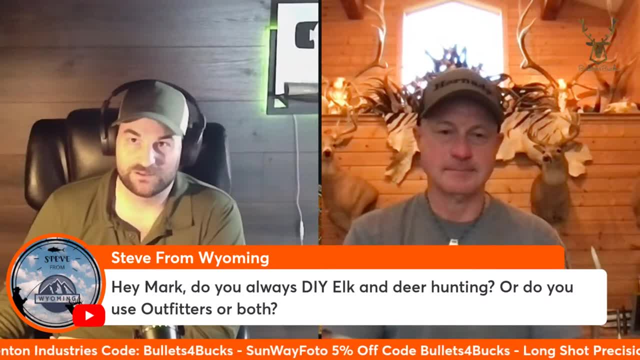 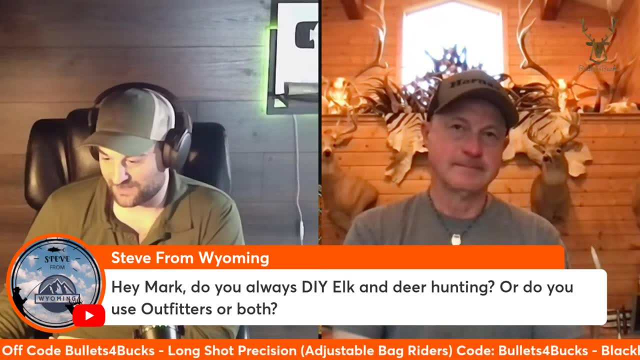 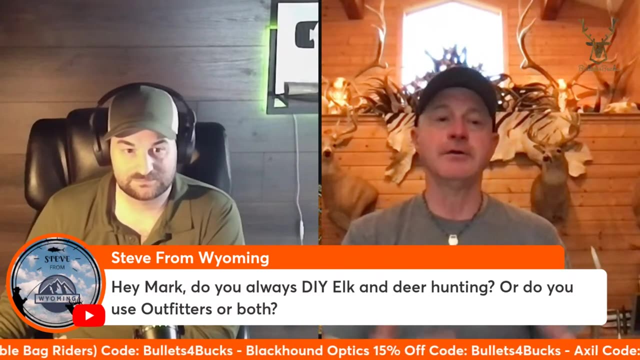 the self-film hunting and have the film come out well, and get the shot on film. oh my gosh, it's just, it's. it's really difficult, in my opinion, anyway, um, and some guys are good. i know a couple of guys that are just. uh, one of my coyote hunting heroes is a guy by the name of john collins, out of 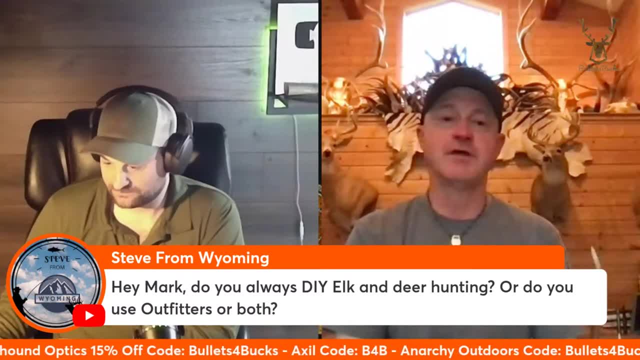 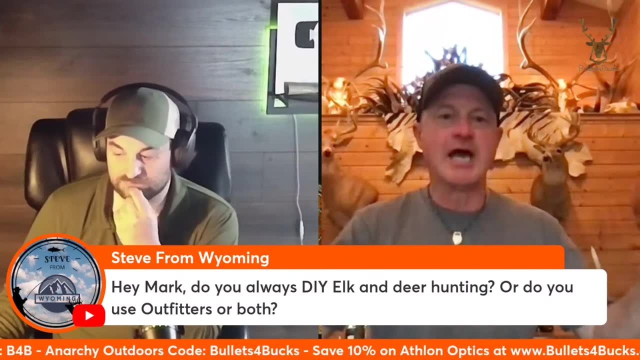 kentucky. i follow his stuff routinely and he sell films all the time. but his country's a little different, like in our country, and you know the steven when you get on that stage where there's a lot of rolls and folds and, uh, coyotes can come from 360 and they're there an instant and gone an. 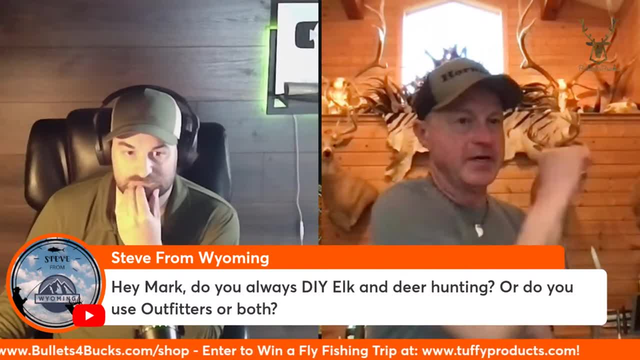 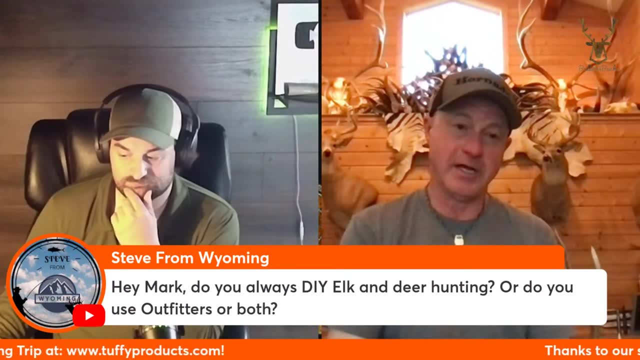 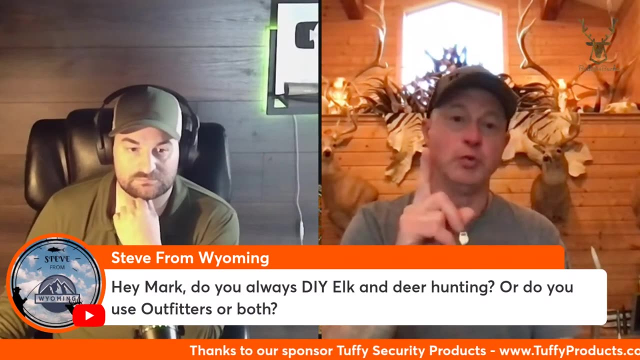 instant. so trying to film. you know i'm gonna turn around over here and everything. well, the coyote sees that he's gone and uh, and elk hunting. i always figure on a diy public land elk hunt. i'm gonna get one opportunity in a week's hunt, uh, and maybe one in two weeks, and so right am i? 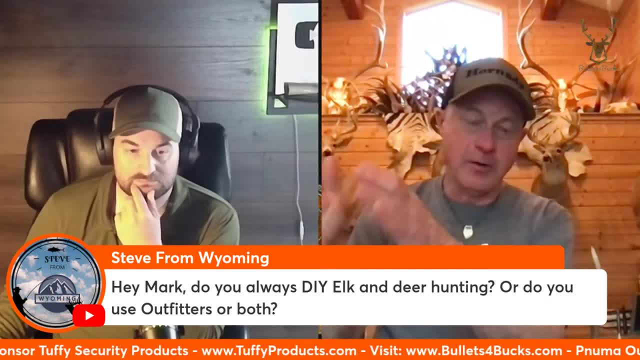 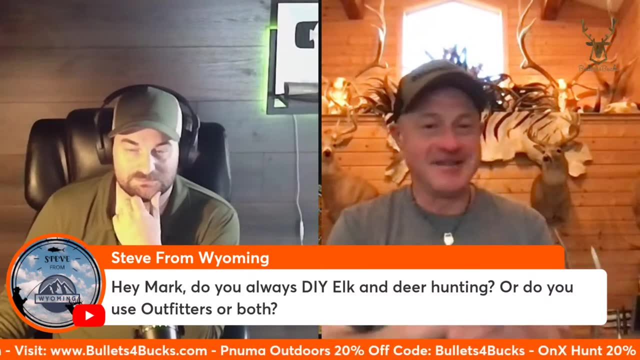 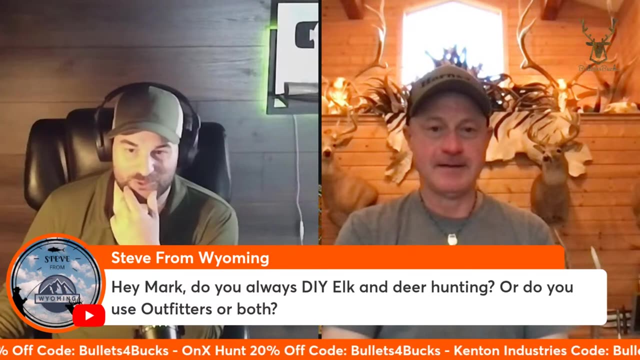 blow that one opportunity trying to film it? or am i gonna make sure i secure a winner's worth of meat for the kaiser family by getting, and then just now? yeah, so i miss a lot. i miss a lot of shots on film. uh, self-filming for sure, um. 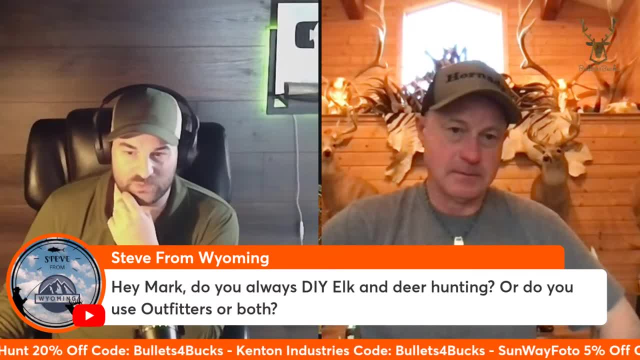 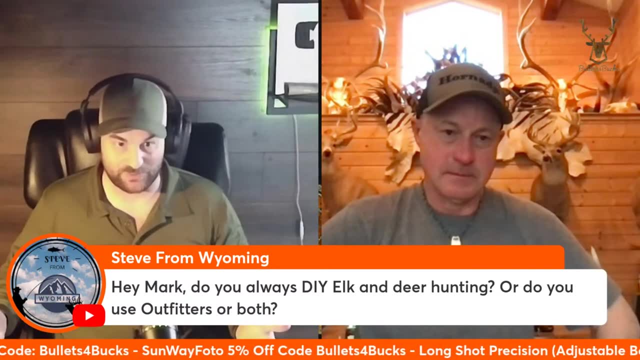 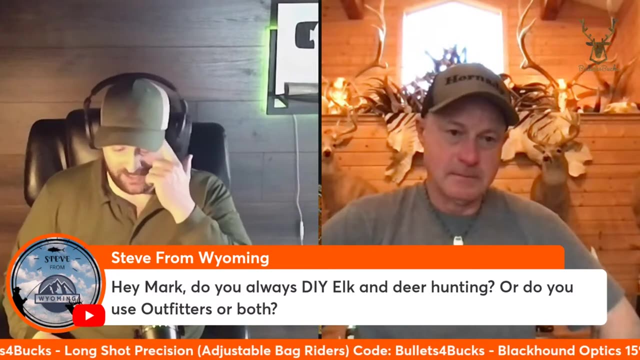 i think now my last elk season was actually one of my- well, as far as out of my successful seasons, because not all have been successful for me, but out of all my successful seasons it was actually one of my hardest. um, it was pretty difficult for me for some reason, which i guess wyoming game and fish uh reported. though 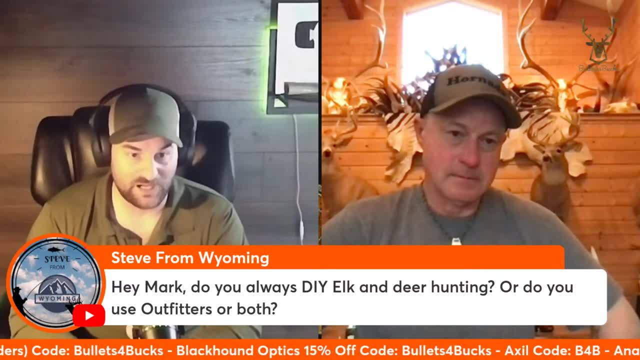 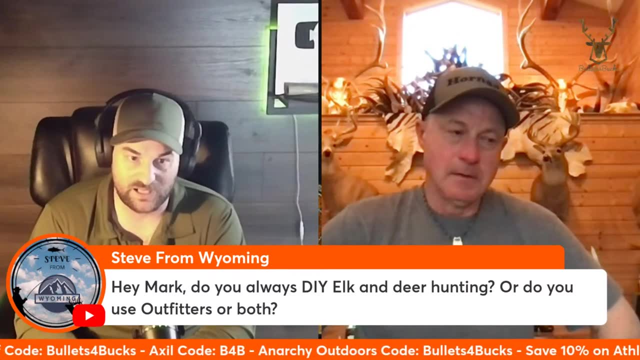 that it was the best elk season in like history or modern modern history. uh, how was yours? i think you didn't. i, if i recall correctly, you were out a lot of days, if i, but i think, because i just saw posts come up and you were actually hunting yours even after i was done. so did you put in a lot of? 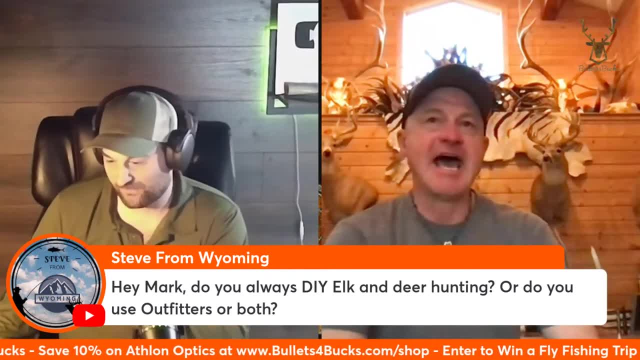 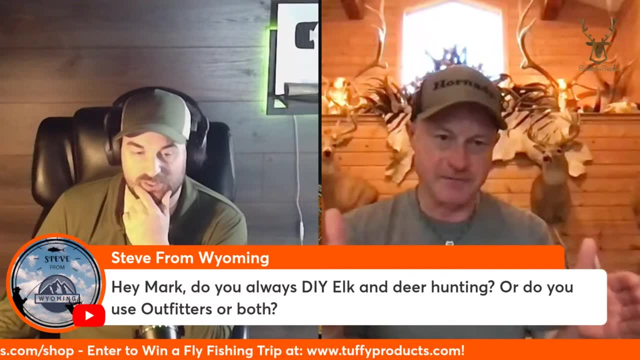 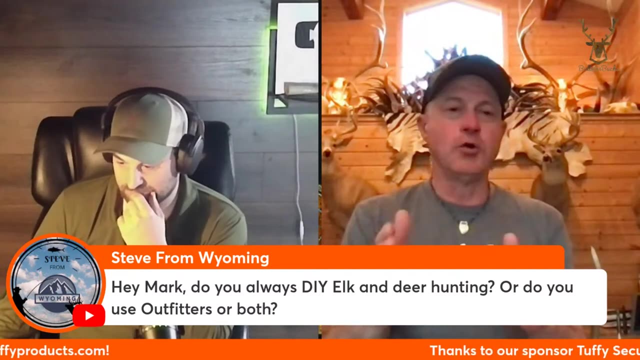 time last year, or how, how was that? i hunted nine, ten, ten of the 15 days of what i was in the field. and uh, the reason i? i, as i get older, i feel like i get smarter. so when a big winter storm comes in and, uh, you know, it's just white out, or those, you know how. 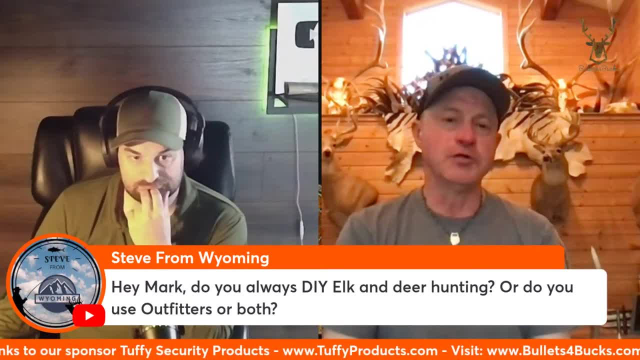 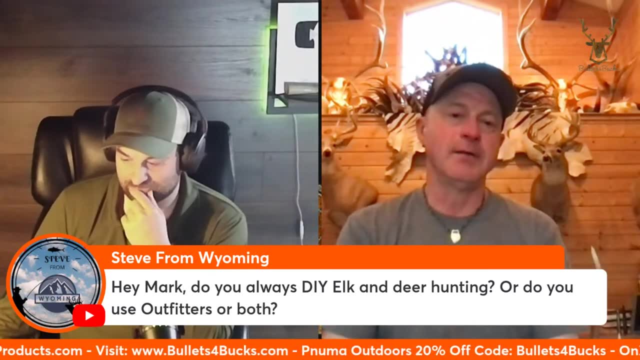 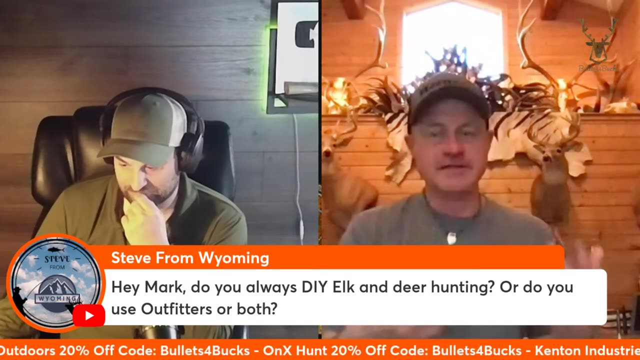 that heavy fog comes down the mountain and you can't already see those days i i tend to take off. it's like i can right, i'm hunting close enough home i can uh, blow home, rejuvenate, get a good shower, get a couple nights sleep and then back in the field. and- and this year, like you said, it was, uh, it was a strange season. 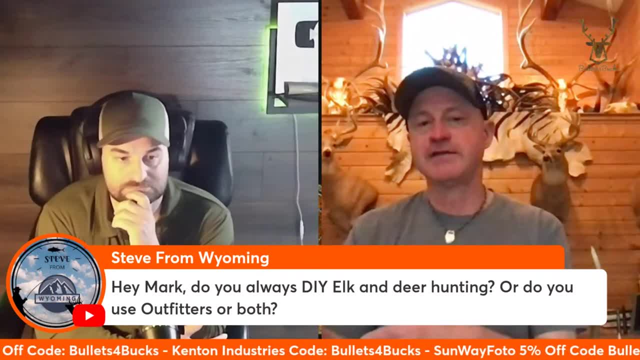 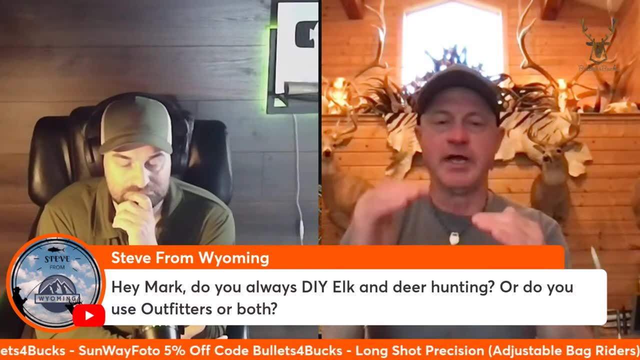 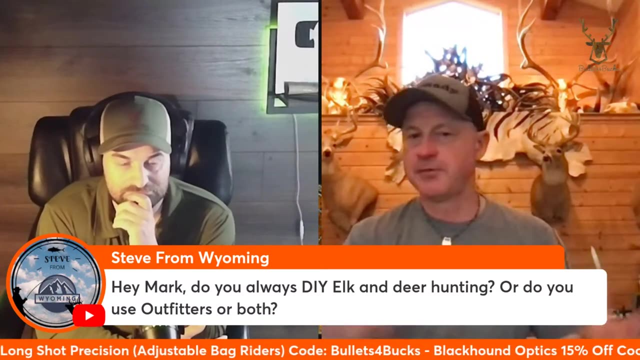 it started out hot where i was hunting and then it transitioned to, uh, you know, horrible winter conditions. but i took off at the very end there. it just i timed it right. a storm was just ending. i was home during the storm, drove back uh late one afternoon, slept, got up three in the morning. 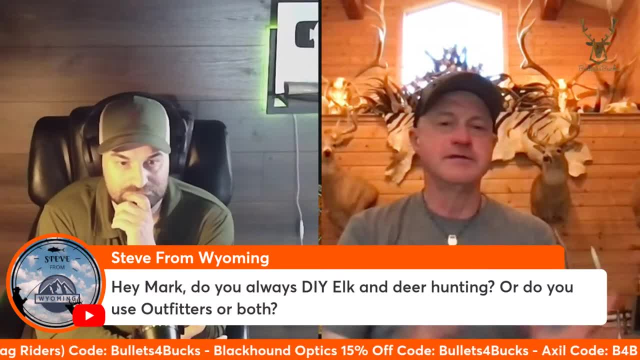 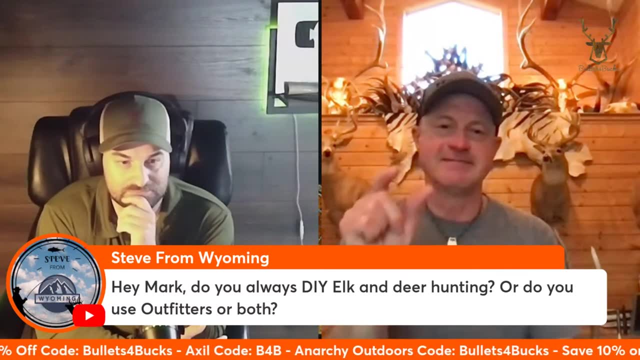 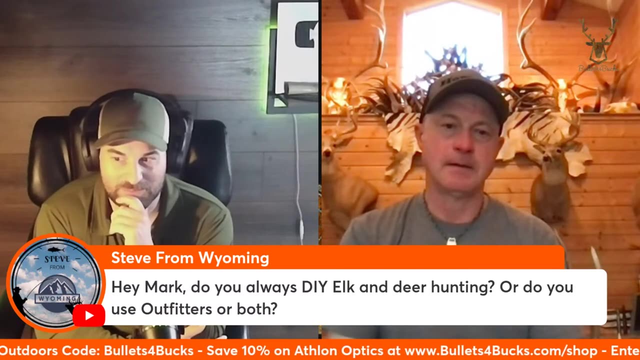 did my hike in storm, broke moon, come out, this prettiest hike i you know i can imagine in a long time. i got up there and, uh, a bull gave me just that much of a window to kill nice mature bull. so yeah, i, i'm getting a little smarter. maybe i don't know. i i think i used to. 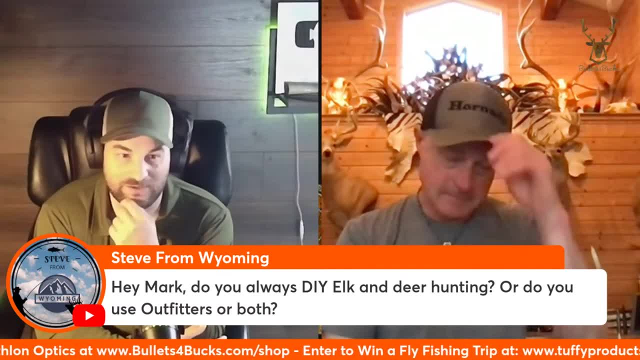 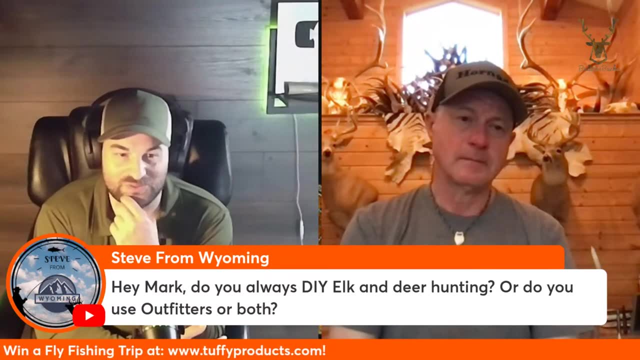 always just go through, literally hunt right through the blizzards. everybody'd leave the mountain. i'd still be up there in the blizzard, but after so many injuries and so many close calls and so many long nights, you know, stuck in snow drifts, it's like, at some point, the return on investment. 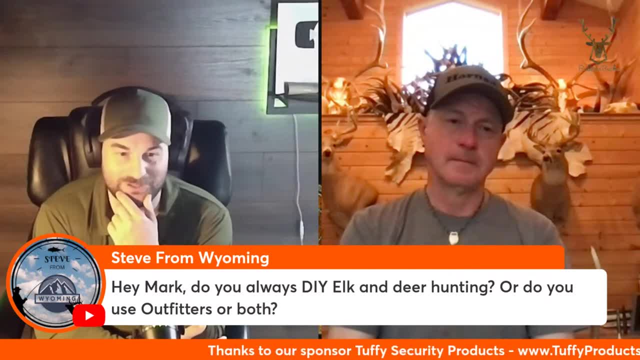 isn't always worth it, and i think you do eventually hopefully learn that, and that's kind of where i'm in the i'm the process of learning that like, okay, it's just not worth it today, uh, and it's probably, you know, those days they're probably not going to be successful either. 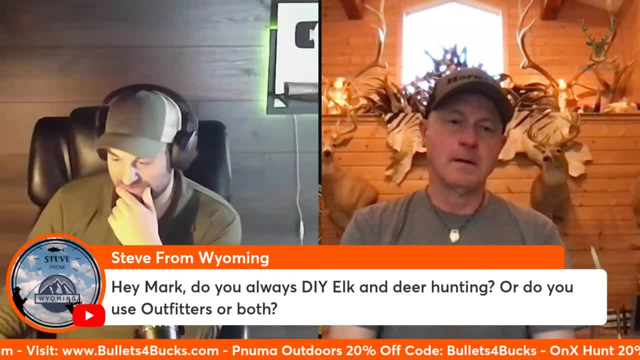 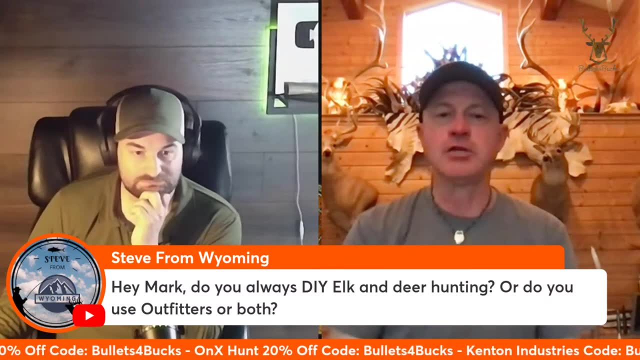 and so you just learn that and you start to make better decisions and burnout in elk hunting, diy public land elk hunting burnout is so real and and i i lose all my hunting partners. even when the weather's nice day, four or five they're bailing on me. 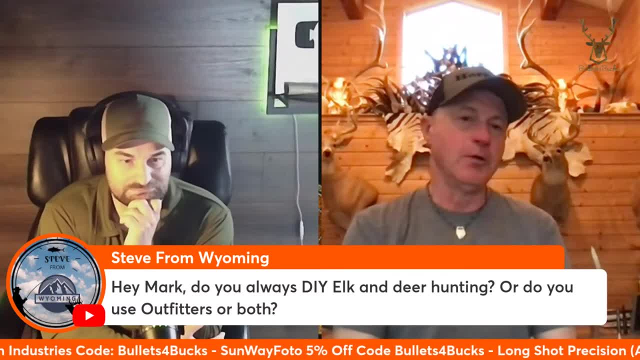 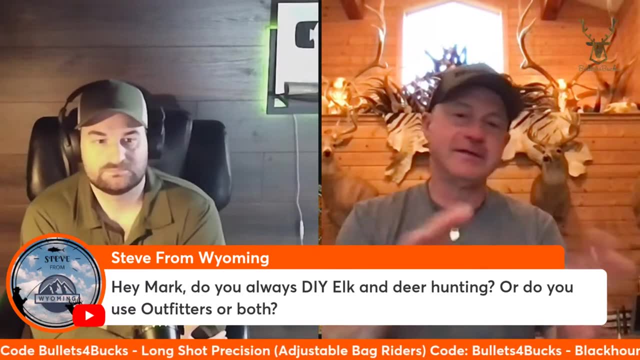 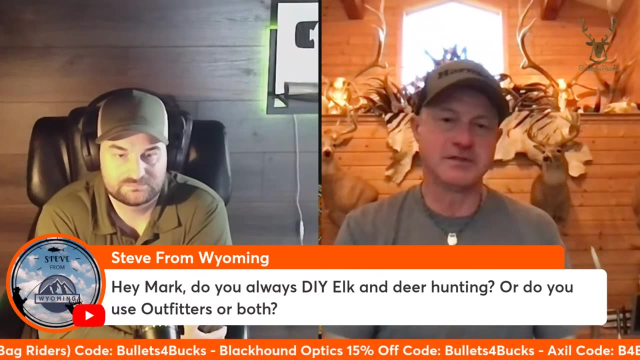 they just they're, they're burnt out, they're worn out. uh, we're not seeing elk, you know their spirits aren't up. so i i think taking those days off. if you can't- now you say you're living in philadelphia and you drive out to colorado- you've got to do the six days straight, or whatever. you know, it's just. 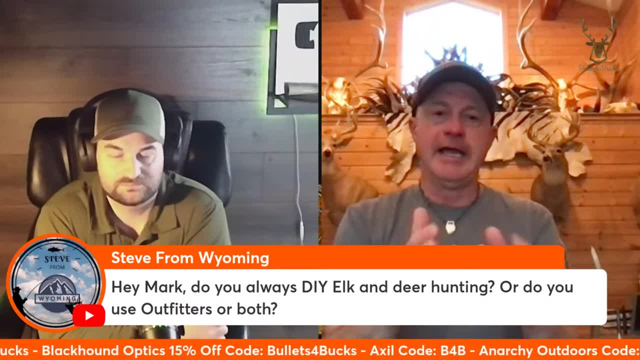 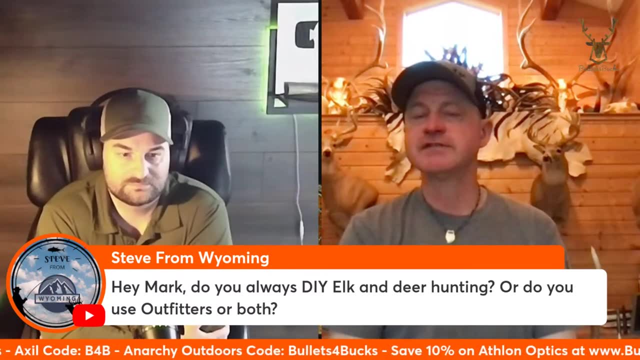 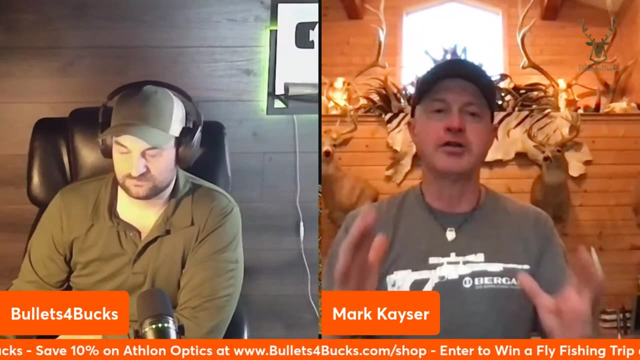 no doubt about it. but another little thing i do and i started this back in, uh, 2016, probably 2017, somewhere there is. i began to do a lot of hunting and i started this back in 2016. i started again. if i didn't want to hunt all day, i would always hunt hard the morning hours. i'm a morning. 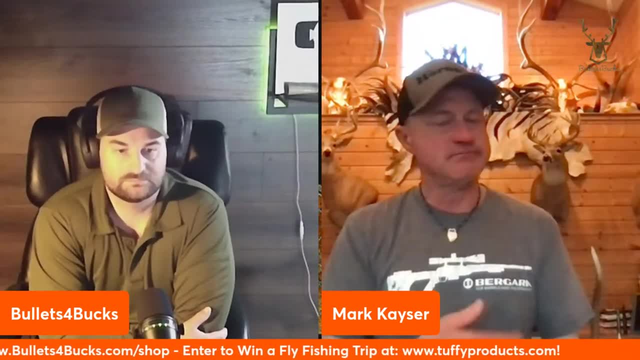 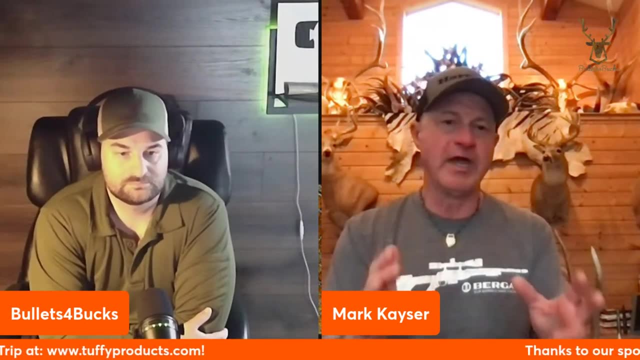 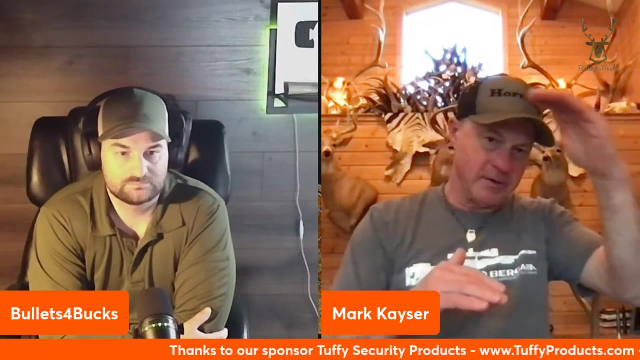 person anyway. so i get up extra early, three or at the latest. i try to get in the woods. i want to be in where i want to be before shooting light and sitting waiting to hear the elk. and in another tactic- and i write this a lot in my articles- is i like to start above the elk over here. 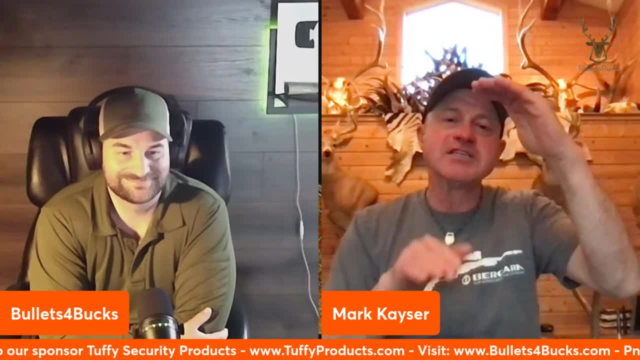 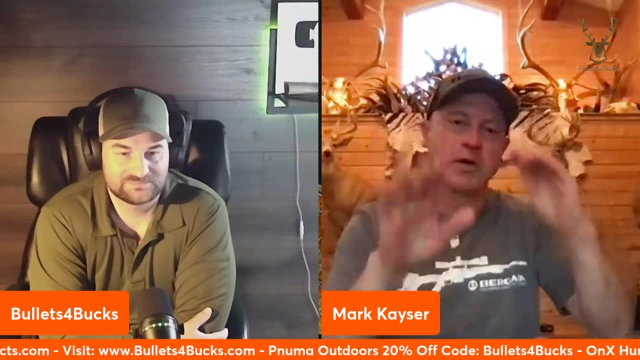 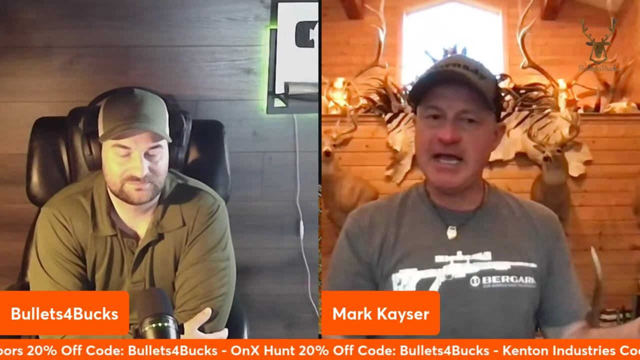 and oh, typically on public lands- work up, not all the time, but the majority of time. they're down low feeding and they work up. so i want to try to be where they want to be and then catch them there and then, late in the day, if if they're not bugling, not doing anything, or if i'm rifle hunting, i just 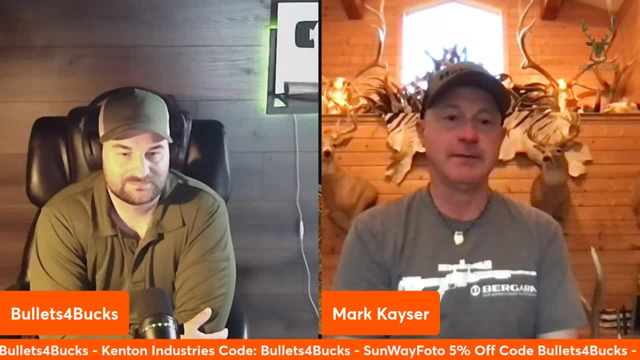 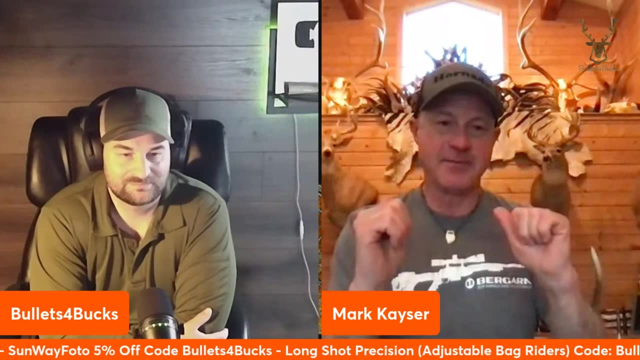 don't have a good feeling. i go back to camp and get a full night's sleep. i just don't stay there till dark. because if you try to do morning early morning, stay till dark, get back to your camp, you know, unless you're bivvying it or in a 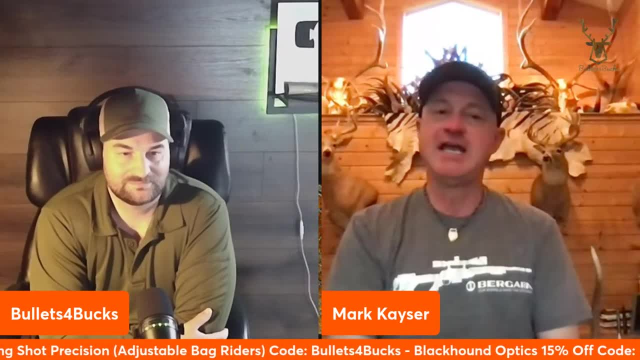 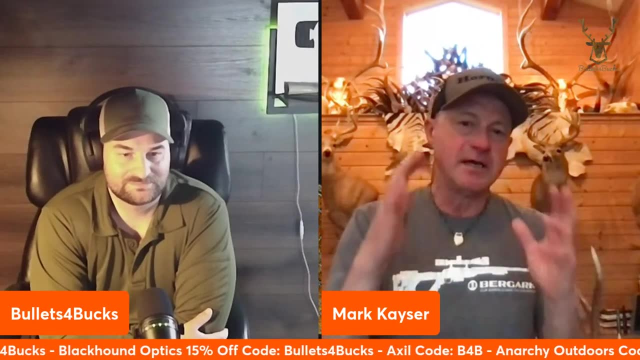 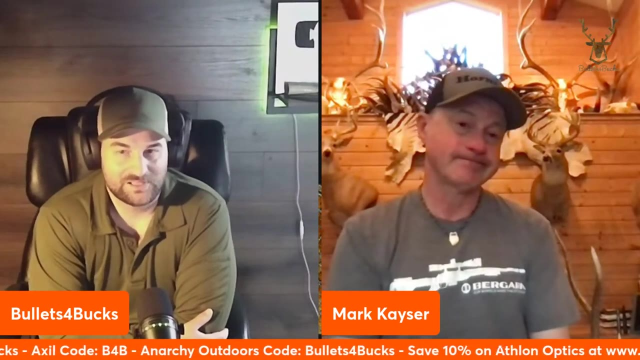 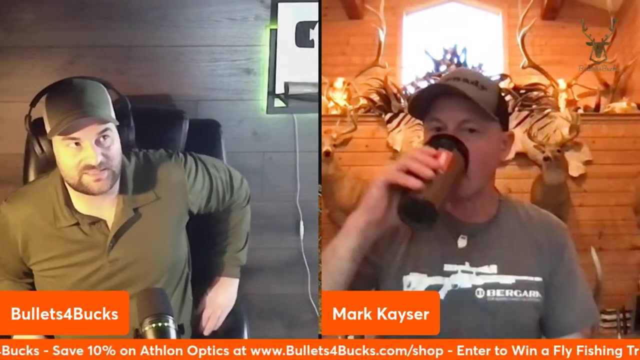 backpack camp and you're just right there living with the elk. those days are horrendous and it's really me become. it keeps me energized and focused and, uh, it's working. i'm killing elk, so i'm not. yeah, yeah, i spent. yeah, i've had the last two elk seasons, or at least this last season i spent two. 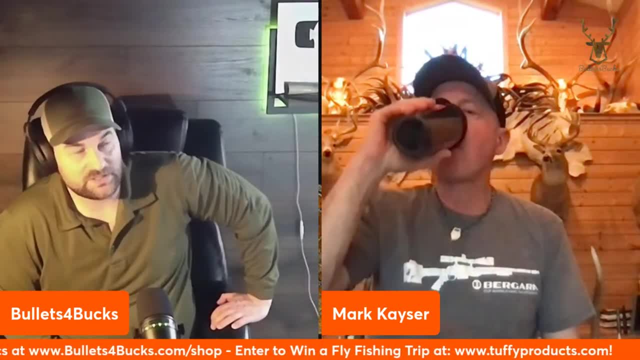 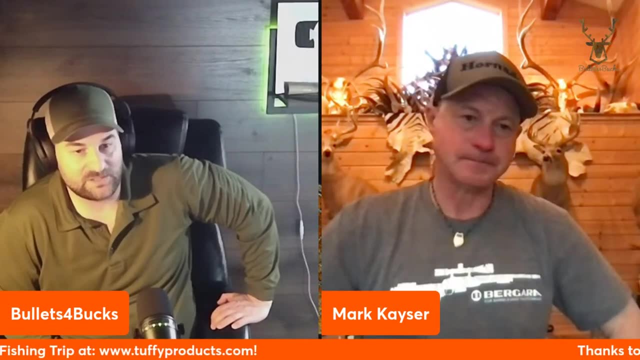 or three, like i'm talking out at three in the morning and then coming back in the morning and coming back after dark by myself, and i never came back and i dry. i just sat out there like just dry snacks and mentally it started to like just make me angry, like it's just the middle of. 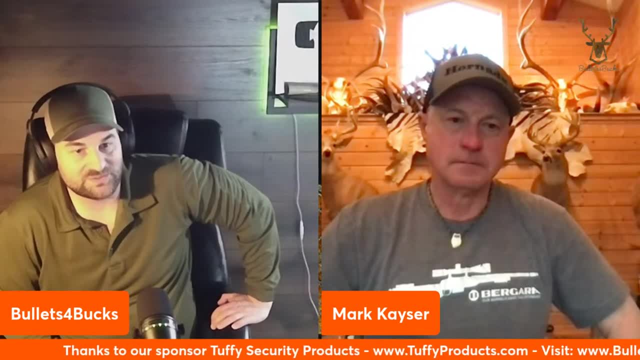 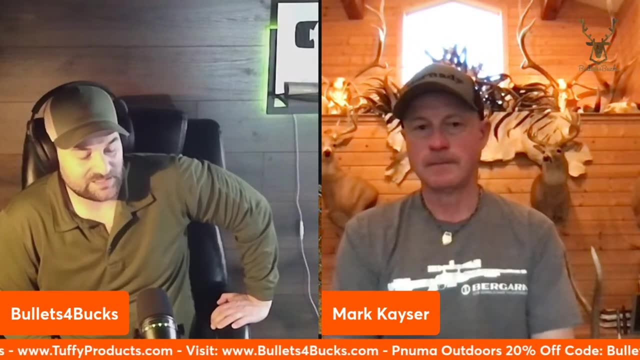 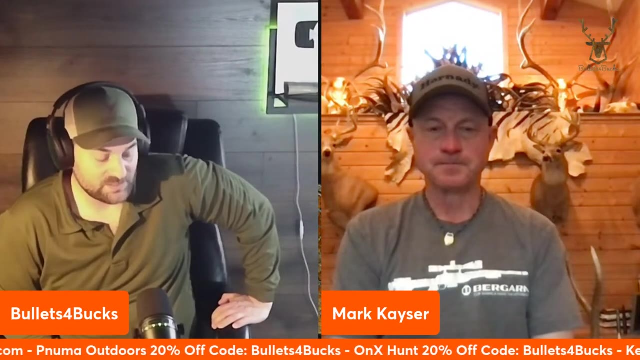 the days were so boring that your mind just kind of just i mean deteriorates a little bit. but uh, yeah, you definitely have to pace yourself, i think. i think that is an important aspect of it, i think, when it comes to elk hunting, well, most hunting in, but even maybe more so, elk hunting on public. 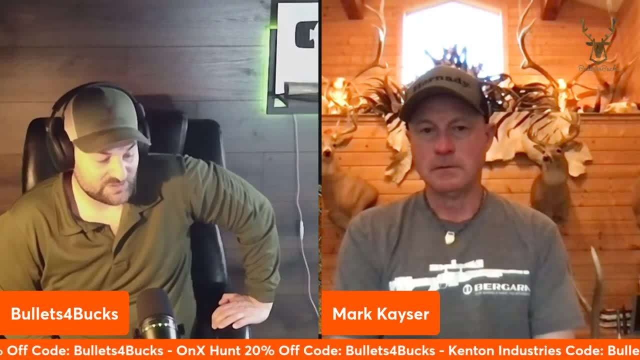 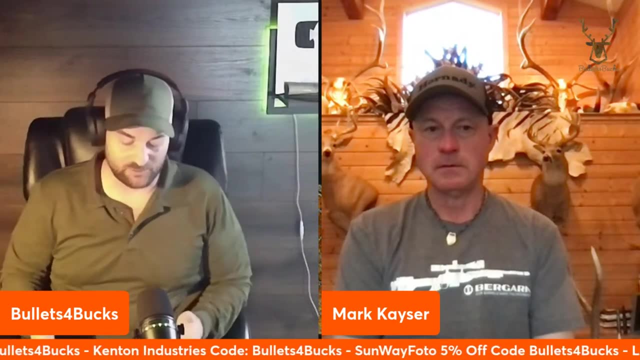 land. it's like the one tip i always have is like persistence, persistence, persistence, persistence. like if you can do one thing, you can screw up a lot of things, but if you're persistent generally, i feel like you'll eventually fill your tag. now some people- i mean they don't have the 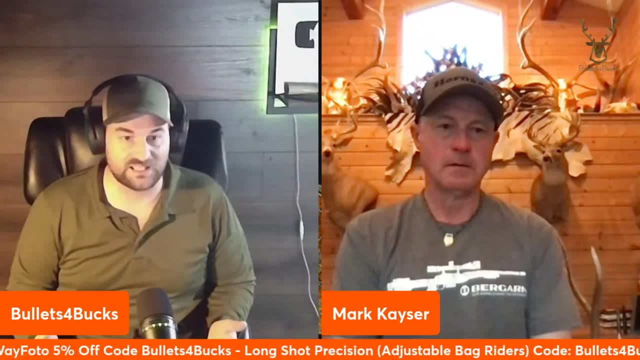 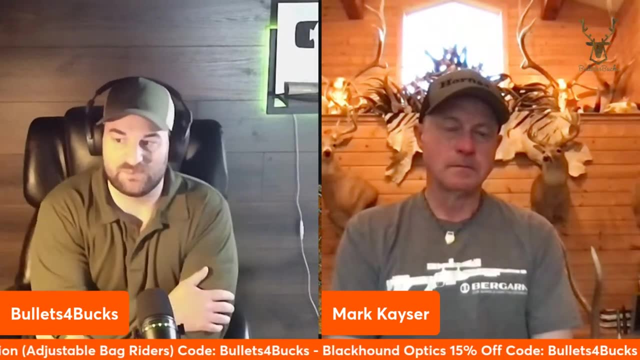 luxury, like maybe you or me, where they can hunt 10 days. they might only have five days, so i get that, and that's probably the majority of people actually. but if you have the time and you're persistent, i feel like, generally speaking, you'll eventually be successful. 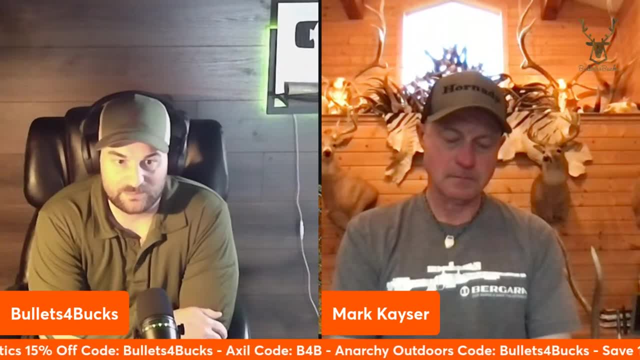 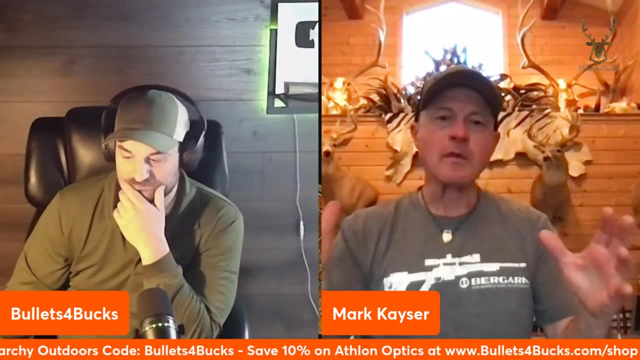 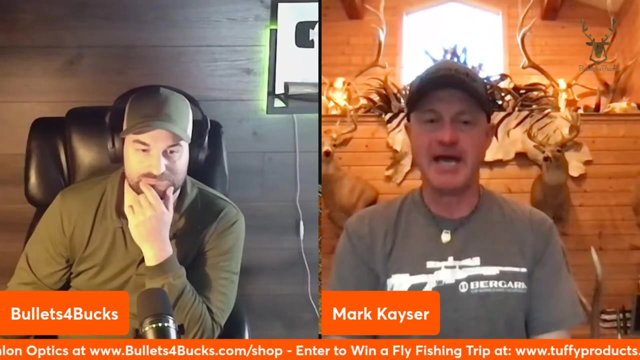 in elk hunt, um, at least on a cow or something like that. but- and i tell people that too, you know my average hunt is 8 to 12 days. if you're going out west, and especially if you've drawn a premium tag, definitely block out the biggest chunk of time you can, so you can take a day off for an. 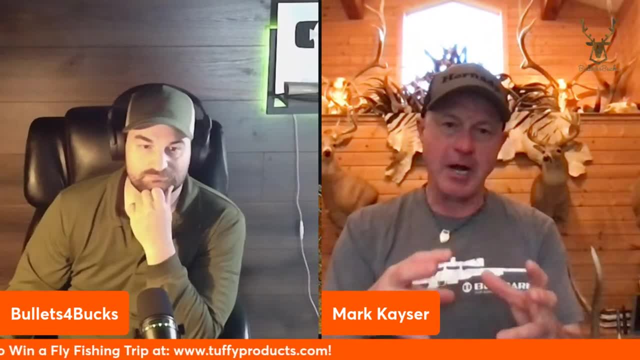 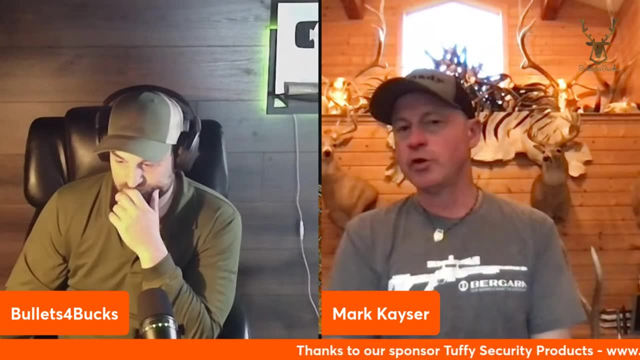 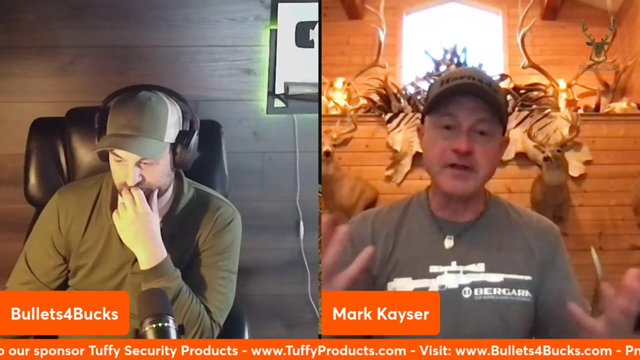 afternoon off. you can control that burnout and then get back into the hunt and uh, i mean sheep hunting, elk hunting, some of those more extreme hunts- they're they'll, they'll eat you up. that's why, when it comes early november- and hopefully i got an elk tag uh, filled- i love going to whitetail camp and we sit in. 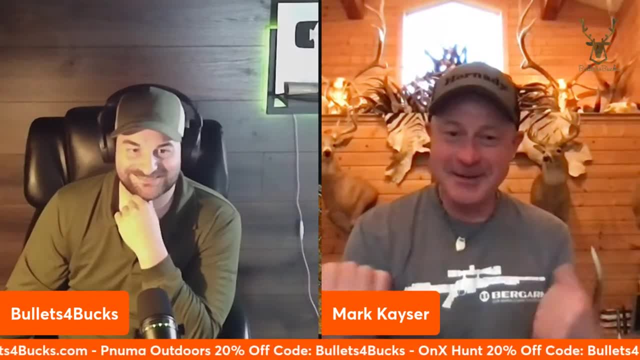 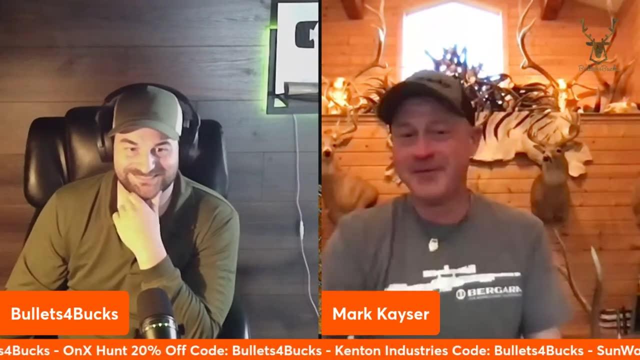 blinds and sit in tree stands, come back to, come back to the farmhouse in the middle of the afternoon, eat doritos and watch- uh, watch espn or a movie or whatever- and then go back out. i mean, to me that's just like that's, that's just 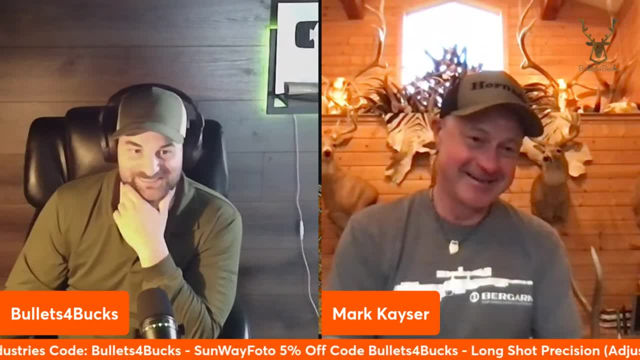 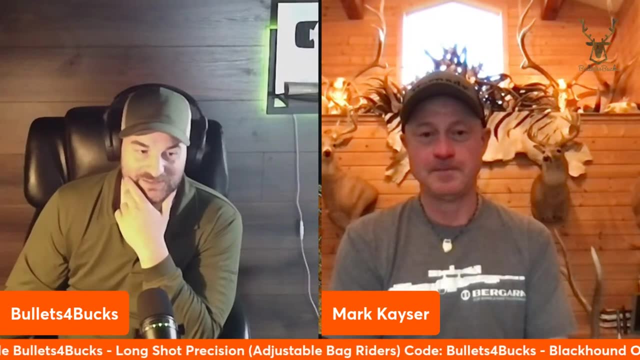 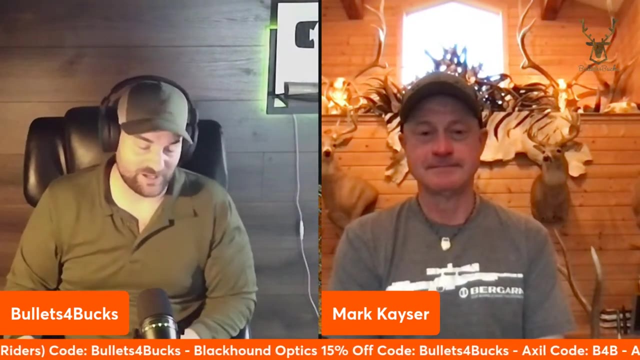 yeah, i think the weather i mean. well, it depends where you hunt elk, but certainly, like october, depending on where you're at, can the weather can be extremely brutal as well. that's something i feel like for non-residents especially, it's like, or even some, even a lot of residents. they 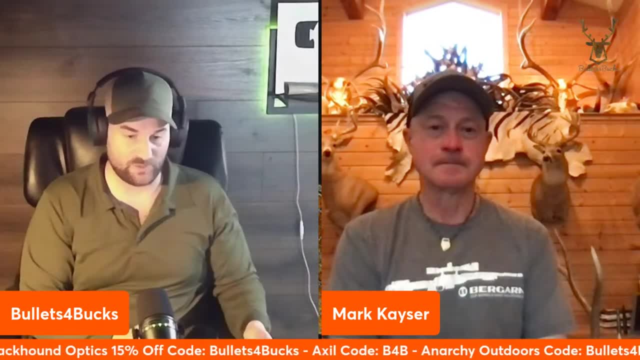 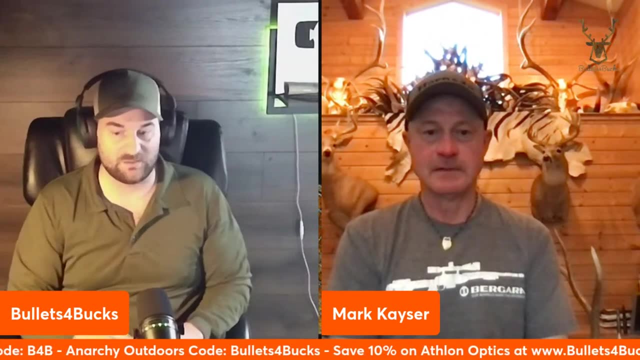 under prepare, like with being prepared for that weather to come in and still being able to sustain a hunt through it, um, even if it's just staying at camp, you know, um a lot of people. i think that's where they fail as well, where they kind of give up and they're not persistent. 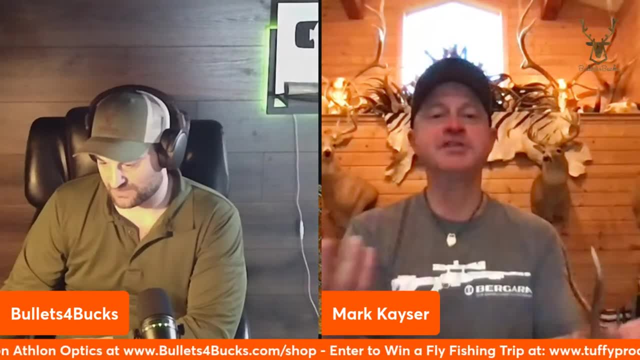 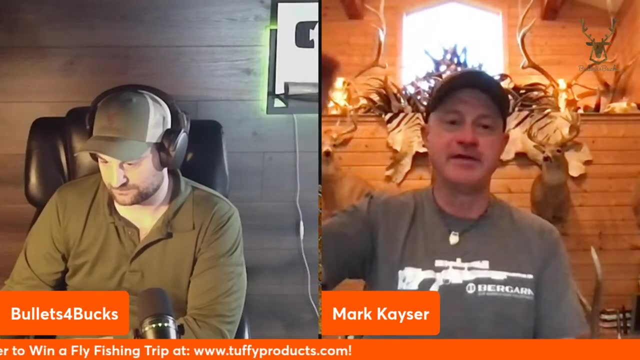 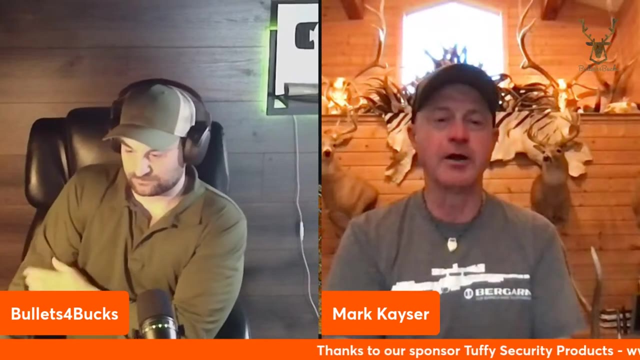 um, i teach that too. pick the right camp. i mean, and i see so many people put their camp at 10,000 feet or 9,000 feet and it's like in those october- you know, the last half october- like our elk season. 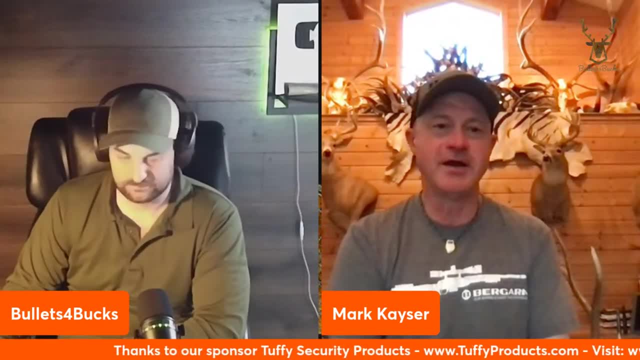 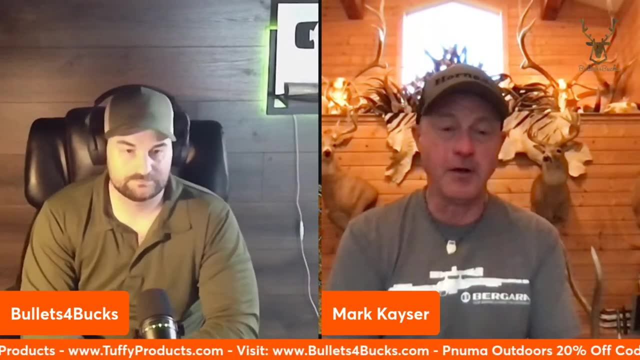 is. it's like, dude, you could just get snowed in there and never see your camp again. i mean you can get two, three, four feet of snow overnight and see if you can get snowed in there and never see some of these big, you know, late fall storms and uh. so i really monitor that as well and i have a 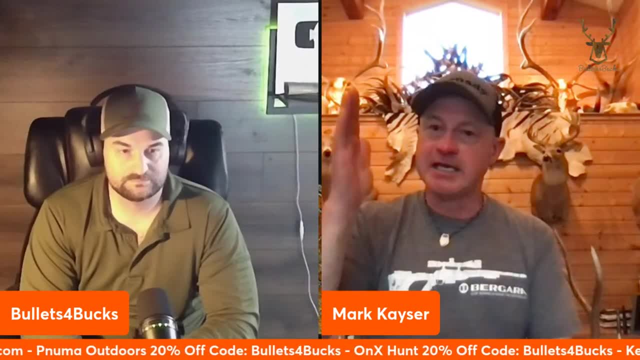 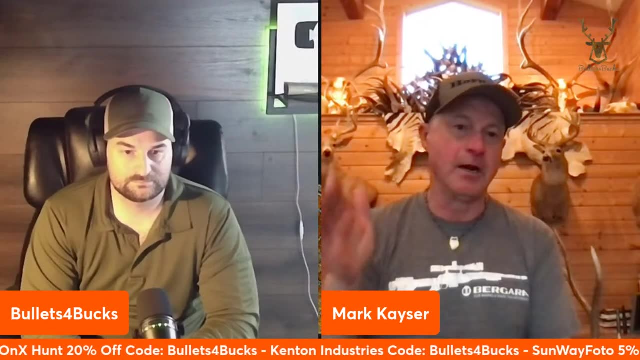 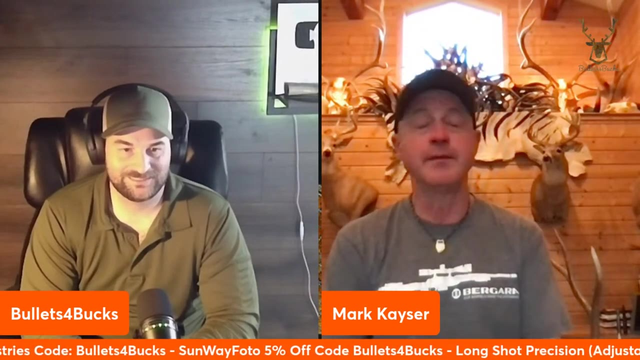 mobile camp. i use my horse trailer. if it looks like i can get away with 10,000 feet or wherever, i'll camp there. but i'm watching that weather all the time so i don't want to get stuck there. i want i. i definitely have backups down the mountain. i can uh go move my camp and uh be in a little bit. 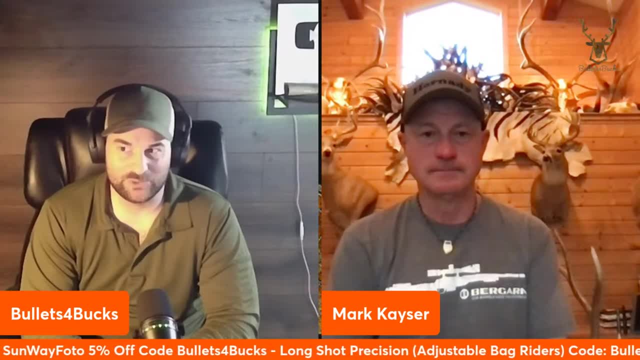 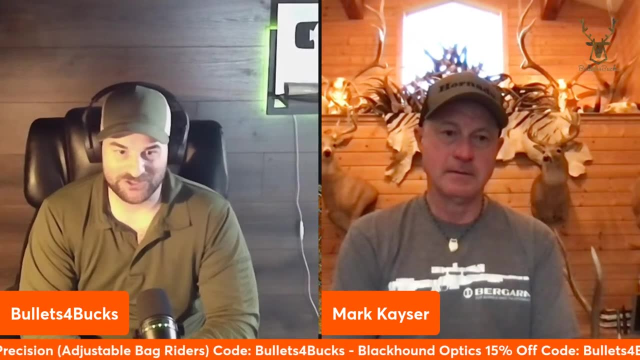 better area. yeah, i've made every mistake in the book and it took me 60 days of elk hunting to get elk. so i've, and i got everything from walmart, you know, on clearance to start hunting. so i've definitely done everything wrong, or or, you know, self-taught to begin with, but i guess once you 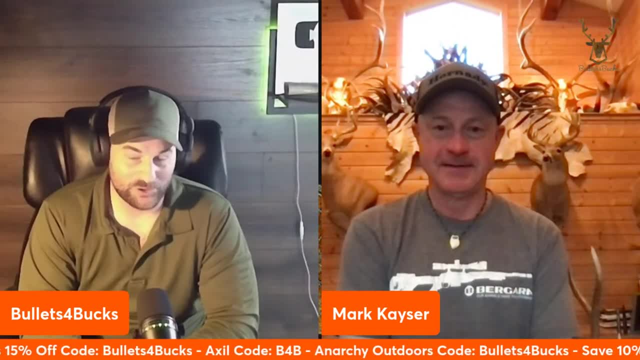 learn it the hard way. sometimes you don't forget. it is easy, um, or you appreciate success. i think that's the biggest thing, man: you really appreciate any success, even if it's a cow elk. after going through that last year there was a guy in a- i drew a pretty good unit. i'm not going to say what unit. 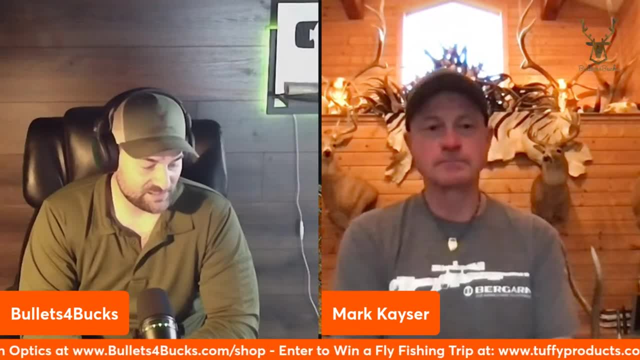 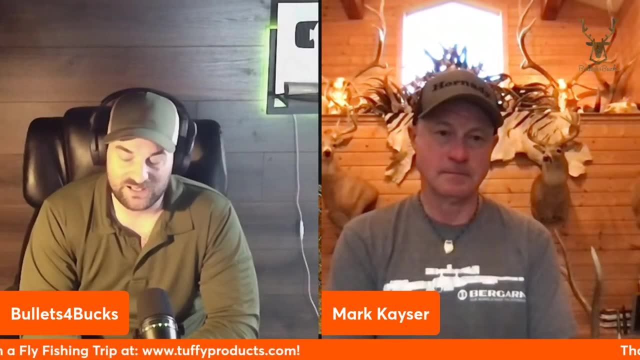 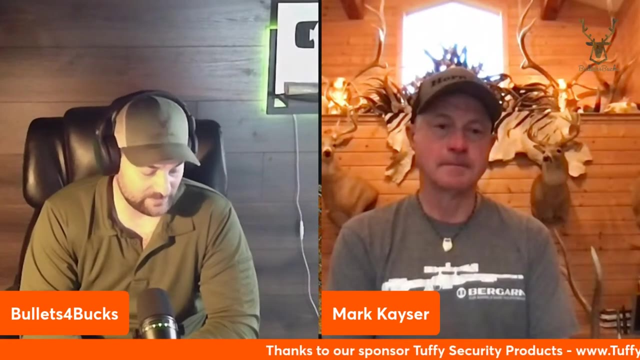 but i drew a pretty good unit for our area and, uh, you know, it might for a lot of people might be a lifetime thing from a non-resident standpoint. and he was a non-resident and he just super nice guy. nothing, uh, nothing against him, right like he's, it's. uh, i don't want to speak bad of him, but 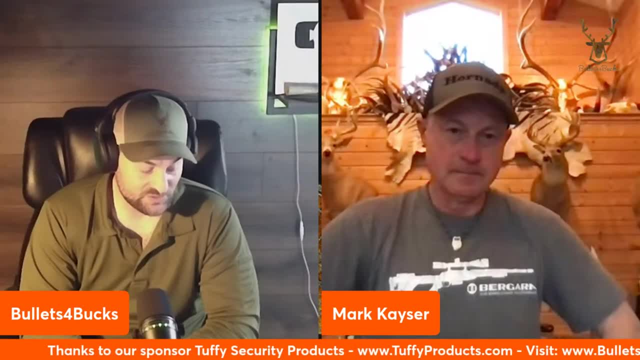 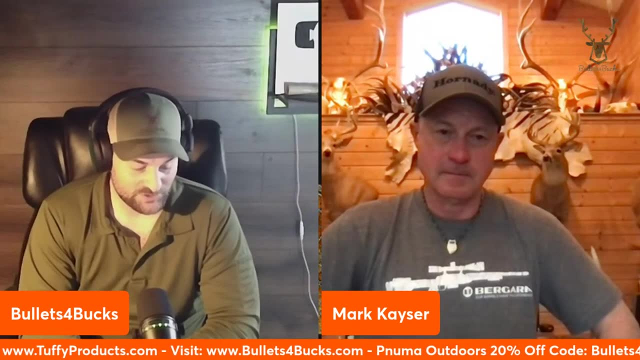 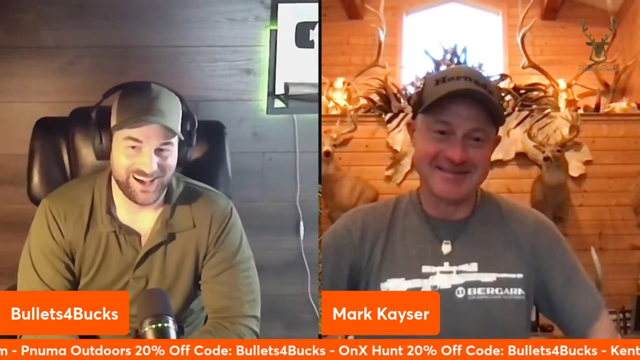 he, his, uh, the first snowstorm. we had a good snowstorm come through early season and he, he was camped near me and i woke up to a tarp and trash laying on the ground and i mean, he, i cleaned up some of his stuff and i really i don't even hold it against him, but man he was. 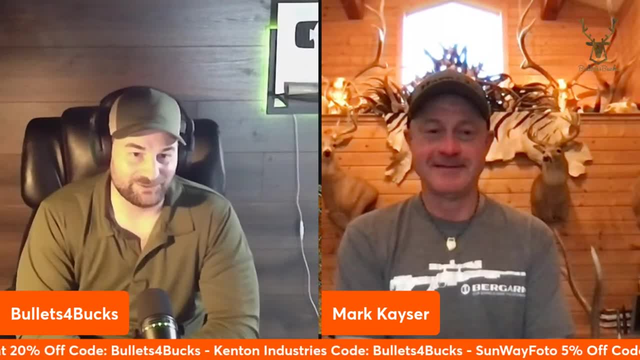 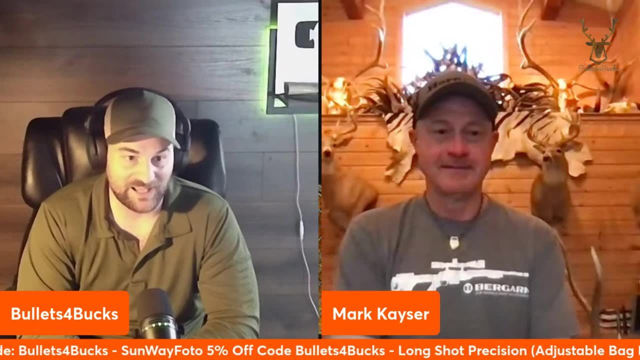 like scared, because he talked to me the day before when it started and it was like he didn't have any of the right gear. he wasn't prepared and he just like fled for his life and i think he hunted one day on a tag that probably took him. you know, i don't know, but we'll say 10 preference points. i. 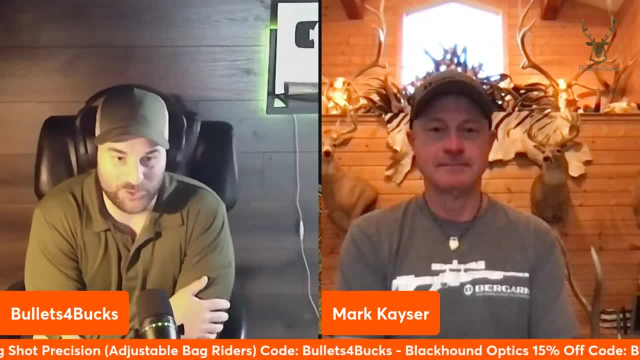 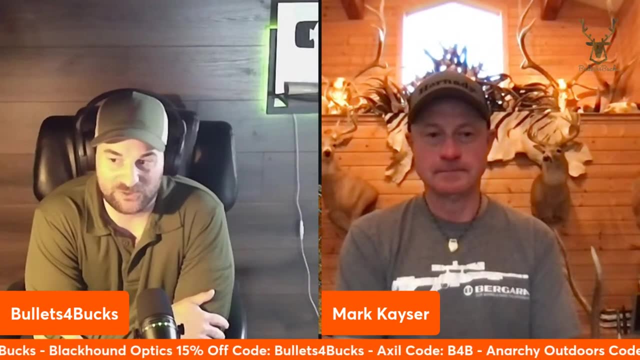 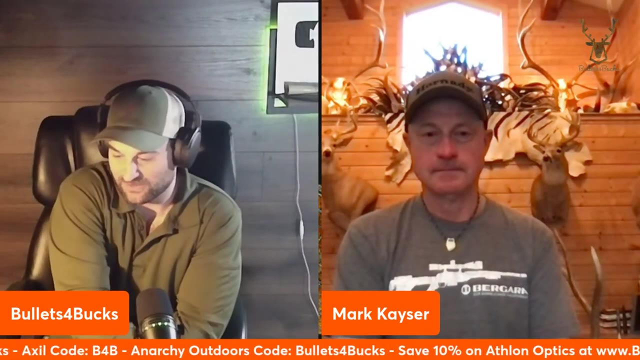 don't know exactly, but you know a decent amount and so it's like man, you, if you got that uh kind, or you know it's a once-in-a-lifetime tag potentially- you definitely don't want to have that happen to you, so being well prepared is super important. um, looks like steve. go ahead, go. 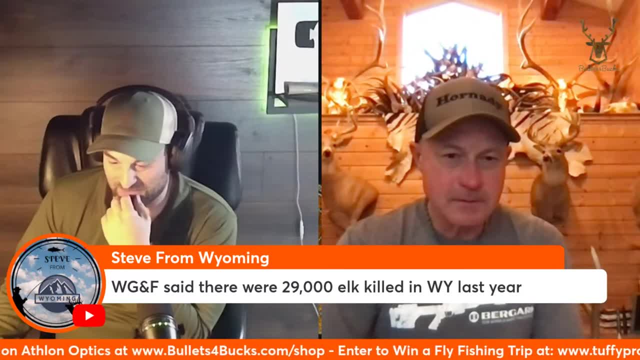 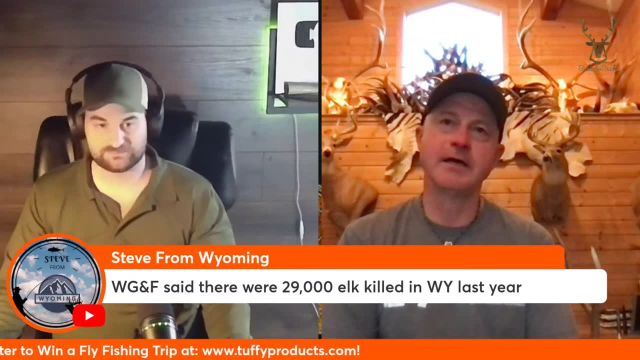 ahead. oh, i was just saying you said, uh, wyoming game fish said there was 29 000 elk killed last year in wyoming. i don't know what the normal number is, though, so i don't actually know. honestly, i don't either. i, uh, i know some of the success rates, you know, and they really vary unit to unit. 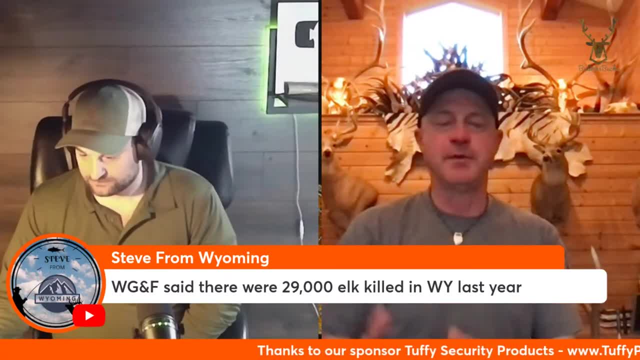 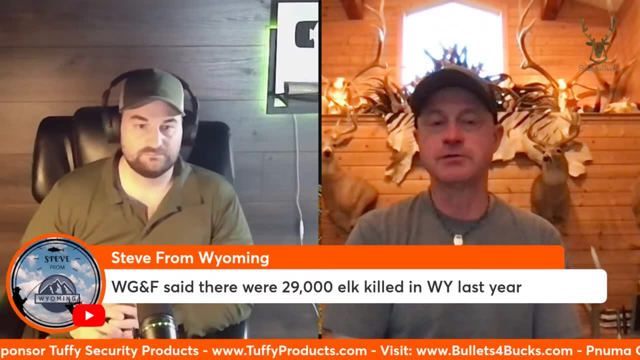 depending on the private land, the outfitted. uh, how much public land there is there. but, um, like one of the units- general units- i hunt here never posts a success rate in archery season over, uh, 15 percent. uh, it's usually 11, 12, 13 percent. 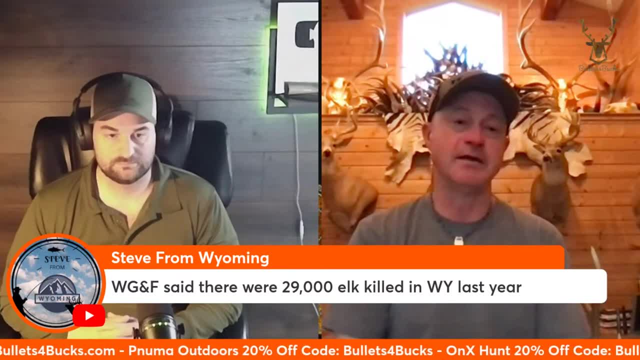 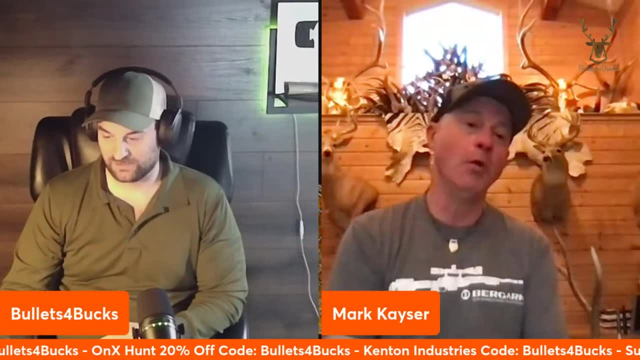 and it's same with another unit, a general unit in montana. so 29 000 elk, that's, that's a lot of elk and i hope we can kill more someday. i mean, i hear all this, well, i hear all this griping. these land owners are like. 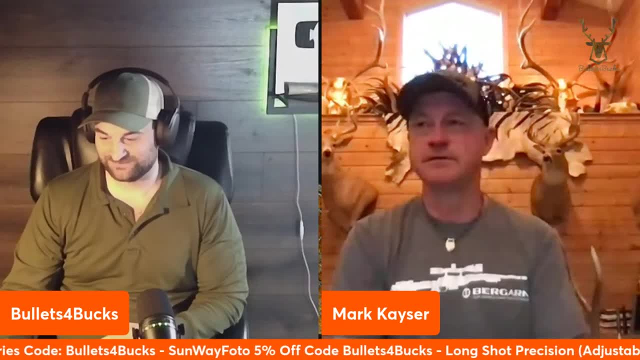 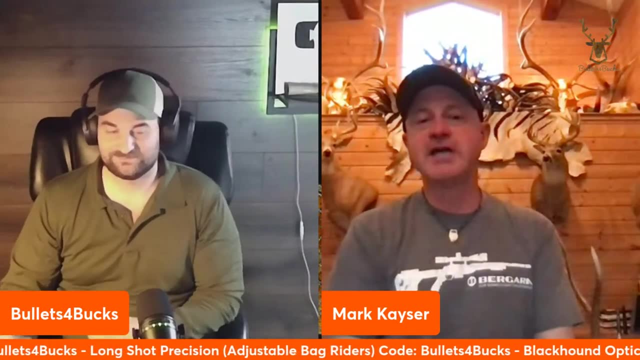 oh, we got too many elk, especially in the southeast, and that was a big part of the legislature this year. and and then they want all these special, you know, treatment stuff, which i understand it. they're eating grass, but the system's in place already. you and i and the rest of the people. 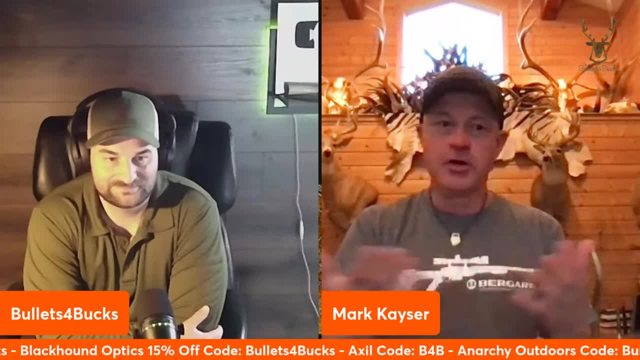 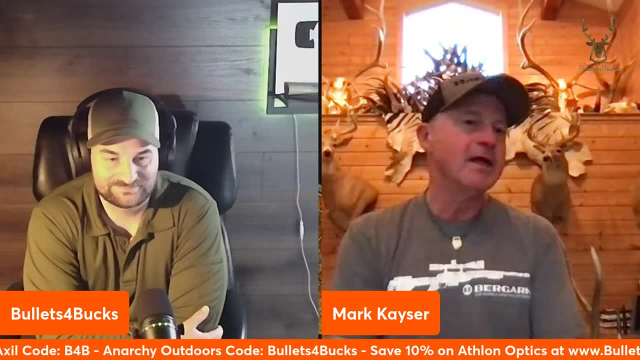 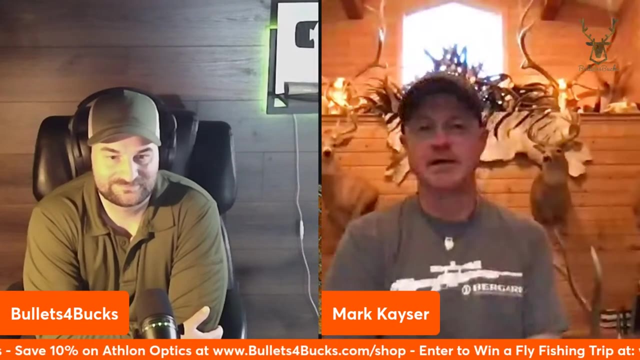 watching. we'll kill those elk- and elk are great meat. i mean, it's a, it's just a great protein to put in your freezer for the family- and we just got to find an easier way to get the public to be able to kill all those elk that are hoarded up on these, uh, private ranches. 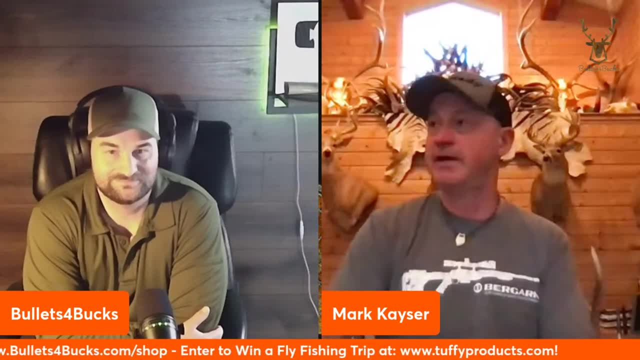 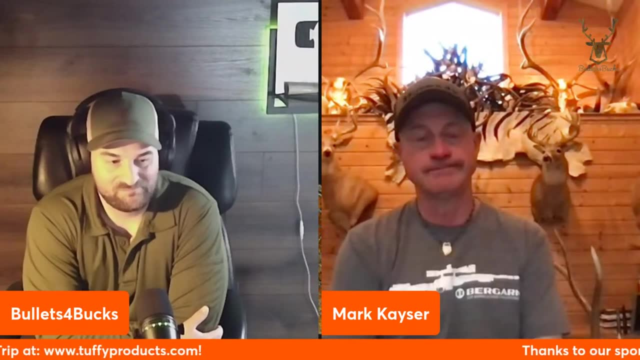 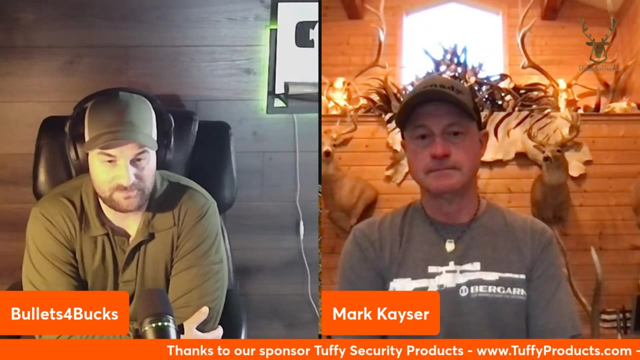 that come late in the year and that's a big problem. that's a huge problem. it happens, you know, right out my front door you know, yeah, yeah, so, and don't they get, or i don't know, i don't they get subsidies, or um, what do they call it? if they damage property, don't they get money from the? 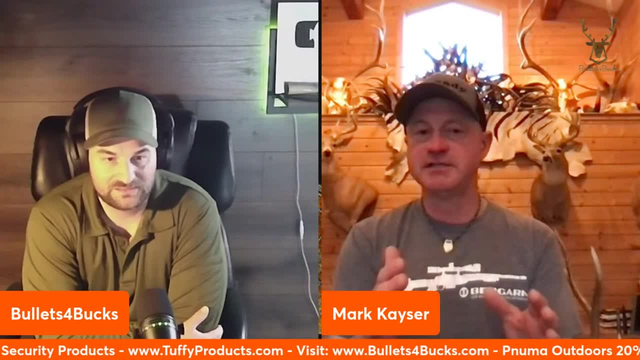 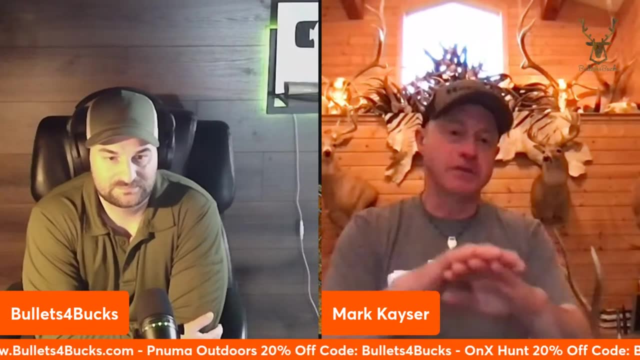 government. no, they do get some, but that was part of the legislature and they don't get money from the legislature. this year they wanted bigger payments for elk graze because the elk were grazing like cattle, so they're eating pasture lands. and again, i understand all that. you know, we're all in this. 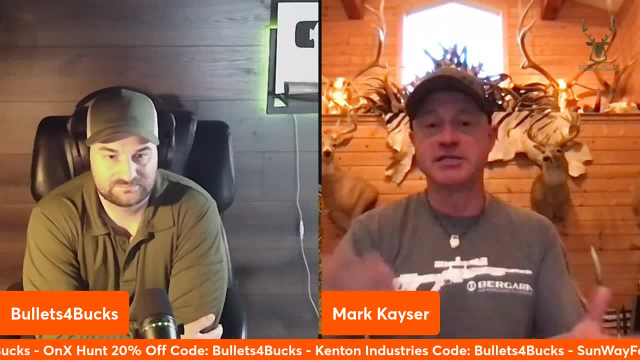 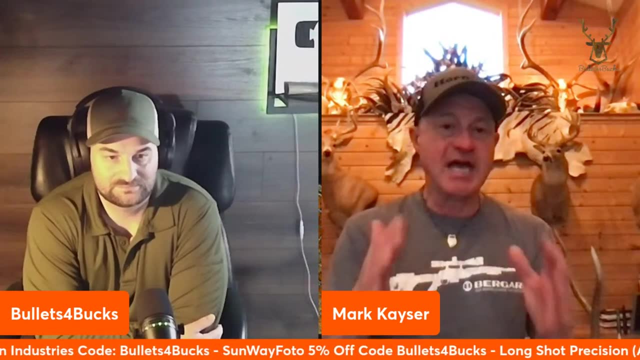 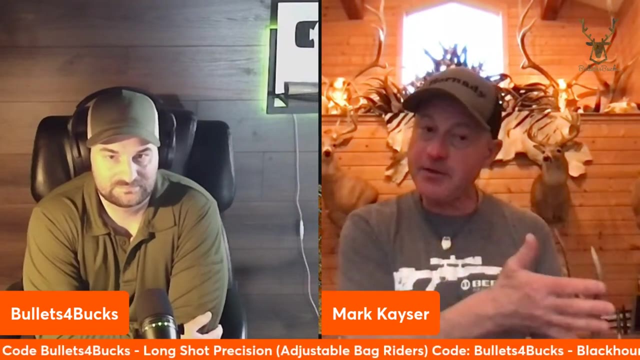 world at this point to make a living, you know, whether you're ranching, writing, running a podcast, like whatever, you know it's all. it's all a money, a dollar deal. but at the same time, elk are owned by the public. we own them. you know. they're not privately owned. the land they're on is. 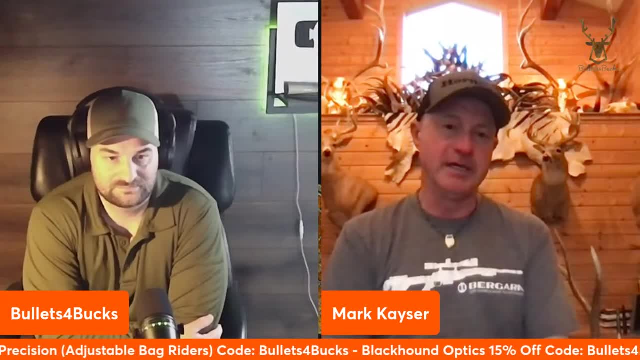 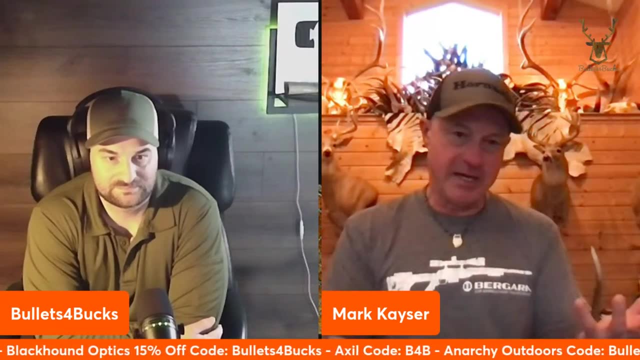 owned, but there's more than enough people willing to go in and shoot those out. and if there's some system- and i know you know there's bad apples in every group- some bad hunters give us what's a bad name, just like you know people that are robbing convenience stores give. 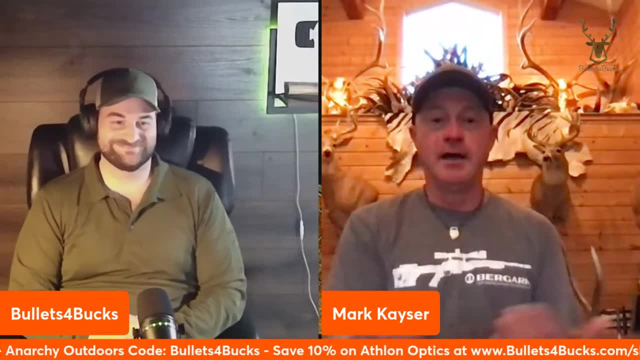 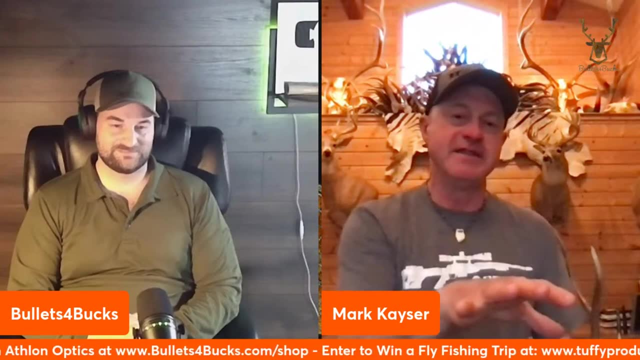 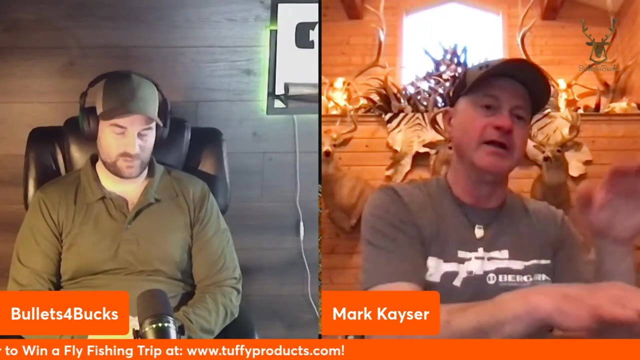 me a bad name and i go fill up my truck there. but uh, but there's got to be some way we can work together. and if you put enough pressure on the elk, you know one day they won't stay there the whole winter, they'll move on. then they'll move on, and they'll move on. and little groups. 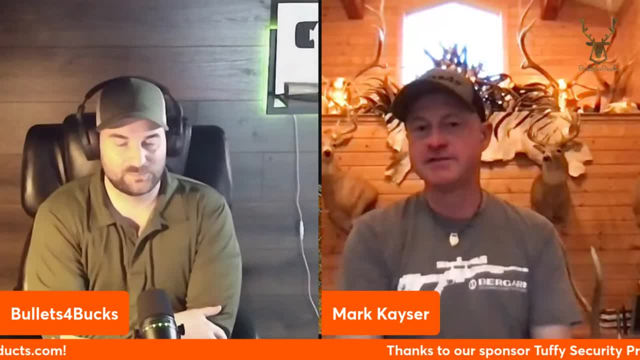 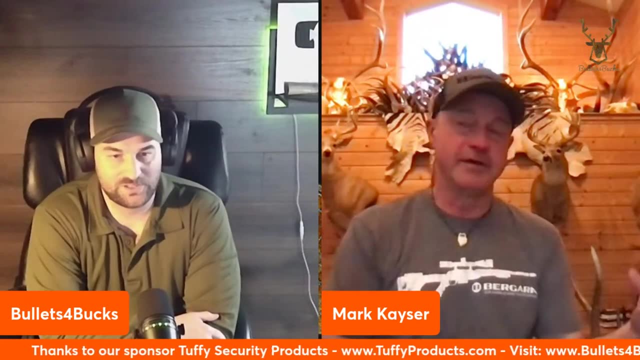 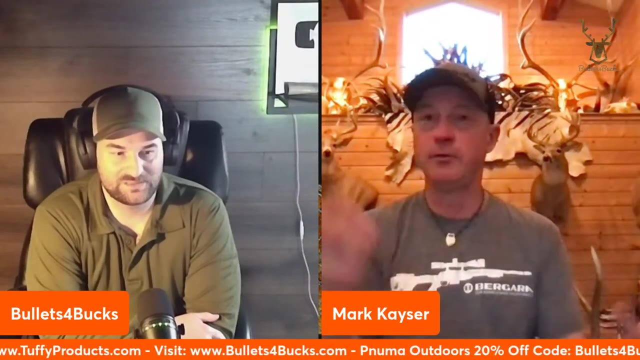 of hunters can be picking off those cows, the antlers right elk all winter and it can go out all winter long. why, i don't know, why i can't you know, it's where the game warden's out, you know, trying to manage it. but uh, is there a reason not to elk up until almost this point? uh, you know. 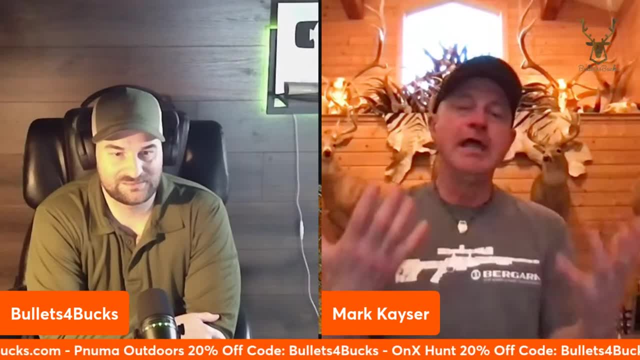 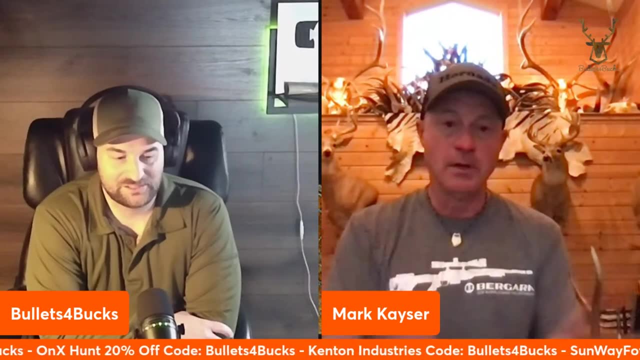 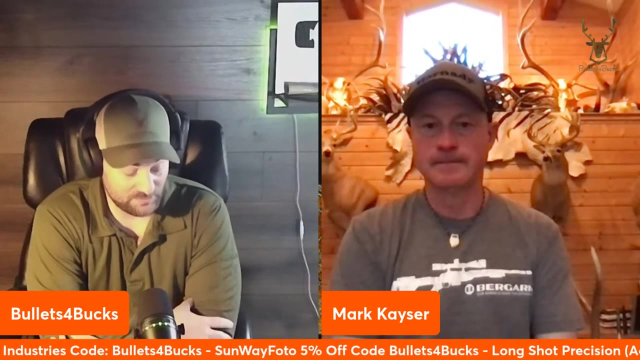 because we've got so many. there are almost, almost in every elk unit in wyomington. they're at an objective or over. i mean it weighs over in some instances. so yeah, there's, there's got to be a solution. i mean not only for landlocked land, landlocked public land, which that's a whole. 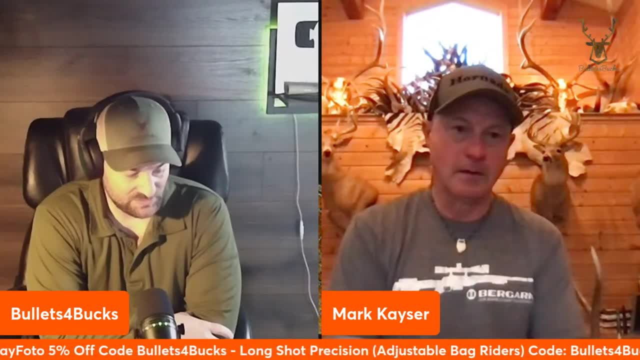 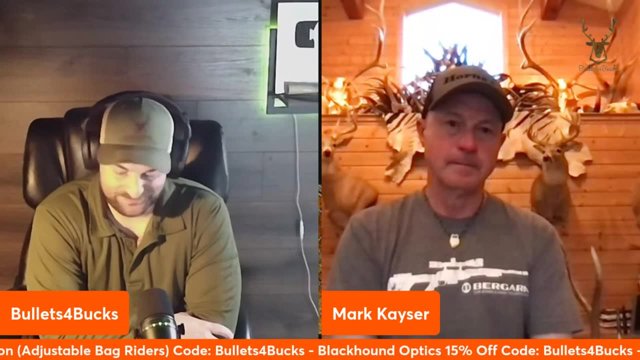 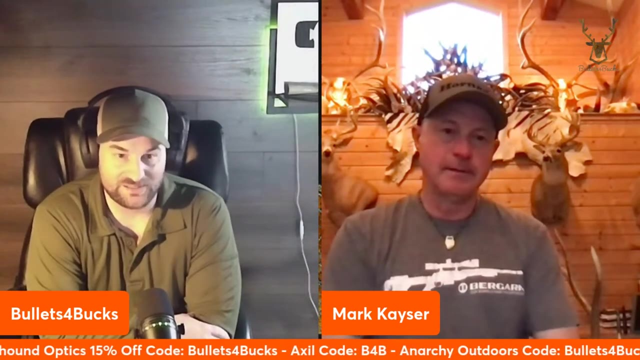 nother can of worms, and and the, you know the destruction of ranching land by, by a wild game. it's just, you know, i guess, finding a way for us all to work together, ranchers and, and, you know, non-ranchers alike, and and and if it, yeah, of course there's bad apples. that's the hard part. 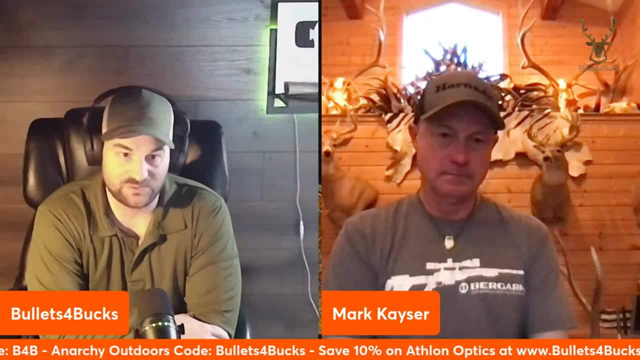 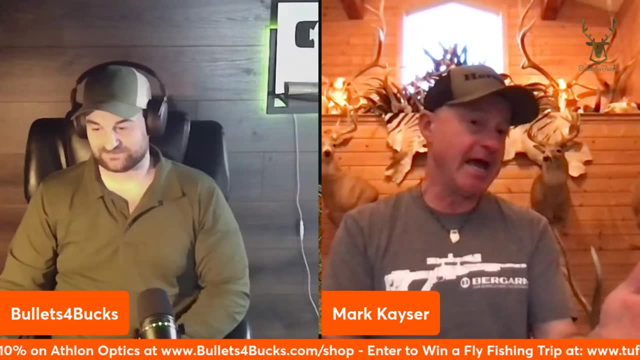 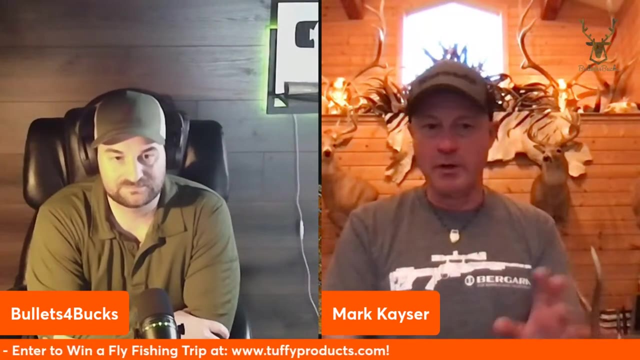 and that's the part that always makes people, i guess, embittered to um that, and probably money, but uh, but if, yeah, if you're in at least your private land out to an outfitter, then that, then that erases it in my mind. it's like that's, that's not an issue anymore, you know. 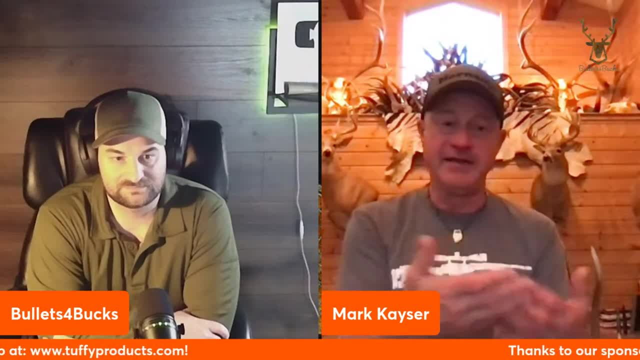 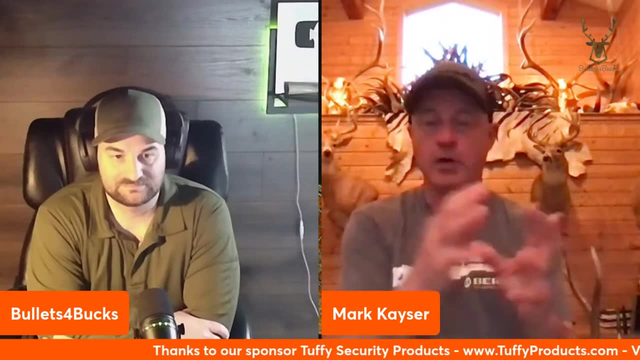 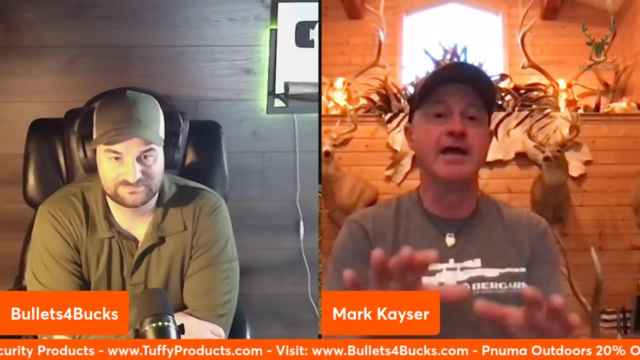 because they're not letting people on during the regular hunting season, and then the outfitter probably don't want people in there after the season because he wants it to be a little sanctuary all year round. so they'll always say that. so there's- i mean, there's a lot. there's just- yeah, there's just so many moving parts to this. but again, 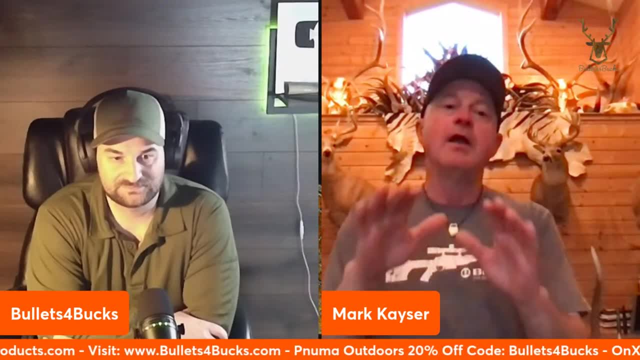 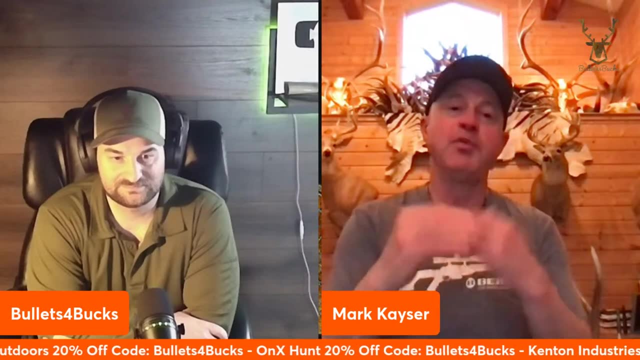 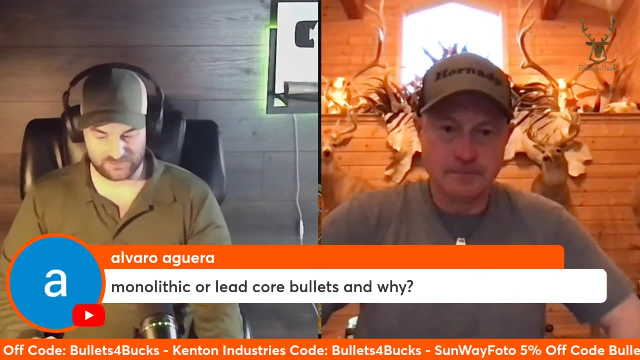 wildlife is publicly owned game and fish has a plan in place to manage wildlife. we just got to get that plan working better than what it is right now. interesting. here's a question, and i don't know if you, if you don't have an answer, just you know. 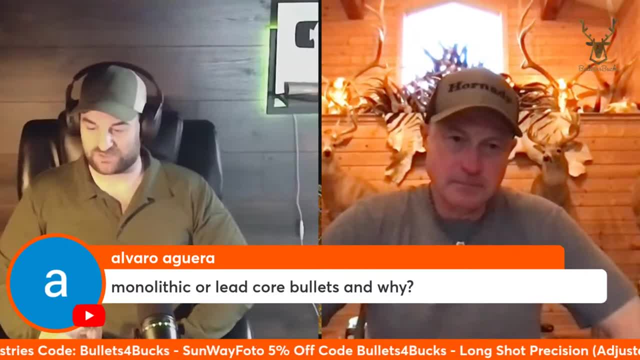 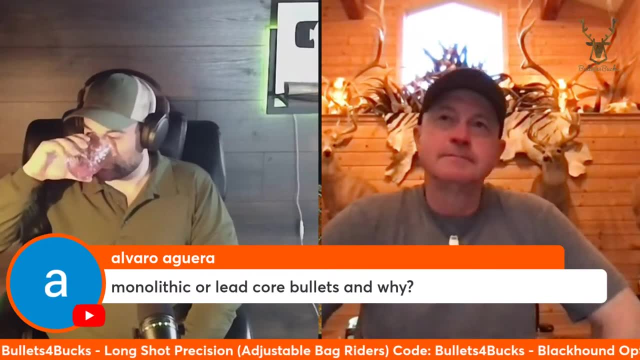 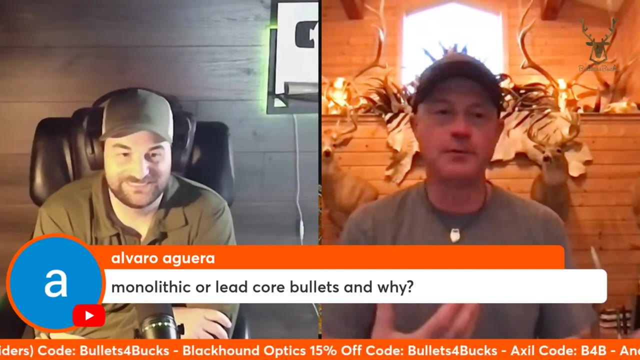 say i don't have an answer, but uh, monolithic versus lead core bullets and why. somebody wants to know here, i can assume, for hunting, um, i don't know if i feel good answering that because i've used both. i've used almost every type of bullet out there. so in fact i shot my last uh elk with a. 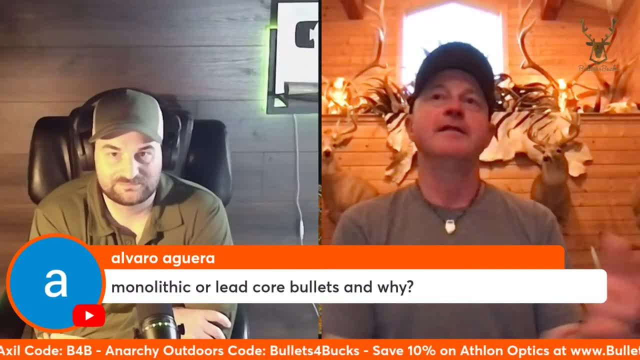 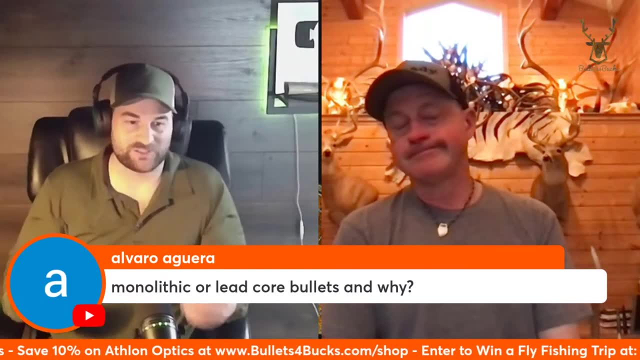 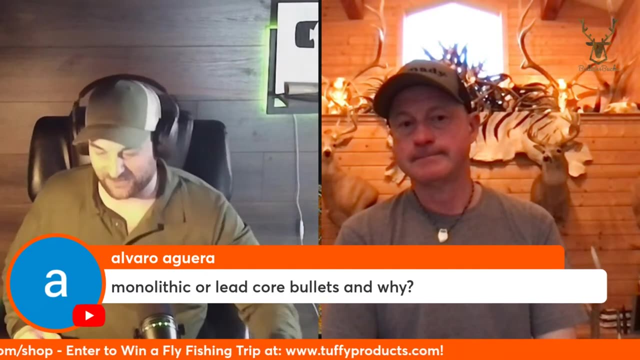 no, not this one, the one before the monolithic bullet and this past elk. again, i went back to lead core just testing a new uh bullet round. so, uh, well, i use lead, i use lead core. so i mean, and i don't you know, i'm not worried about offending people, so i guess i, i, i don't see. 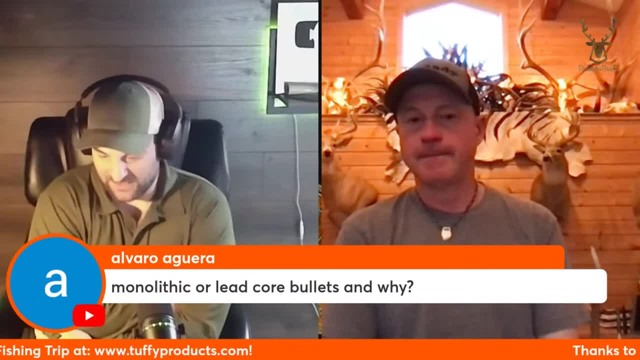 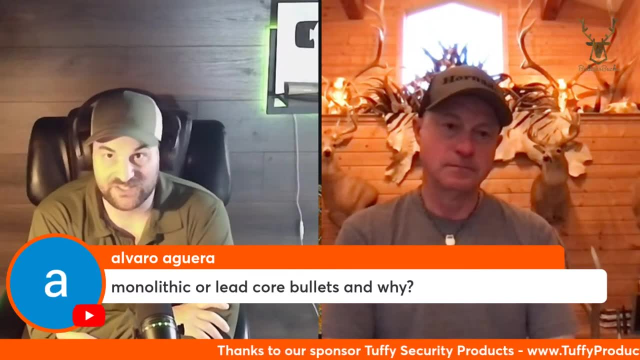 anything wrong with either one. obviously there's environmentalists are more into the monolithic because they're usually solid copper from my but uh and i know in alaska all my hunting buddies in alaska have gone. almost all of them are going monolithic because of grizzly bears, i guess they. 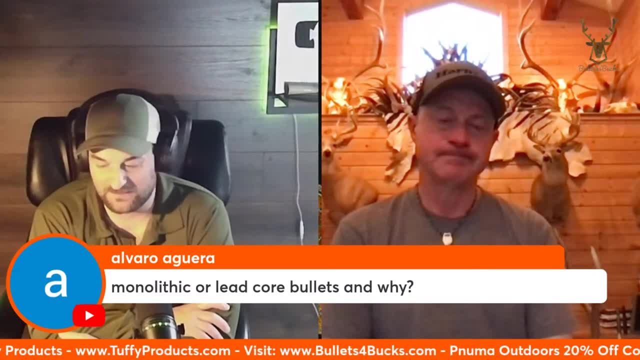 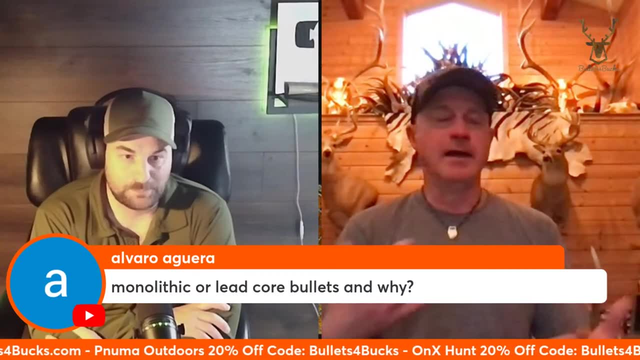 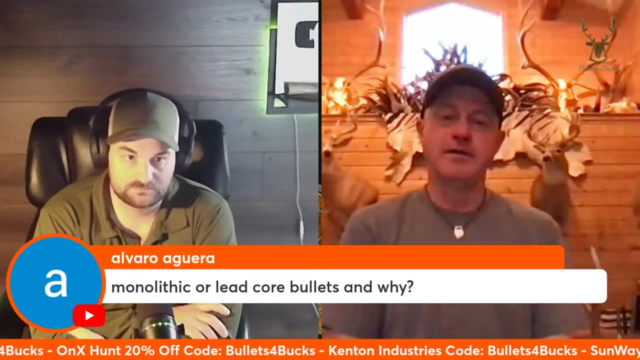 they want better penetration, but that's um. you know, they don't want that bullet to fragment or fall apart or you know whatnot, hold better on a grizzly bear. you know, in certain situations like that, grizzly bears, cape, buffalo, moose and even elk- uh, there are reasons for a bullet to stay together better and not splinter. 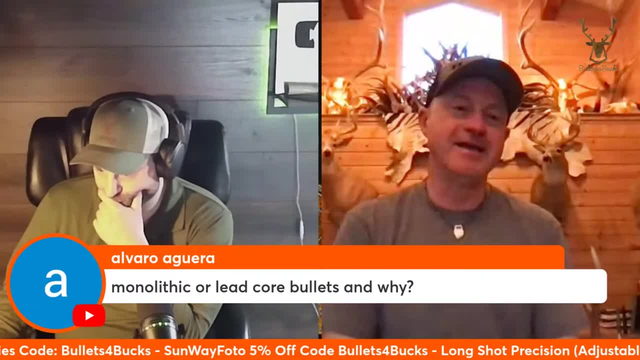 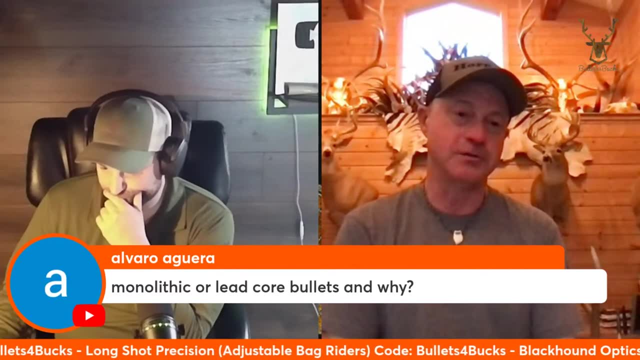 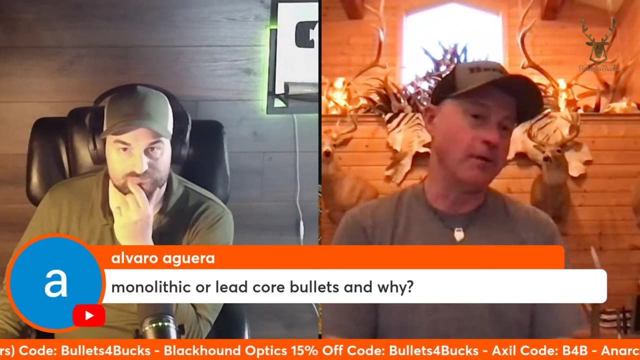 obviously, and mushroom. but what i've found over years of hunting, again it so much of it comes down to shot placement and making sure that shot is true. and even when you feel like you've got the best shot opportunity, you know things can still go wrong. so, uh, whether it's going to be the bullet or just the animal moved, uh, you know. 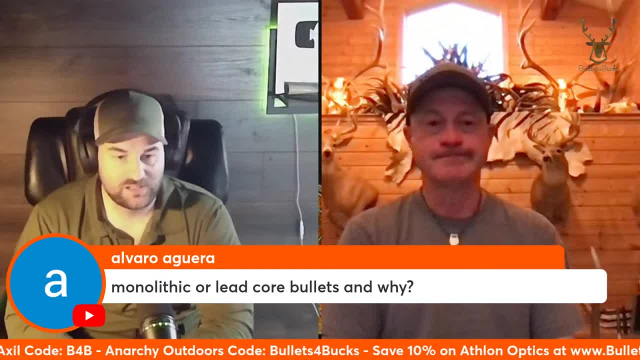 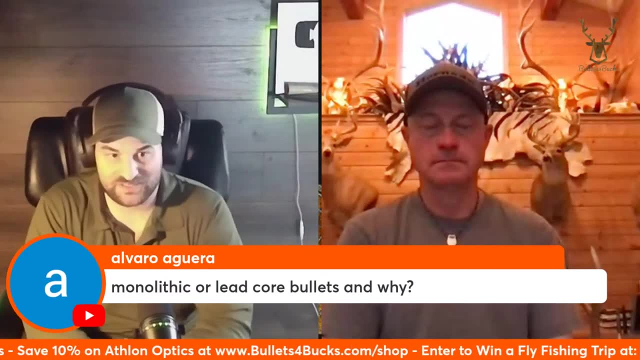 sometimes things can't be helped. but yeah, what's your? uh, these, these, like my channel is more of a gun channel, i guess, but i'm actually not as big into ballistics myself, i'm more in just like bolt action, rifle construction, um, and how they perform. 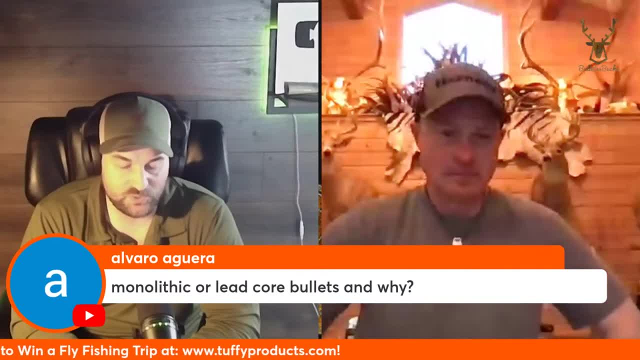 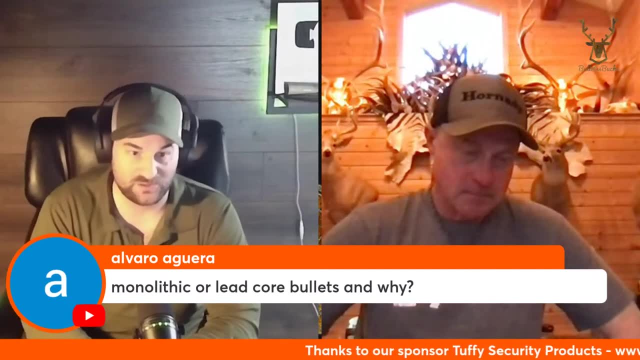 but what, um, i guess what's your current favorite hunting rifle? or and and down to like the model. do you have a model you really like or you're going to use this year that you are really looking forward to using? well, the one i used last year, i'm waiting on a new one, but i don't know if. 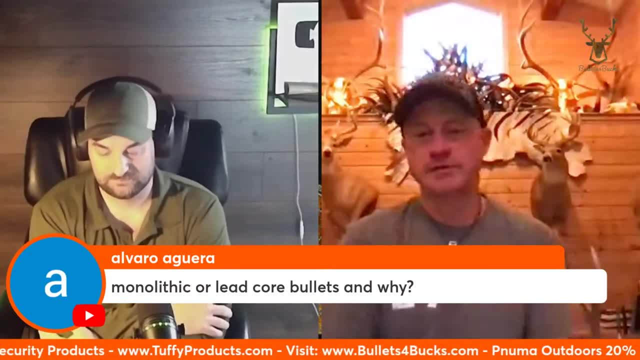 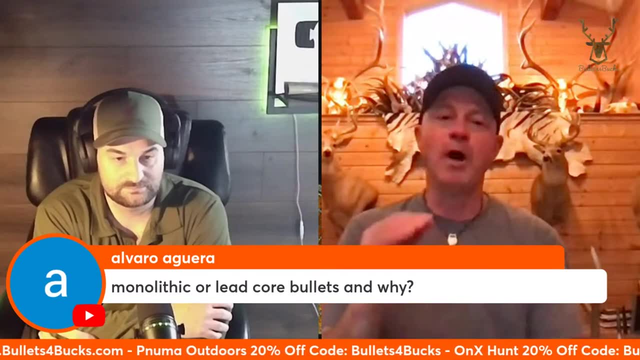 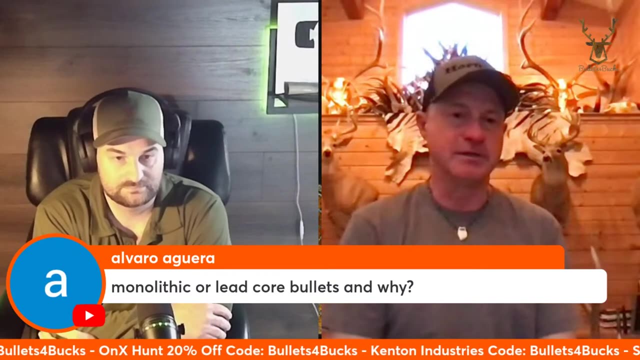 it's going to show up, so let's just put it that way. the one i used last year was the bergara carbon ridge and, uh, with the cure barrel it weighed 6.6 pounds. i wanted to get it in the 7 prc uh, but just because of some manufacturing, i, i, i just couldn't get that caliber, so i went with the. 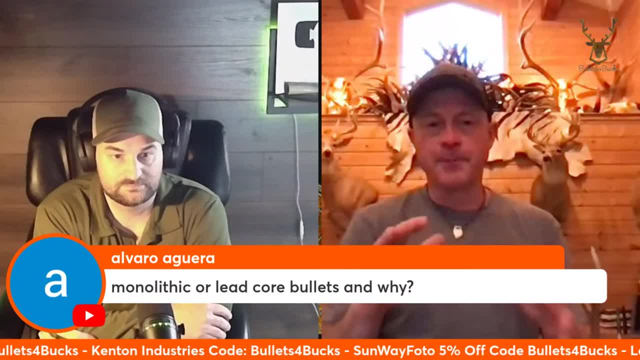 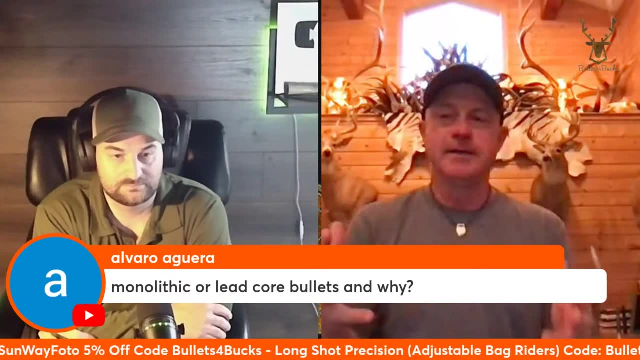 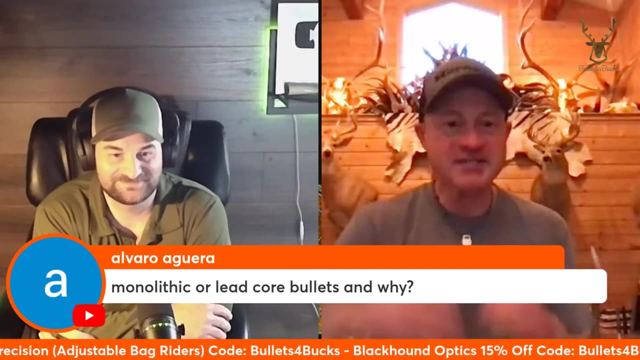 300 win magnum, that that caliber sounds big but i use it almost for everything and and i the reason i do is i feel like, uh well, i, i like teddy roosevelt carry a big stick. i like that saying for one thing, but i start out with l, usually in the back country, and then you're using that rifle. 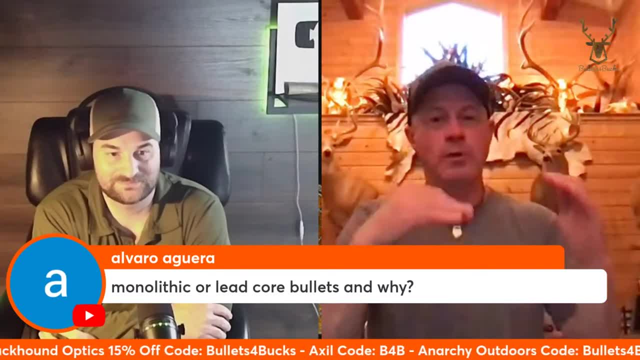 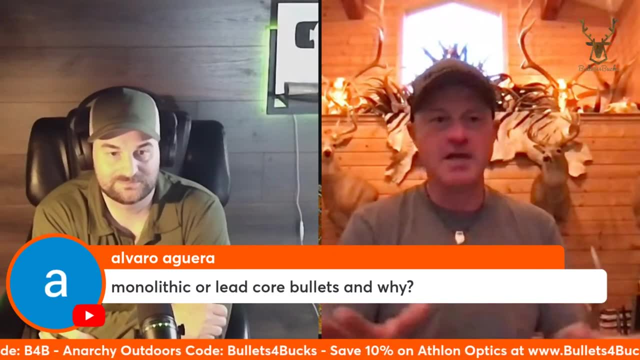 and i just, i just get a feel for it's the same thing. i just get a feel for it. it's the same thing with a bow. once i set my bow up, i use the same bow. whether it's for elk, antelope, white tail, i don't change anything. it's just because i, i just like to have that it's, you know, almost mated with. 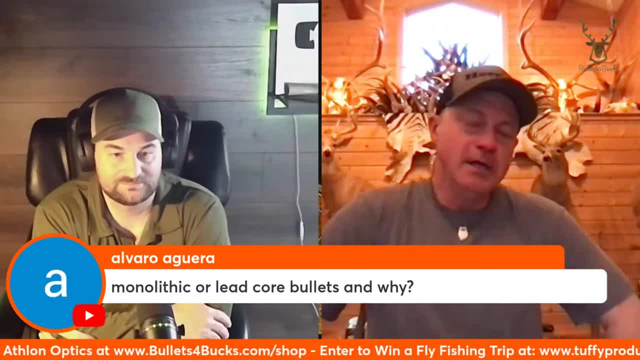 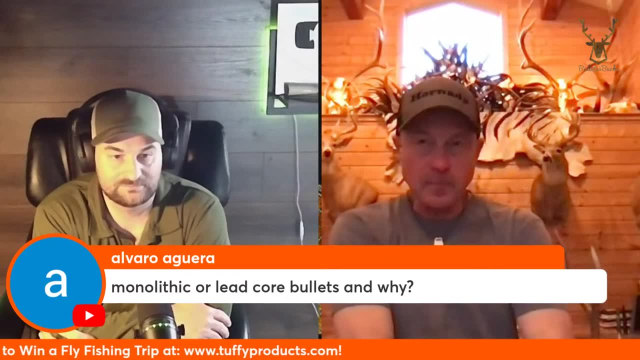 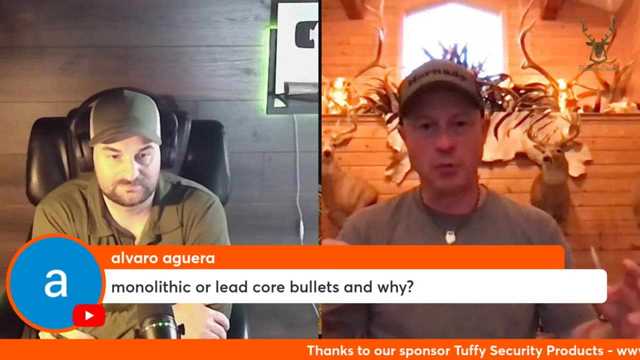 it. so that's the rifle i'm using. i had a sierra uh six hour sierra six rifle scope on that in an um a four to eighteen configuration for power and a four, four objective, just to keep the weight down again. and i have been, even though it seems odd, you know i'm trying to keep. 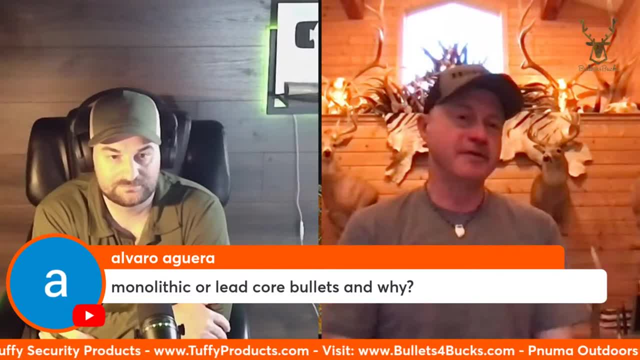 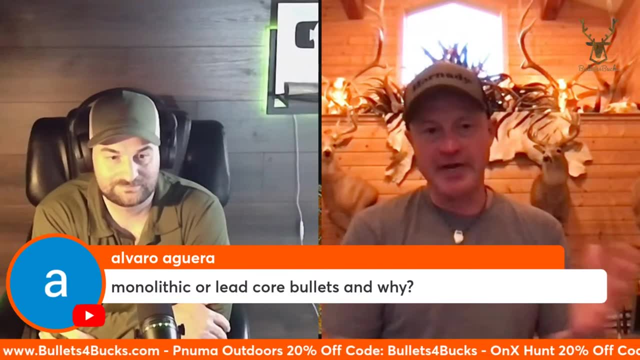 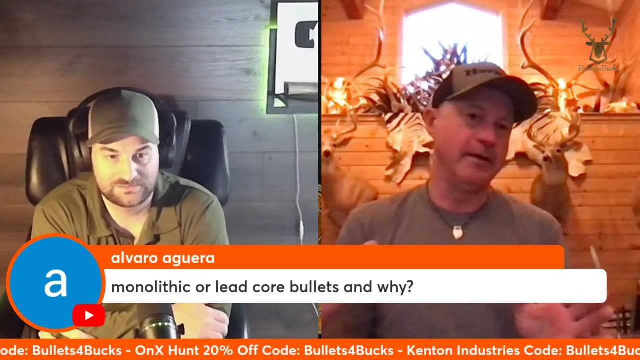 that gun on a nutrisystem diet. i do slap a suppressor on it, usually a silencer central, and i'm waiting for my back country, but i got a banished 338 as a suppressor i've been using. i really like i love. i love a suppressor for everything now and yeah and uh and it's getting. 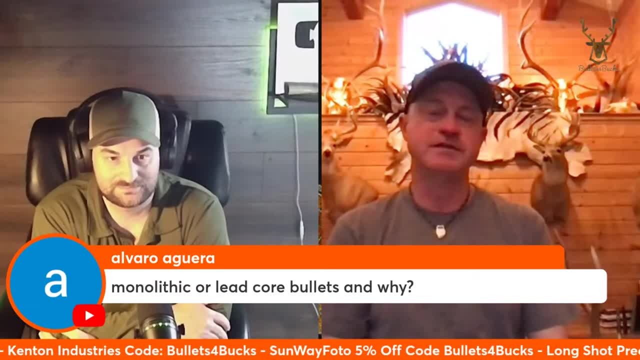 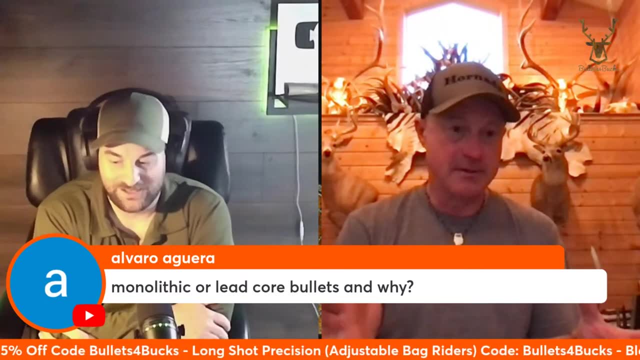 easier to get. i'll use a company like silencer central. obviously it's easy, they watch you through the steps, but i know the atf has reduced some of the time. now again i heard somebody got. i heard somebody got one in 48 hours, approved something. 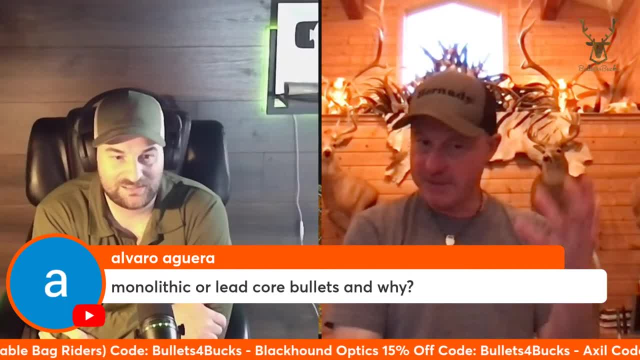 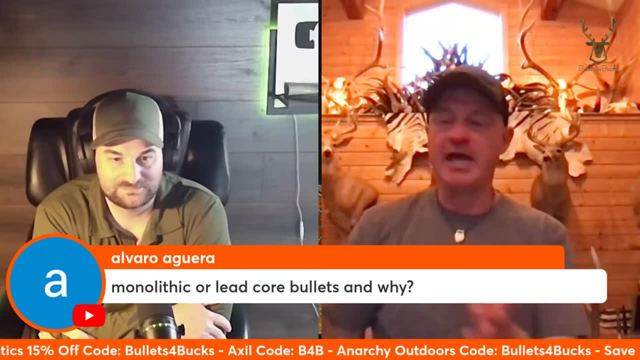 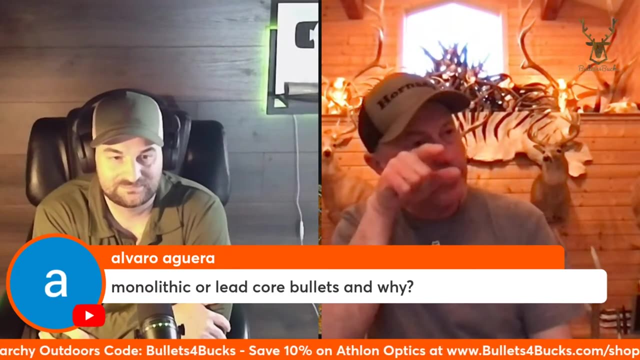 crazy like that it's. it's, yeah, i've heard the same thing. so, uh, but a suppressor- one of the reasons i like a suppressor- quiet, obviously, and when we're filming i can talk to my cameraman, not have, you know, hearing protection in. but the other thing is this year when i i was laying 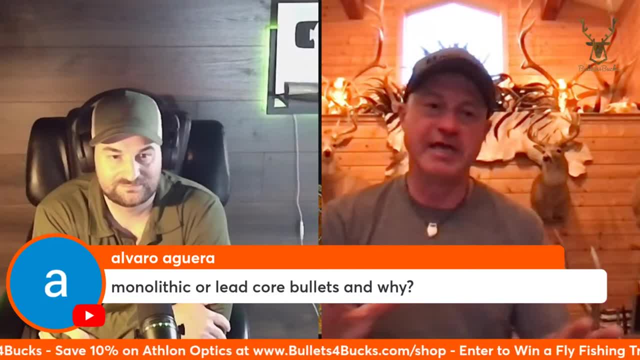 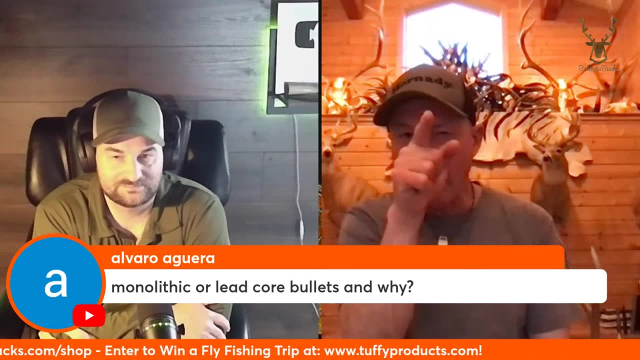 in the air. i was laying in the air and i was laying in the air and i was laying in the air and that bull stepped out and he only gave me- i mean, he really only gave me- two, three seconds to get the shot off. but when i pressed the trigger, looking through the rifle scope, i watched that. 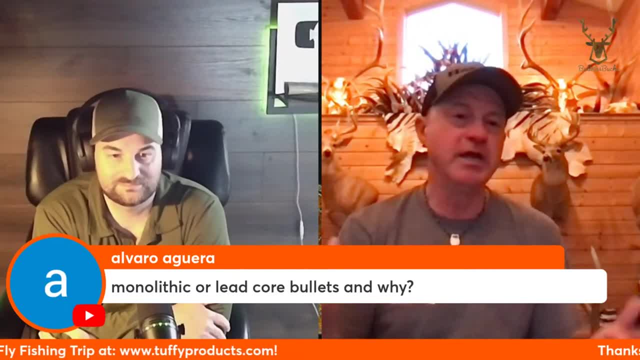 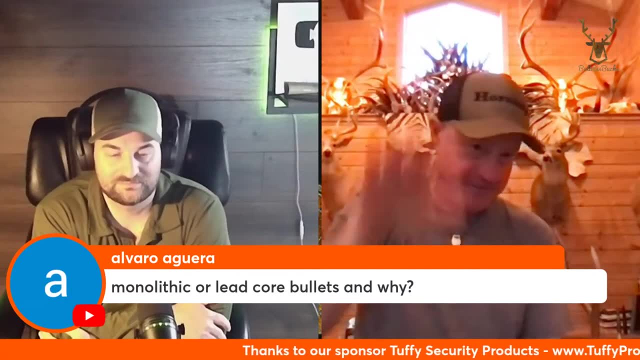 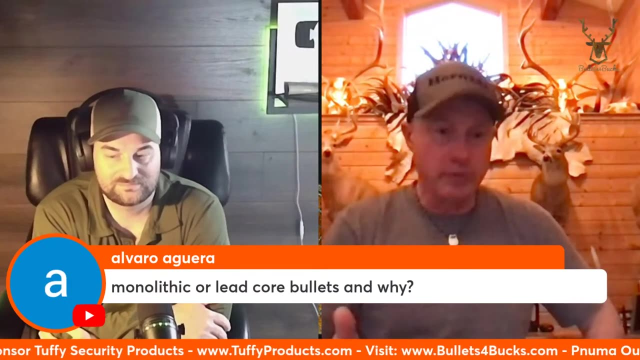 bull tip over. i knew i'd hit him, and with a 300 win mag, even with a break on it. but without a you know suppressor you're gonna lose that sight vision and you know you're gonna be able to see that. and i i boosted my confidence right there that that elk was down because it was a. 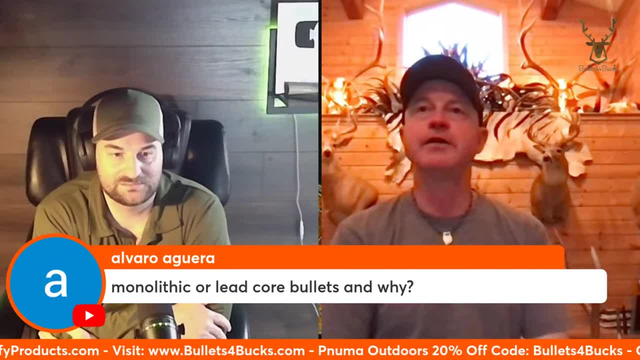 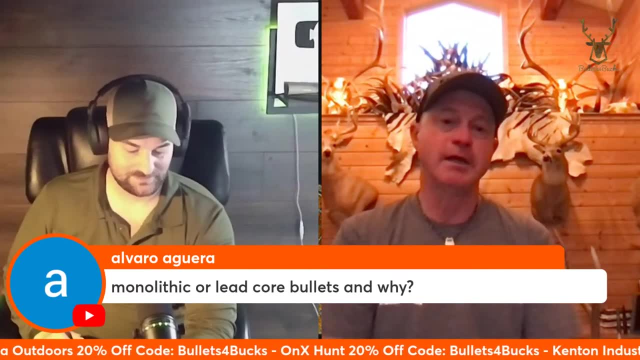 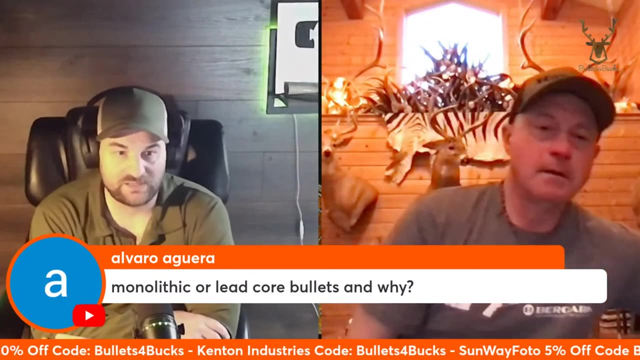 thick timber. he just walked through a little opening and then down into some timber. so lots of reasons to use suppressor today. um, yeah, i got one on that. i got one for the first time, the like november the year before last, and uh is when i finally got one, and i you know once you go. 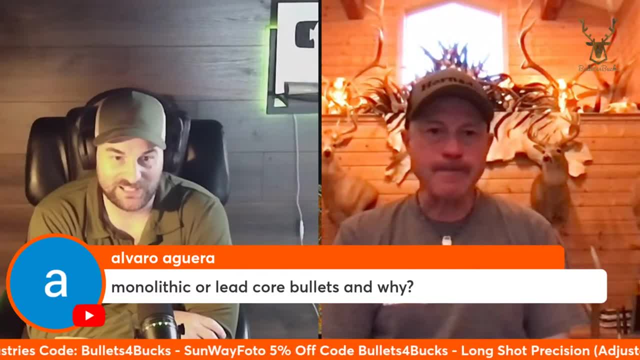 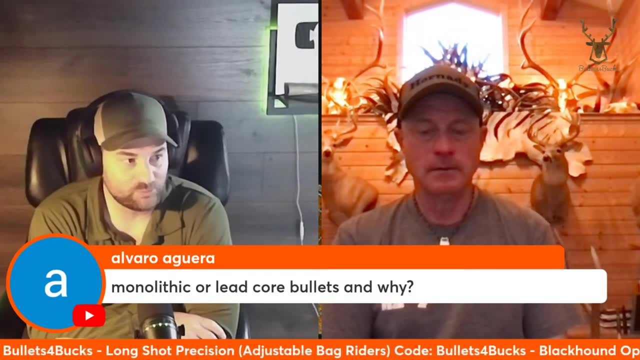 suppressor, you never go back, i guess because for hunting anyways, because i mean just so many benefits. and then, ironically, that october, right after that, i got one and i was like, oh my god, i got one. and i was like, oh my god, i got one. and i was like, oh my god, i got one. and i was like, oh my. 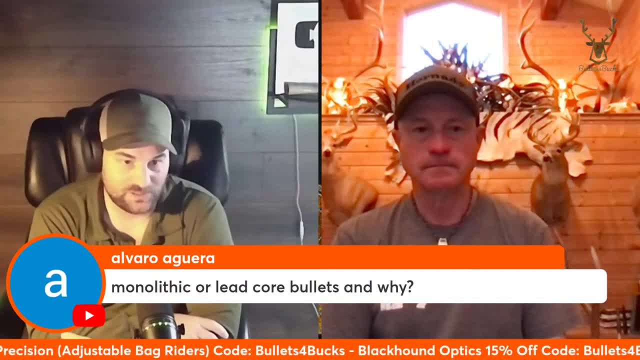 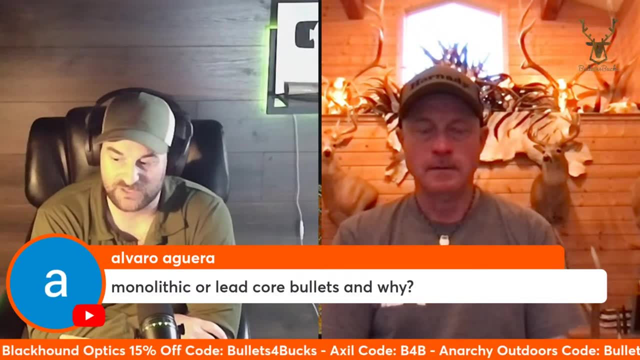 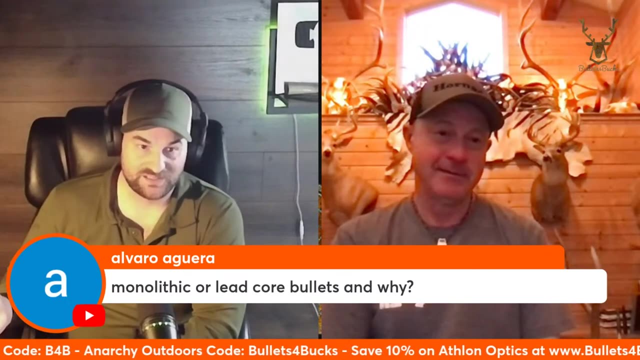 before it came in the. you know it came to the ffl or whatever. i it's embarrassing, but i took six shots without hearing protection with a muzzle brake, 65 rpm, and my right ear has probably never been the same and i mean i've, but i i always hunted unsuppressed, without hearing protection. 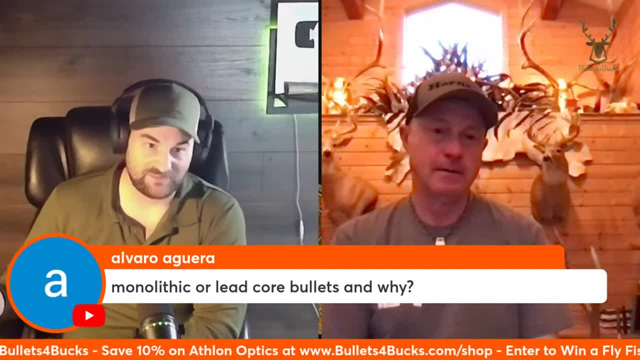 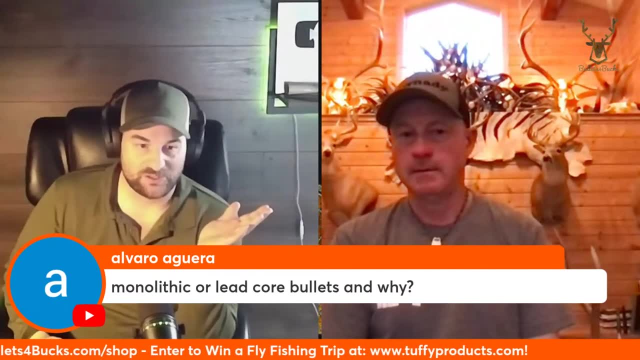 um, and then normally not that many shots with a muzzle brake though, but that was like the icing on top. and then the next month i got the suppressor, and i was like man, for one thing i should have worse hearing protection, but for another i mean a suppressor, just because me. i'll be honest, like 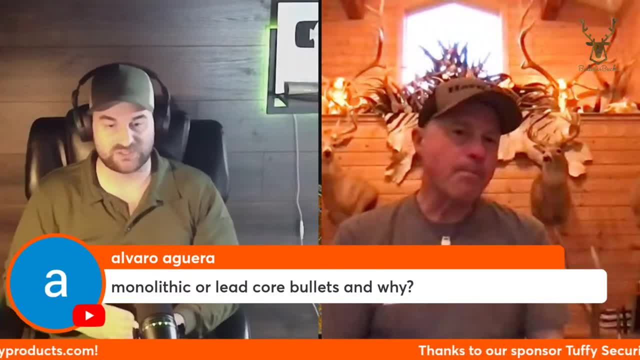 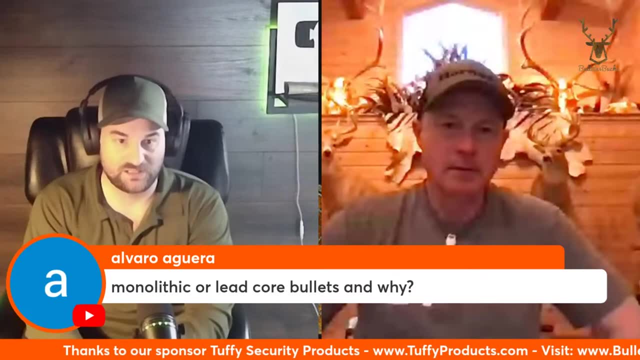 unless i'm using something that's passive, in a earbud style, i'm going to forget to put hearing protection on a hundred percent, a hundred percent of the time, like i'm just always going to forget, because i get in the moment, um, when i'm hunting, i'm just going to forget to put it on. so, uh, now, 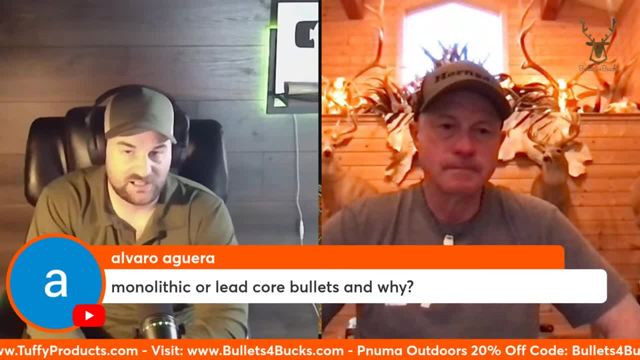 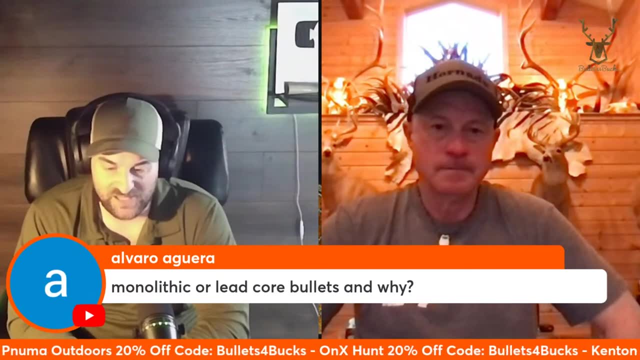 that i've gone trying to use suppressors on everything hunting just last year. it's just, you know, i don't have to, i don't have to worry about putting hearing protection on it's, on the rifle, so to speak. um, and yeah, reducing recoil and whatnot, and and arguably, if you do miss, hopefully you don't. but 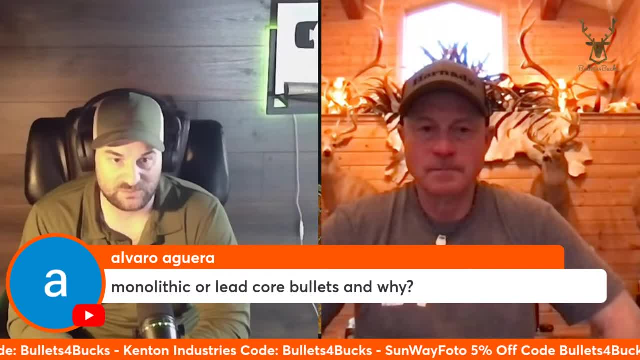 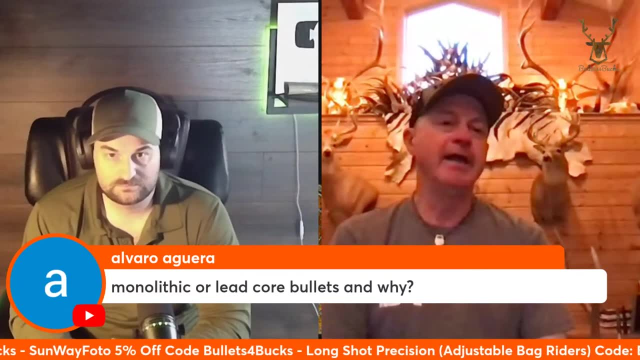 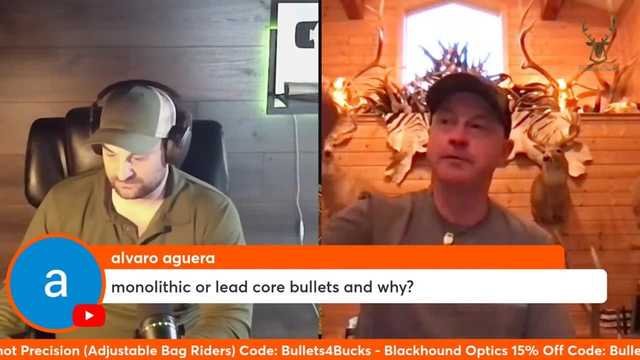 if you do. generally the animals don't really spook the same either and you might have another opportunity. um, and i have. i had an elk low two, two or three years ago and, uh, with suppressed rifle, he, let me just finish him off right there. you know, we just uh, yeah, and the other bull there. 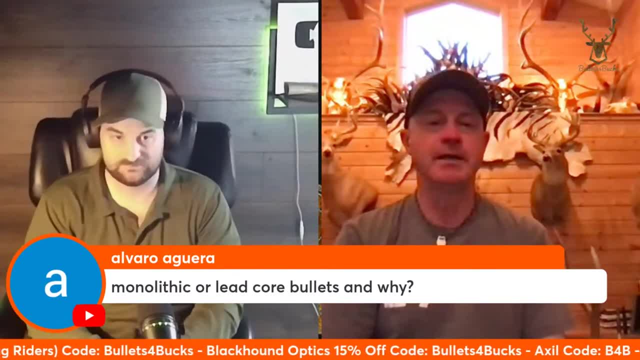 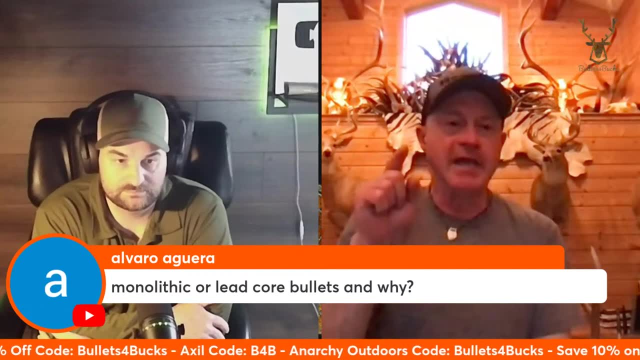 was another bull standing right above him, just stood there, never ran anything. so, and another one of the things that i like it is i i have a coyote dog i use and when i'm you and when he's with me, i don't always use him, i don't always let him go, you know, out to the coyotes or decoy or 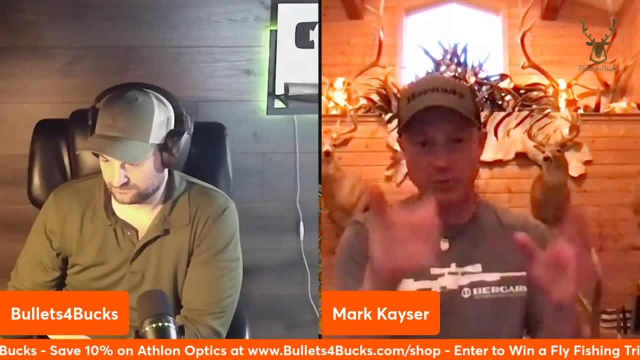 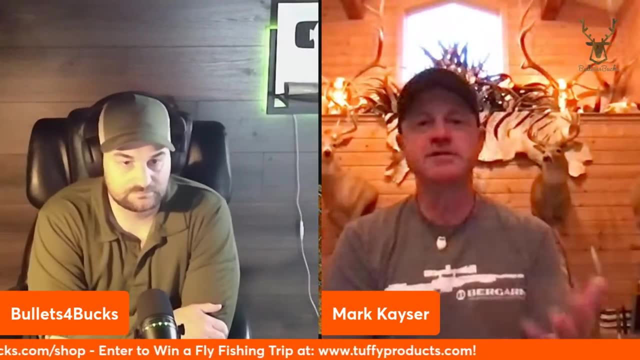 whatever, a lot of times he just sits beside me and until i read what coyote's doing and when. so when i shoot, and if he does stay beside me, uh, it's not affecting his ears. my first coyote dog, she actually went deaf. now whether that was from shooting. you know being around an unsuppressed. 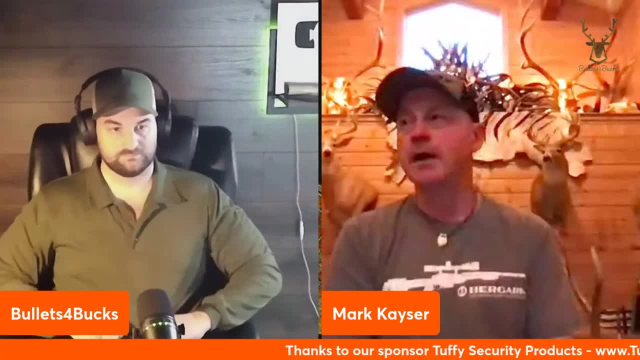 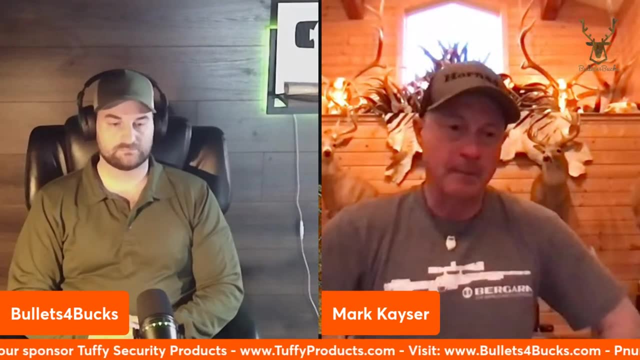 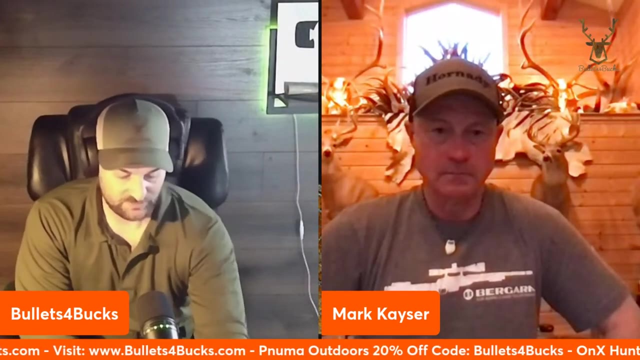 rifle, because back then i didn't have suppressed her. uh, i don't know, but that dog was right before she died. she was, she couldn't hear anything hard, and so that's interesting. yeah, i've actually never had never hunted coyotes with a, with a dog, before. that'd be that's interesting. i've seen videos of it, but uh, so so use sig scopes. 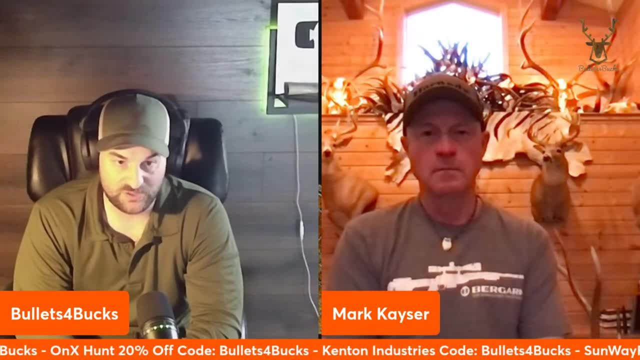 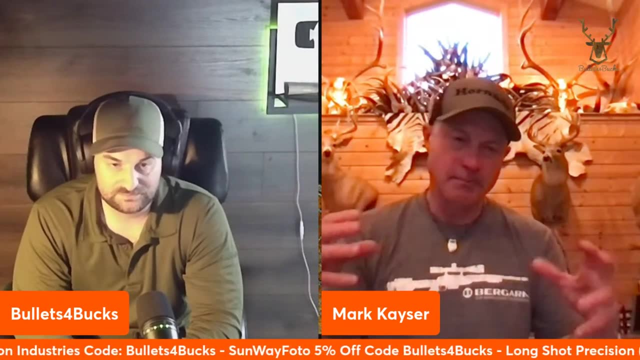 that's is that you know, do you have a special scope you're going to use for if you get this new gun? uh, in particular, i'm just kind of curious. i'm probably the same one because that's their basically the most compact one with the 18 power. 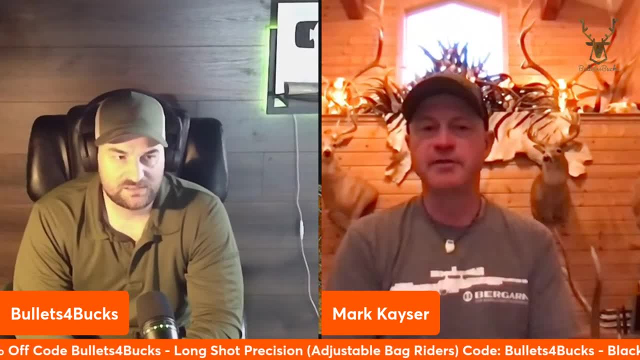 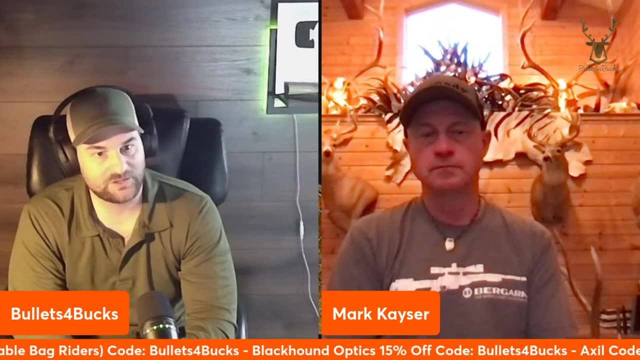 the higher magnification. so i'll probably just set it up again. on the uh, the bergarit, is that the ridge carbon wilderness? is that what they're calling it? or ridge? yeah, so it's. is it the? is it like the- uh, wilderness ridge stock, but with the carbon fiber barrel? is that the one you're talking? 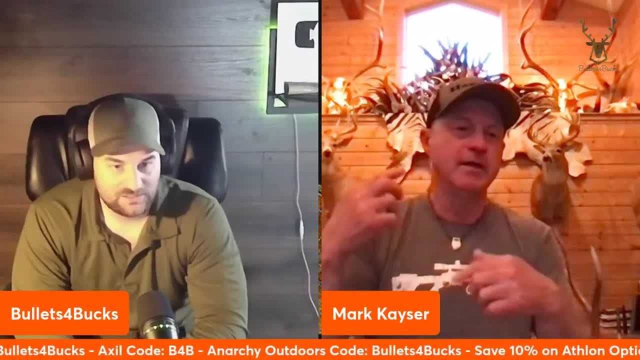 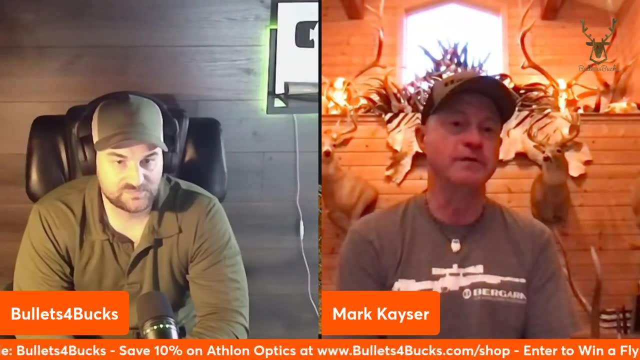 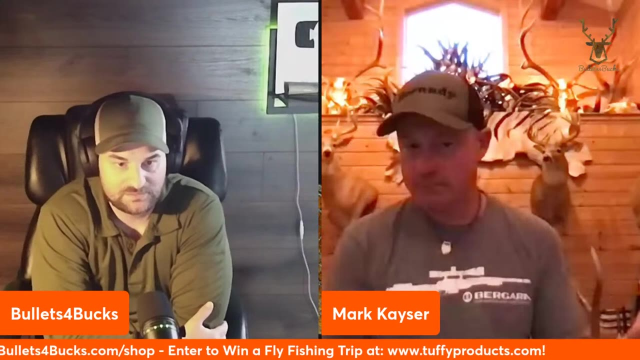 about- i'm trying to get your bear on it- which is the stainless steel carbon wrapped and then the carbon is actually intertwined with stainless steel threads to reinforcement. yeah, what so? and you've seen good accuracy out of it. yeah, i'm getting you know under a under a minute of moa off the sandbag. 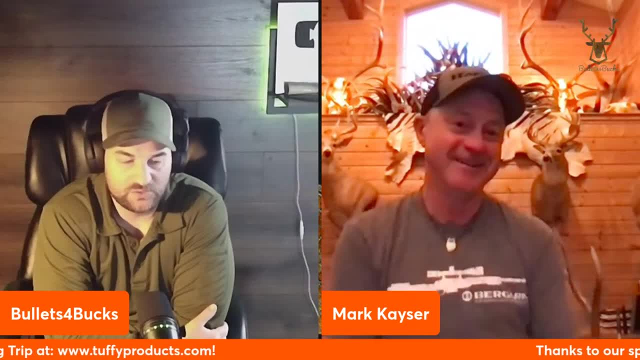 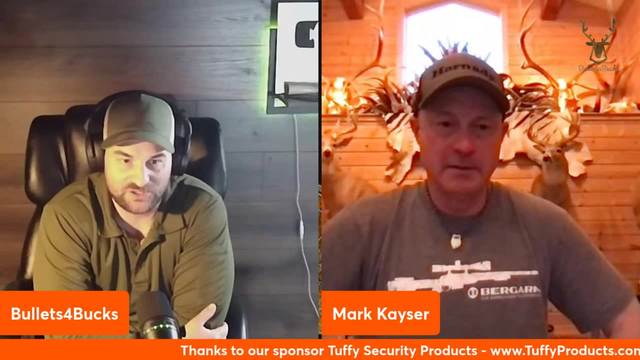 bench, with the bench that wobbles along, are you using, are using this? are you using sigs, uh sigs, uh 190s out of it like the sig ammunition? are you reloading? i'm just curious because i, i, i, i have mixed uh information on those. i'm 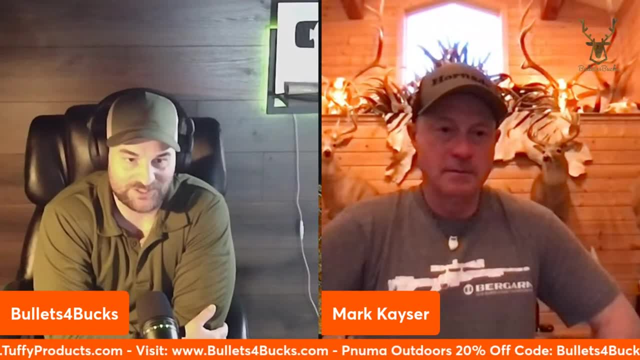 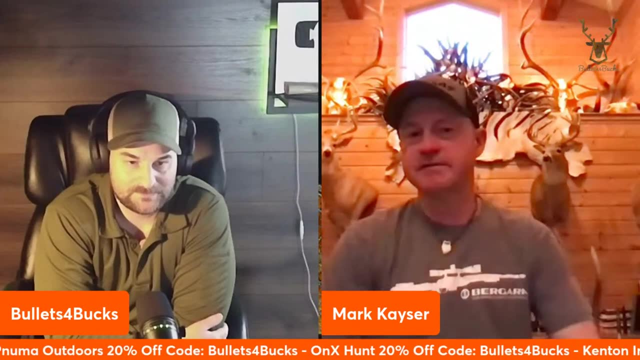 I'm not going to start an argument over it, I'm just curious. I mean, I'm information gathering, so I'm curious what Emory mission you've had success out of it with. Yeah, ELDX, Horn, ELDX. 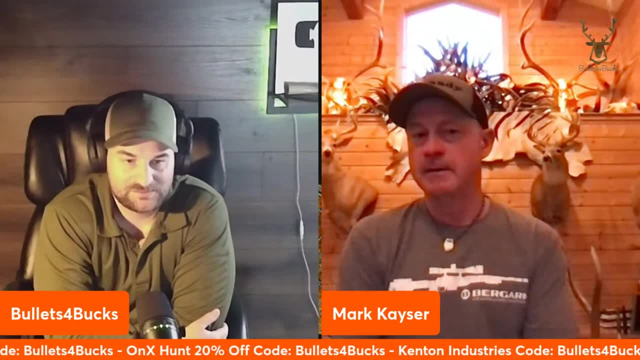 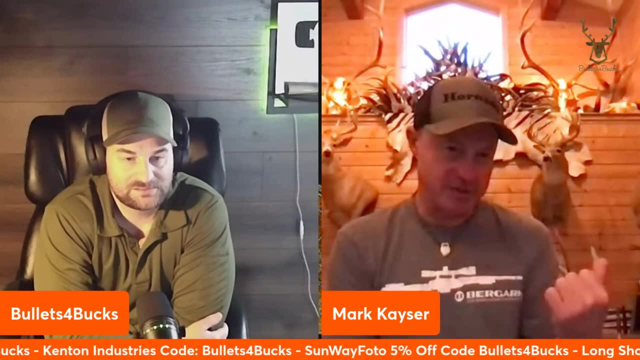 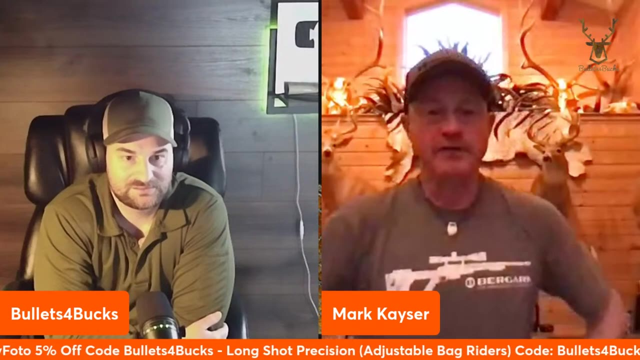 Oh really, Precision 100, 200 grain is what I ended up Now. I was shooting a Bergara MG Light the year before, which is a chassis rifle, DRL rifle. I like that rifle too and that's my backup rifle. 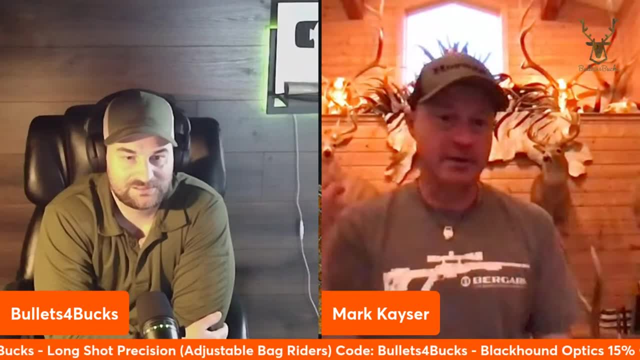 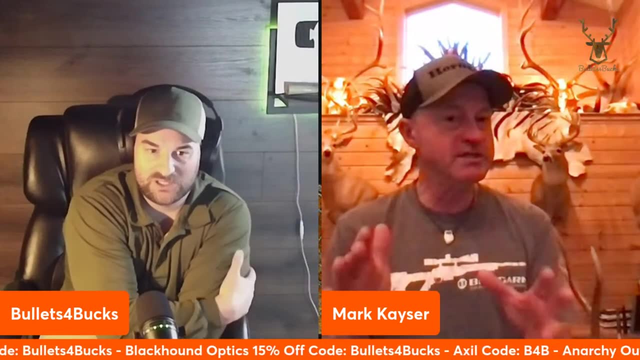 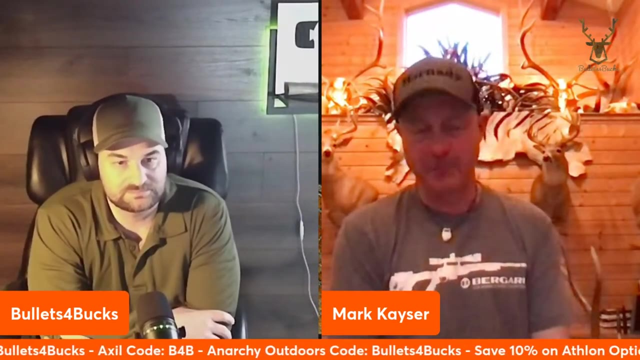 I carry that, as you know. if one would break, I got that in the truck, I can just pull it out. Holding stock right: Yep, Yeah. and magnesium alloy chassis: Yeah, for some reason that rifle loved the 180 grain CX bullet from Hornady. 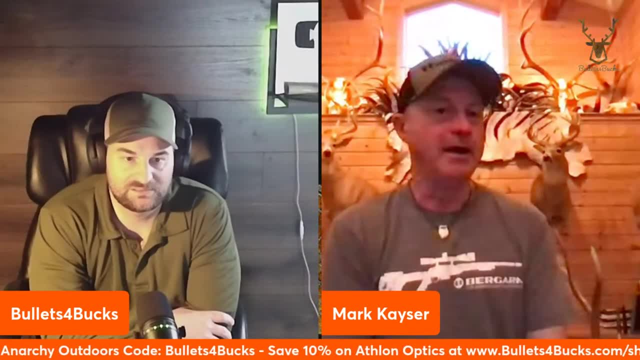 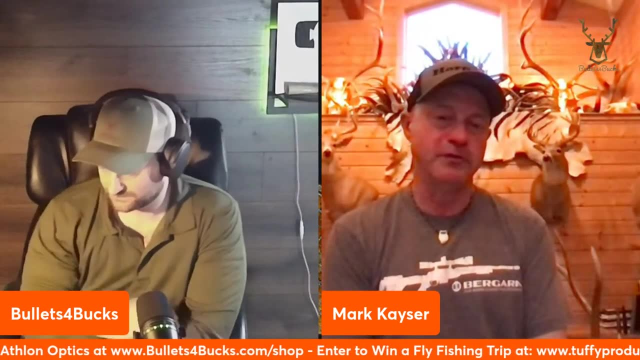 the monolithic. so I went with that, and that's why that question. you know, which one do you prefer? I don't know. I've seen deer and elk just tip over the same with both of them, so I'm not sure. 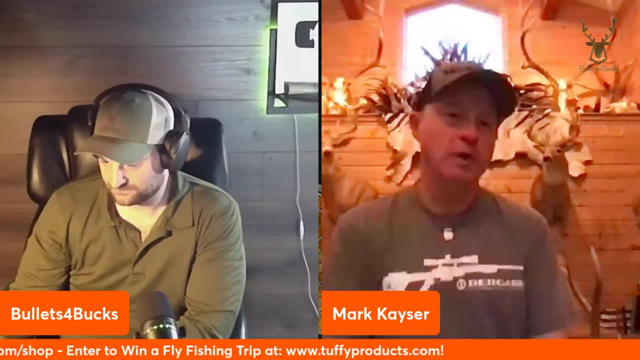 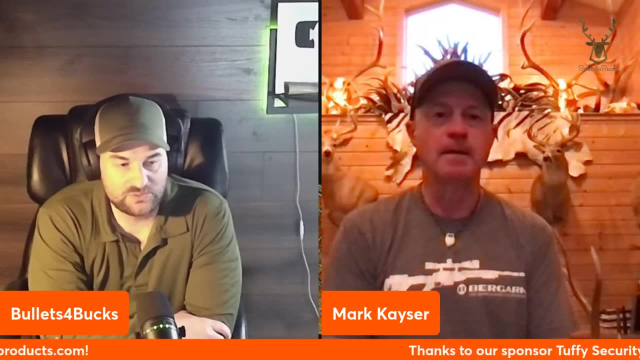 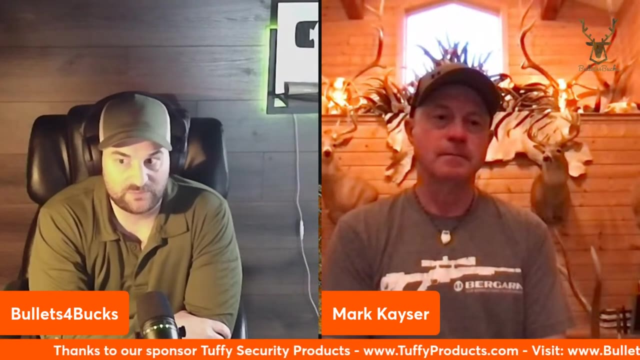 I'm not sold on either, one being an outperformer of the other. yet How did you like hunting with a chassis rifle? So I've actually never hunted big game with one. I've kind of generally steered people away from them because of, I guess, 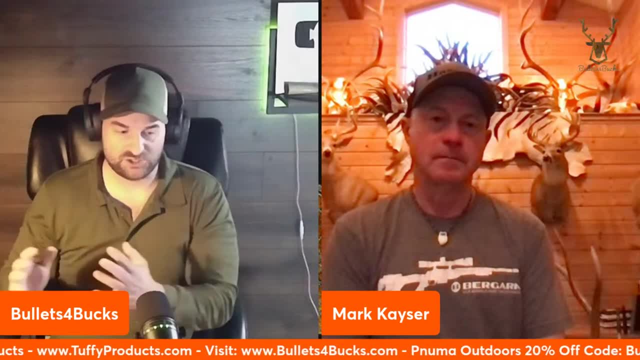 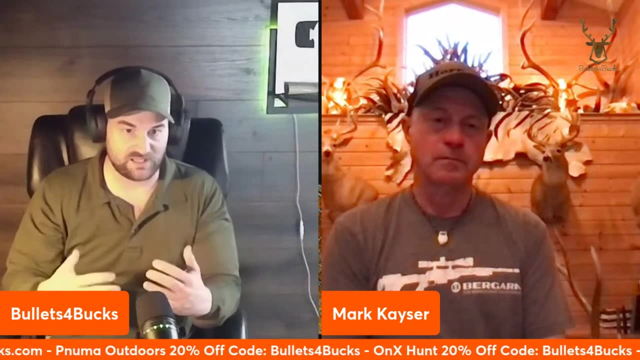 well, in general most of them weigh more and then in general a lot of them are so skeletonized that branches and stuff kind of can get caught in them and dirty and blah. I just different reasons like that. Did you like hunting with it? 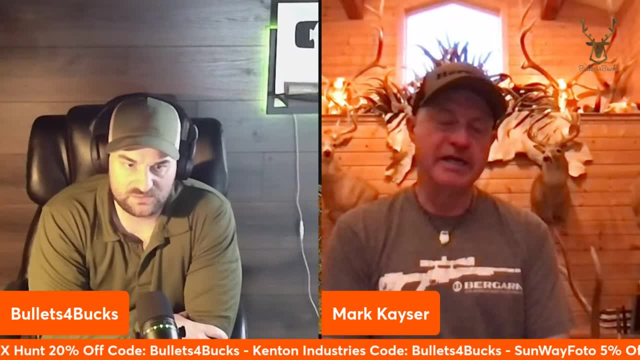 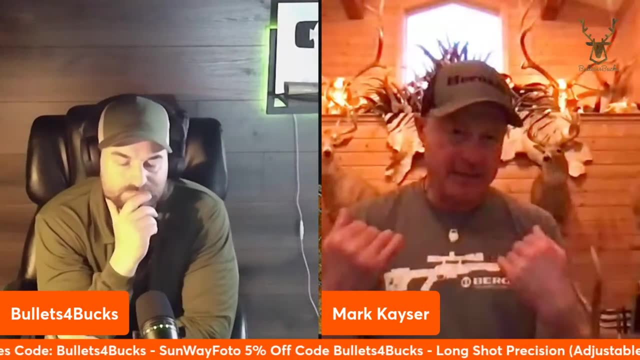 I think that one has a folding stock- right It does, and that was one of the things I really liked. So in the mornings when I go in, and late in the day, if I'm coming out and it's dark, you're after shooting light. 4F shooting light. 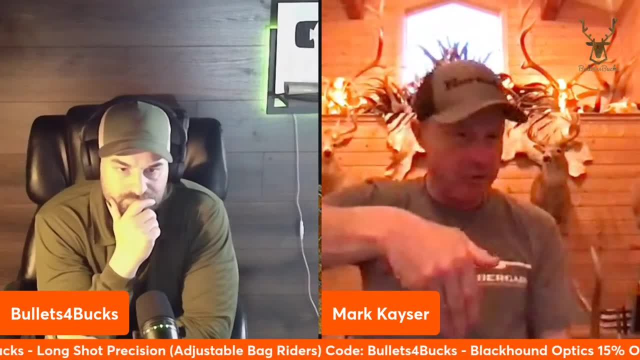 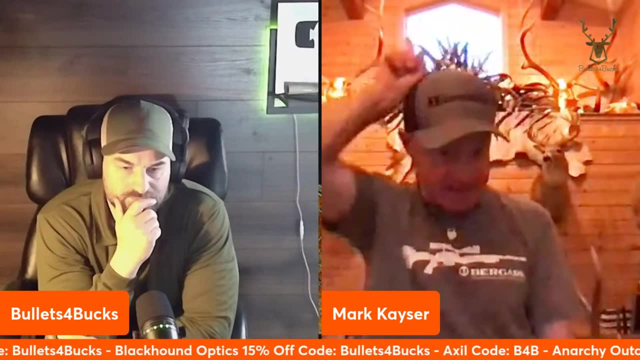 you can fold that stock up and then put it into, you know, your holder on the back of your backpack. Almost every backpack now has a rifle holder with straps, And that does not barely, if at all, go above your head. So when you're going through timber, 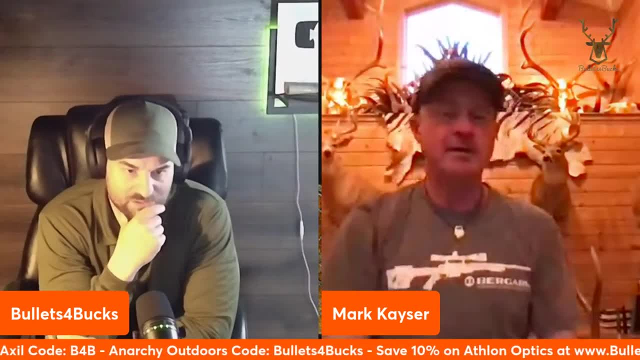 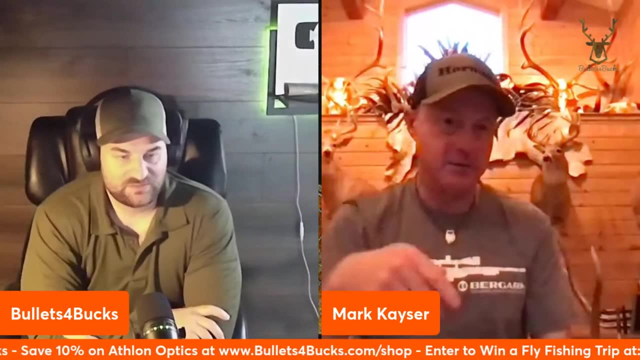 you don't have that rifle sticking up your catch Right. That's one of the biggest problems. I can't off too most of the time on a hiking interval to reduce that. See, since I've started hunting with cans, I've kept mine on while actively hunting. 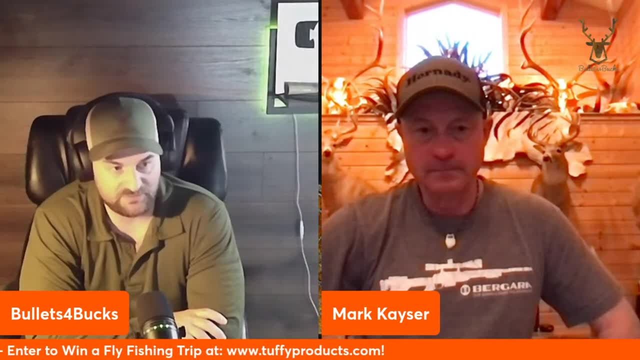 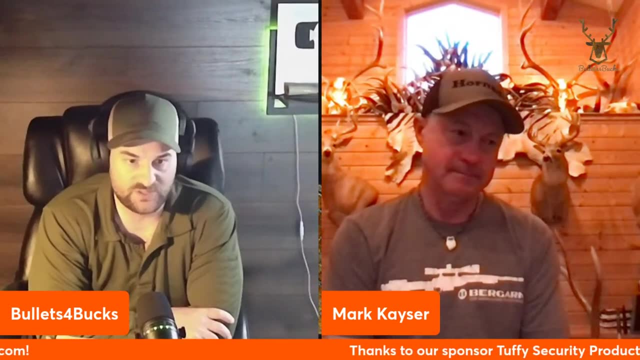 and I've started to really have I wouldn't say major issues, but obviously I'm like a flagpole and I'm hitting everything, And so because I have some pretty long rifles, I've been using them on. So I've been thinking, considering, after kind of being like no, no, no. 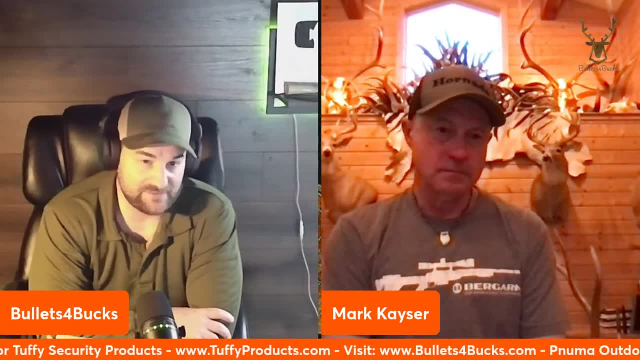 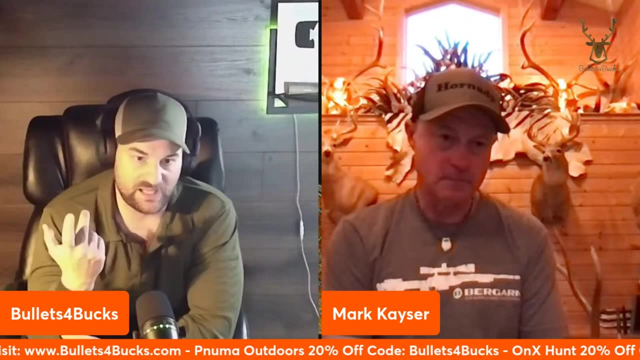 you know, trying an ultralight chassis. I've never done it for hunting, I don't have one right now, but like an MG light or a SIG Cross or the new SIG, was it Sawtooth? the Magnum version just is coming out of the Cross. 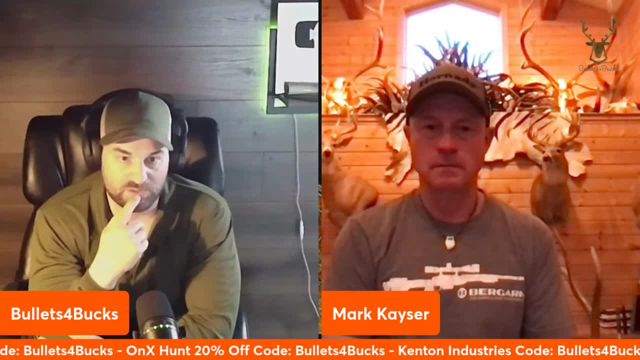 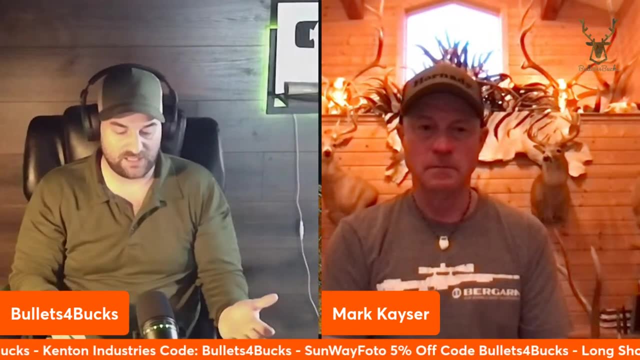 or something like the Fixed by Q, although the price point on that one's really high, But something you know: ultralight, because that ability, Yeah, to leave the can on, fold it and then have that really short overall length. 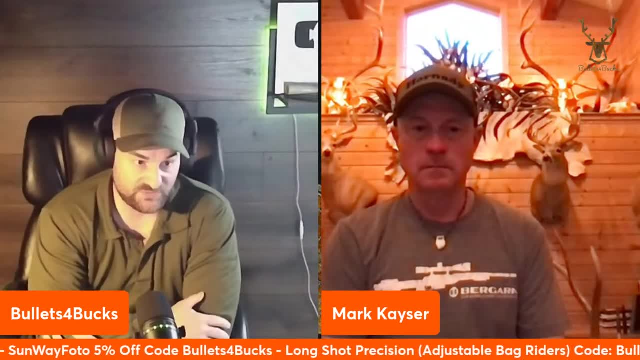 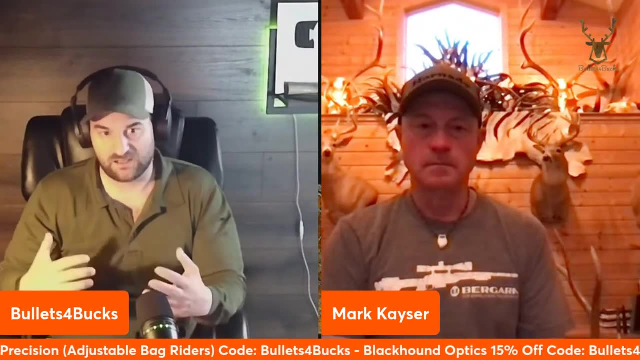 And the ergonomics on a chassis. I've always at the range as far as like feeling comfortable and shooting accurately. I've always loved the ergonomics of a chassis. I just haven't liked the idea of you know the, maybe the weights or the. 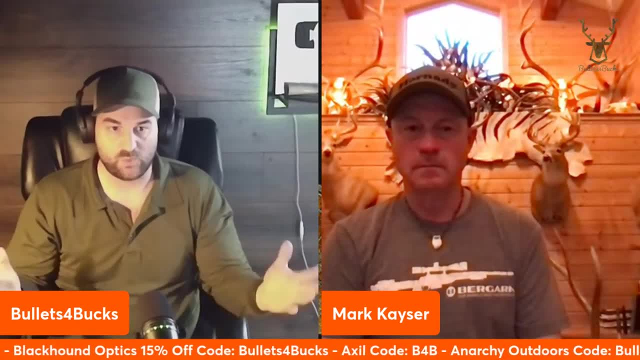 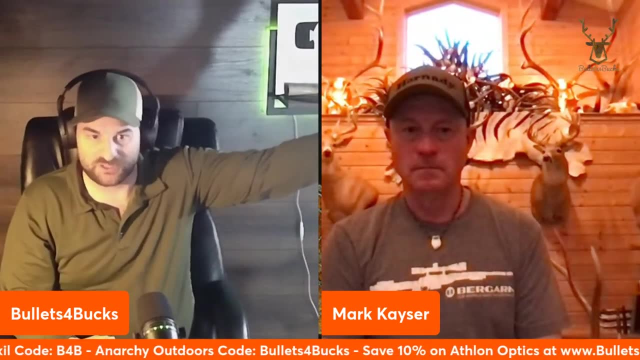 maybe a lot of ways branches could get caught on them when. but if you're cutting down the overall length, I mean my barrel and suppressors getting caught on branches anyways with the more traditional styles. So I guess, I guess I'm starting to reevaluate where I'm at on that. but 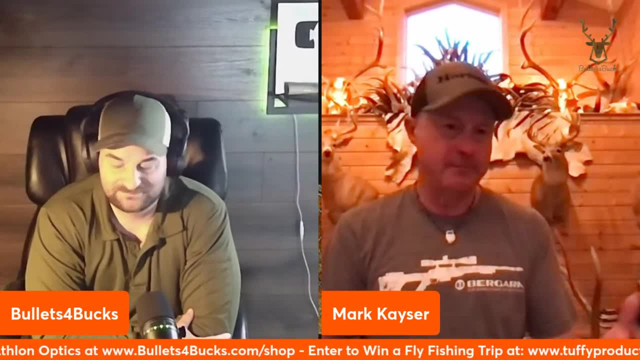 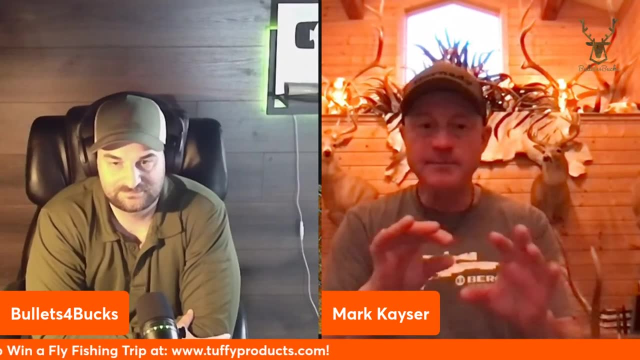 Well, the regular PRS rifles, you know standard, they are heavy, You know they go up to 18 pounds or whatever, But like Bergara's MG, and now they got the MG Microlight, Yeah, So you know they're pretty lightweight rifles. 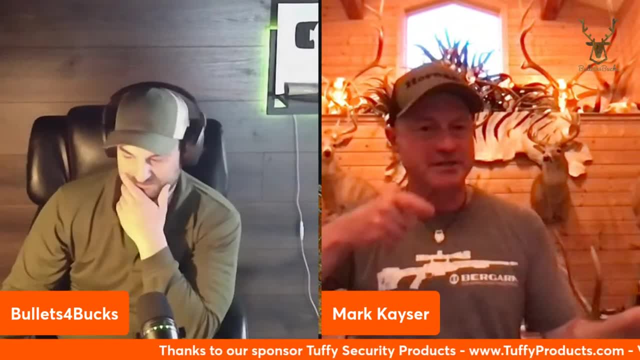 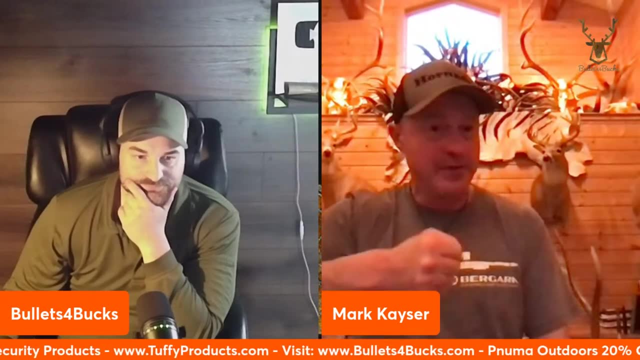 Oh yeah, The thing that really freaks a lot of people out is just the feel It's just, it doesn't have. you know, it's got a standard, It's still grip. I mean it's a, it's a standard pistol grip. carbon fiber magazine. 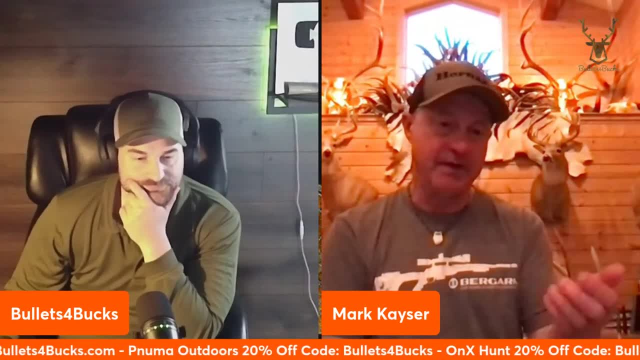 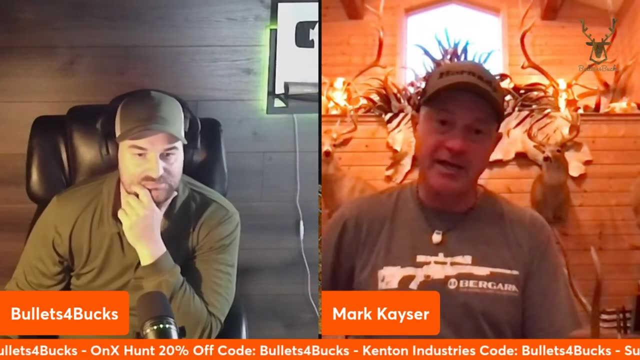 which I love, a magazine on any rifle? I I'll just say that I'm not. I just think there's so much easier to clear and make safe, you know, and have an extra magazine in your pocket, and I've only needed it once- uh, elk hunting- but when I did need it I just pulled that extra magazine. 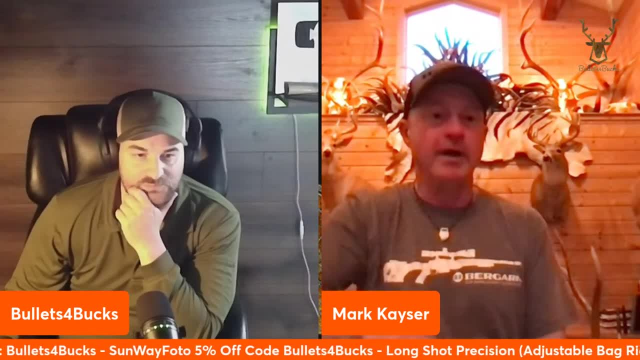 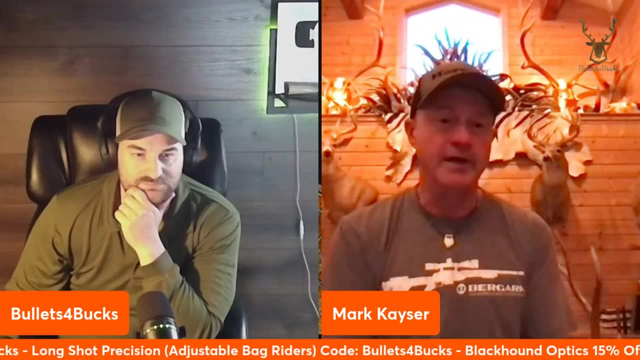 slapped it in and I was, you know, shooting again where, trying to feed it into you know top down feeding. Uh, it gets to be a little hard or slow on a rifle. So uh, I don't know. 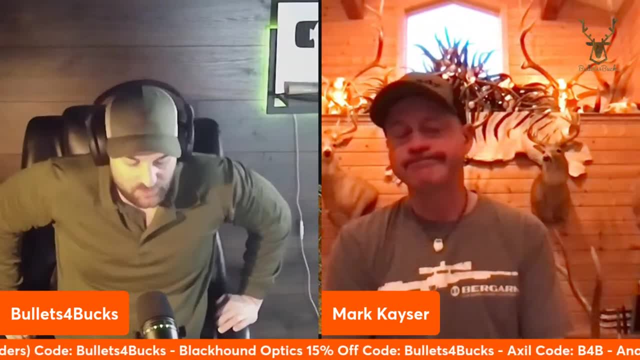 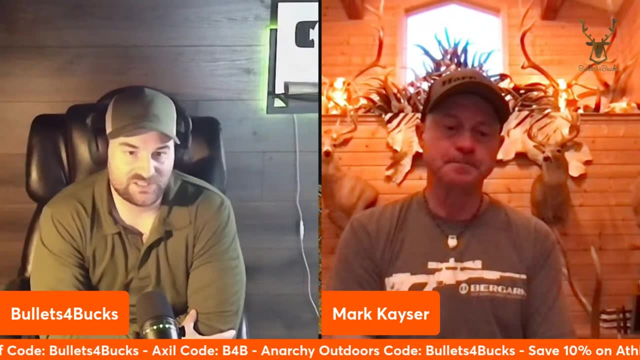 I go ahead. Well, the market, I mean the market, technology in the market. it's so competitive, It's constantly changing, a little bit at least. And so, like I know, when I first told people, don't like initially, don't go hunting with 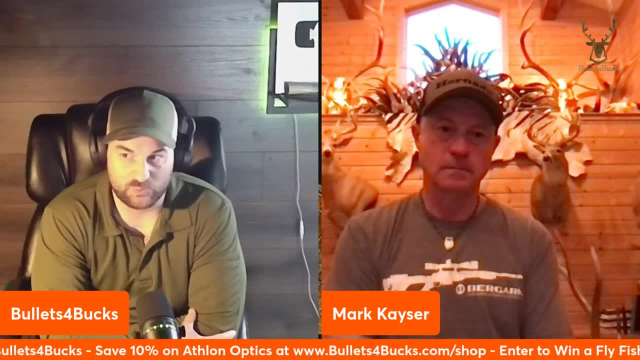 a chassis. if you're going like on Alcon, it was also because, like there really was almost no options and it was like the RPR, the Ruger precision rifle at like 10, 12 pounds, Yeah, Dressed out. 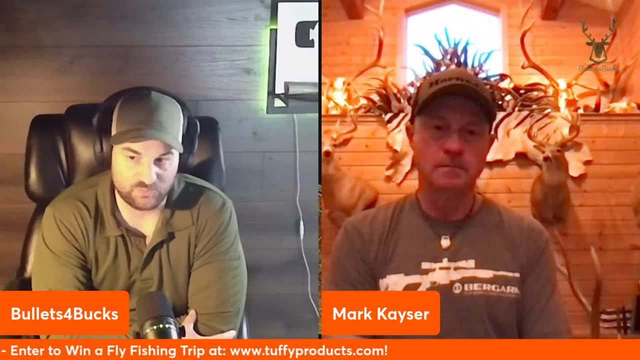 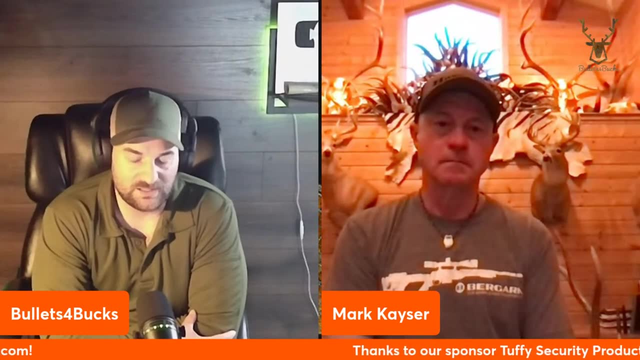 So I mean, back then it made sense, but now that there's there's just more and more ultra light- uh- options with folding stocks coming on the market, it makes sense to reevaluate it as well. Um, so the ergonomics of my rifles are a tool. 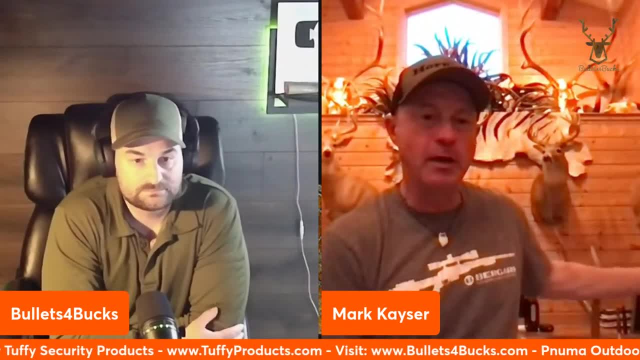 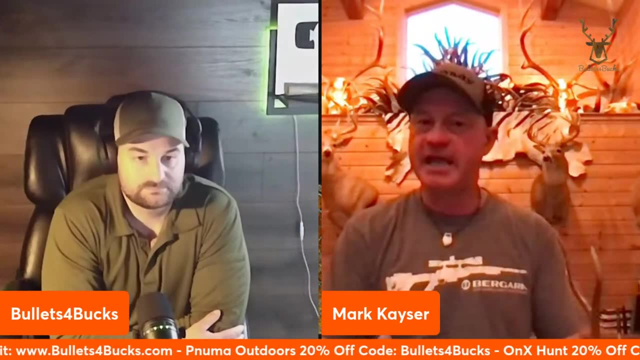 I don't have. I can reach in here and start pulling guns out if you want, but I don't have one gun in there that I can't just throw down on the cement and walk away. They're all Stanley hammer type of things there. 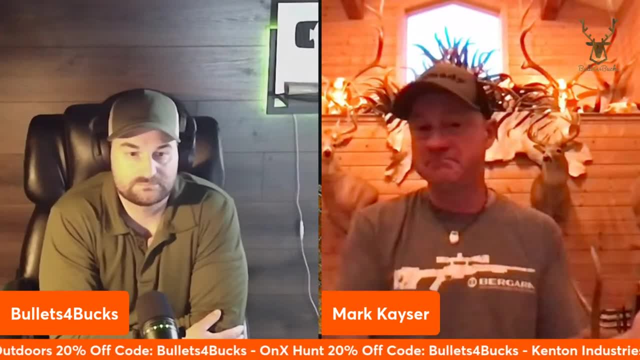 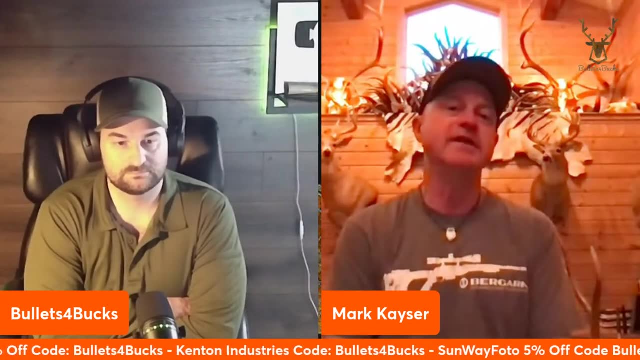 None of them are going to be an heirloom to my uh and my son. his guns are the same way, maybe because he grew up under me. but, uh, I just I like guns that are tools that I can beat the crud out of them. 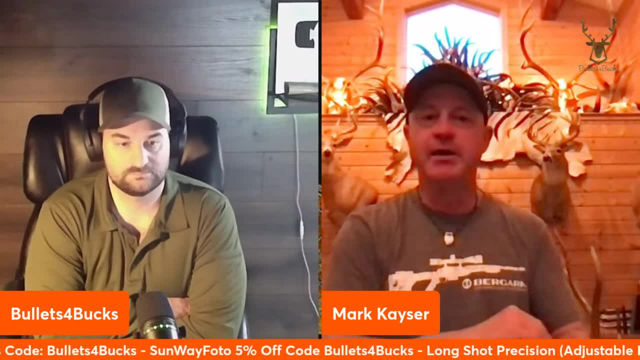 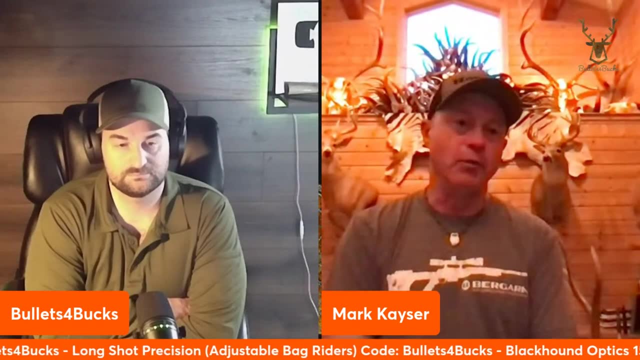 I can lay them down on a rock and they get scratched up, I don't care. Uh, so to me, I just want function, and my function now, as I get older, is lightweight. I just want a lightweight rifle. I'm not carrying a base rifle that weighs nine, 10 or pounds. 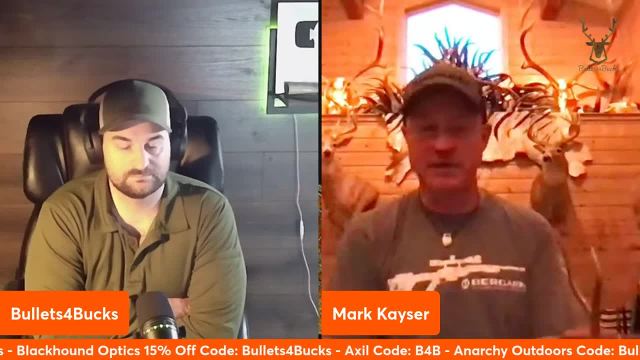 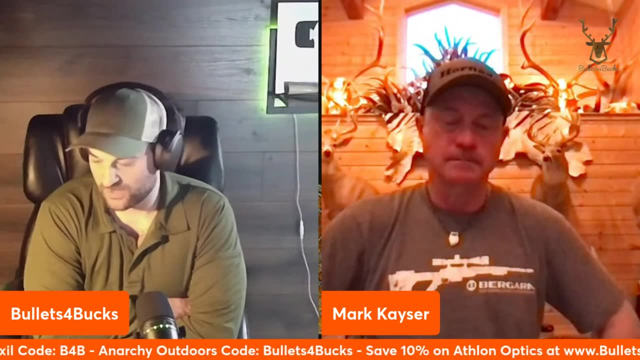 I'm not carrying a base rifle that weighs nine, 10 or pounds without the scope and ammunition, everything up in the mountain, or I'm just not going to do it. Right, Right, Yeah, And I guess one. I guess we'll close here pretty soon. 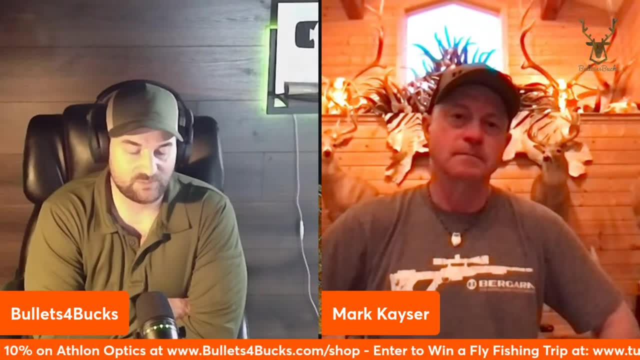 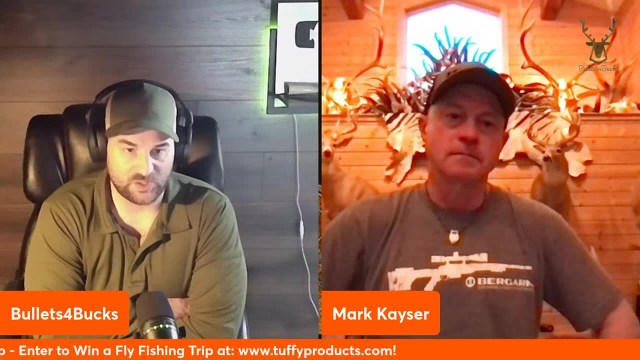 Just like I guess we can close with this question, Like: do you have a preference or what would you recommend to people? uh, for Western health, Western elk hunting as far as a caliber like seven REM, mag, 300, PRC, 300, wind. 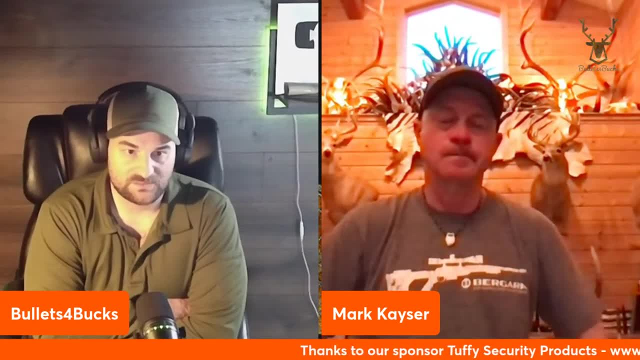 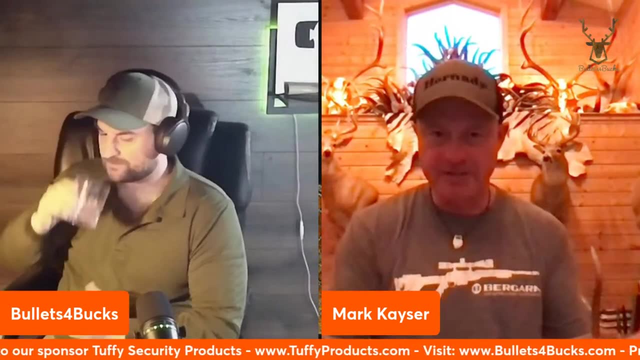 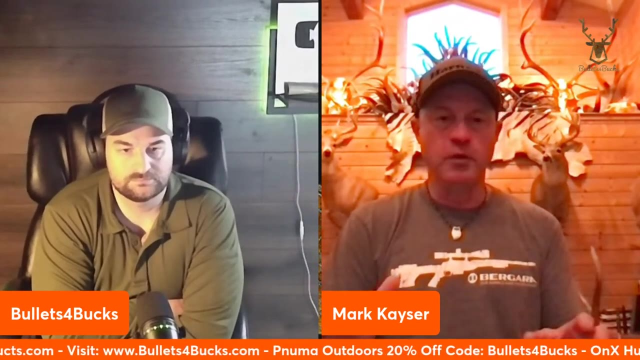 like kind of a do all uh cartridge. what would you recommend for big game? Well, I think it's hard to beat the seven known seven PRC right now. I mean, I it just for, uh, it's ballistic coefficient, uh, you know it's performance. It. it rises above the crop out right now. That being said, if you're going to get a rifle and say, maybe go to Africa or Canada or other places with it, You know a little more exotic, maybe even South America, for red stag, it's hard to beat. 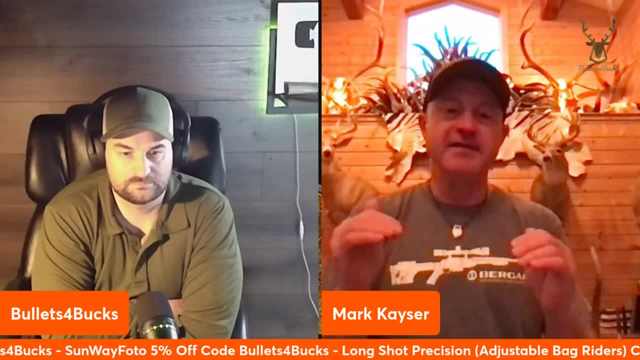 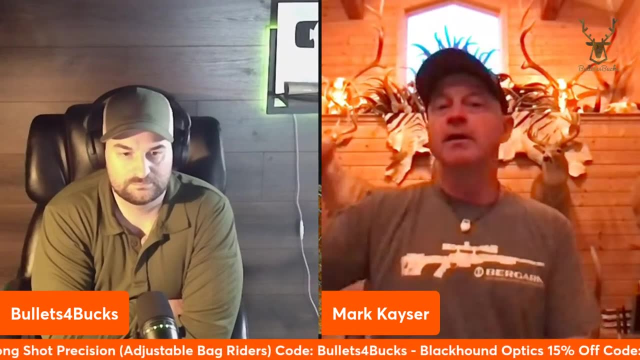 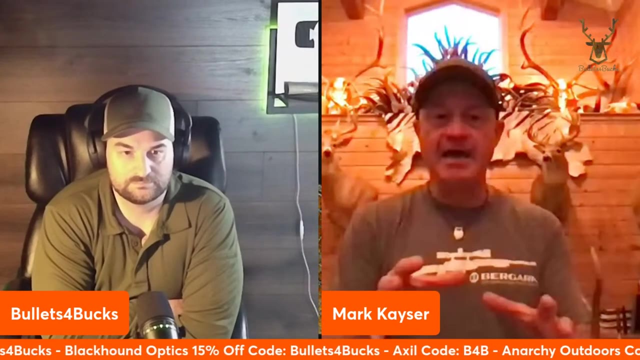 the 300 Winchester Magna, because that caliber is known worldwide And you can uh go into a sporting goods store in Johannesburg, uh moose jaw wherever and get that ammunition if you would need it. So I like that, but I really like the seven PRC. That being said, I like the 300 PRC And I shot a lot of my first uh critters For the years when I started out with the seven millimeter Remington Magnum- uh, those are my favorites. I don't like shooting stuff with small caliber. 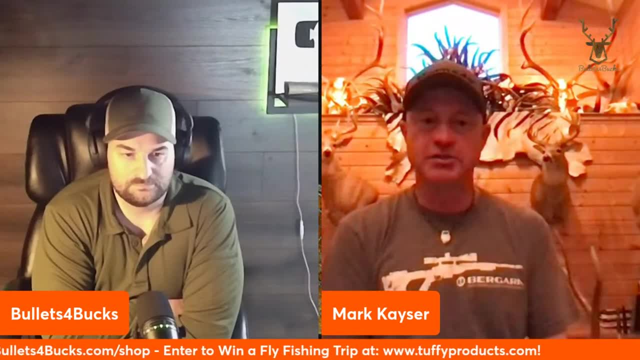 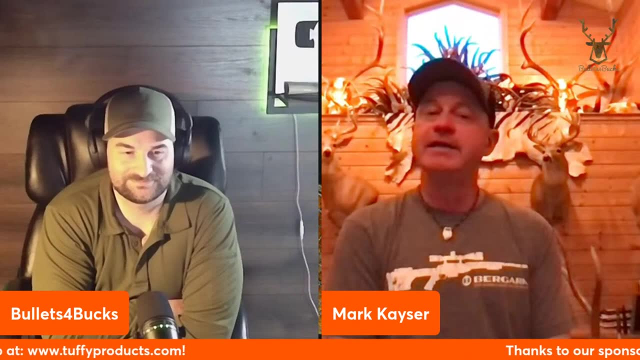 I do have several six five Creedmoors and I know guys shooting elk with them And even the six five PRC. uh, I just again especially elk And I think that was your question to begin with: elk and and a big Western mule deer. 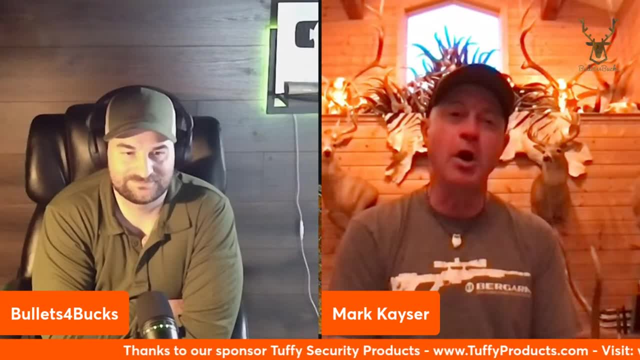 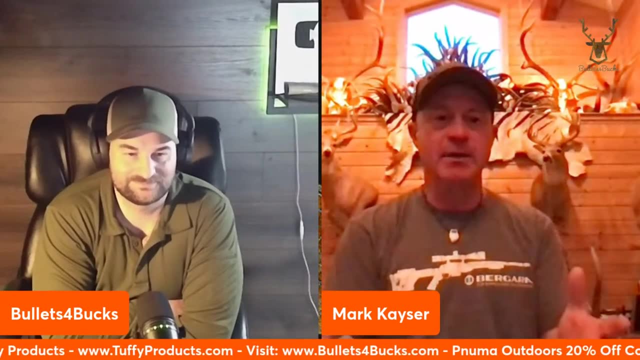 a big Western whitetail. Those are big critters. You just want to hit them hard. What would you rather? lose A package of meat or lose an animal? I mean so that everybody says, oh, it's just too much gun for an antelope. 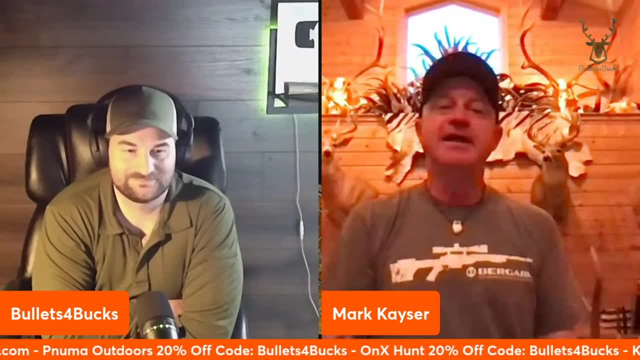 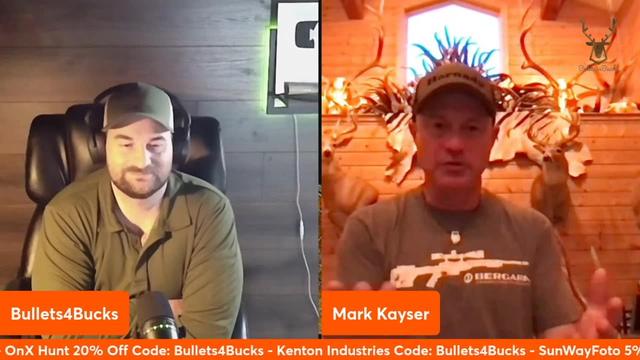 I shot a lot of antelope with the 300 wind mag And it's like, yeah, maybe it is overkill, but I feel comfortable with that caliber. It shoots right for me. you know, usually a 300 or a seven or whatever. 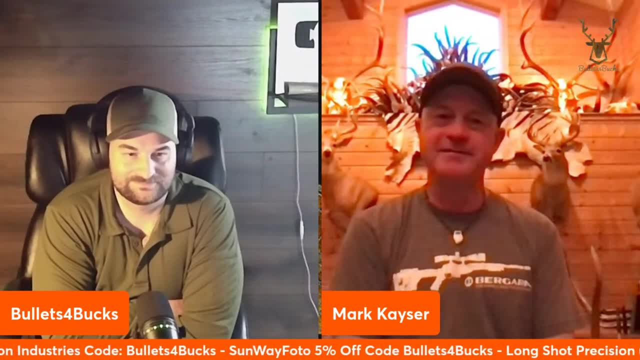 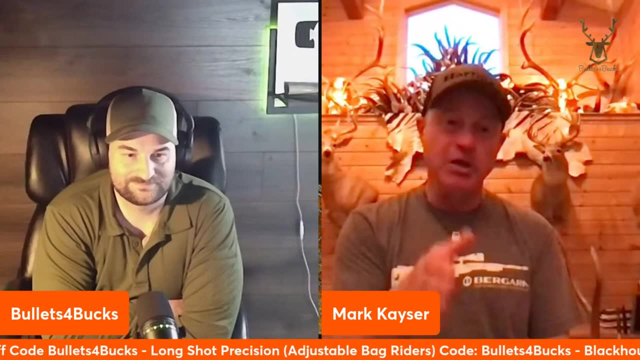 And uh, okay, I'm going to lose a little meat out of the deal, but you know what Critters going down it's, it's anchored And uh, and even, Even if I hit it bad, they know they got hit with that. 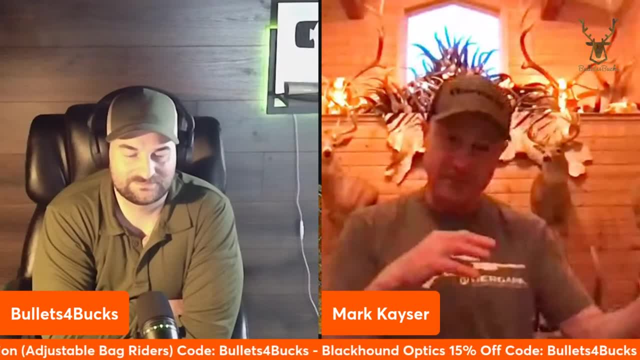 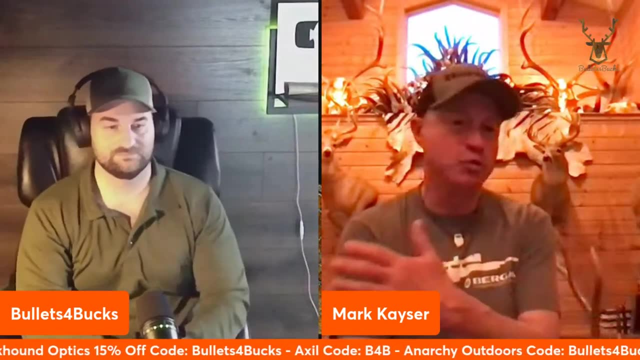 And usually you've got a chance, especially suppressed, quieted, Uh. but when they get hit with a 200 grain bullet, 180 to 212 grain bolt, whatever they're getting hit with a lot of energy, typically under four or 500 yards. 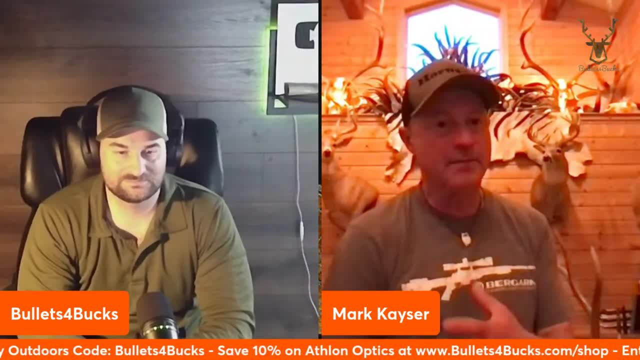 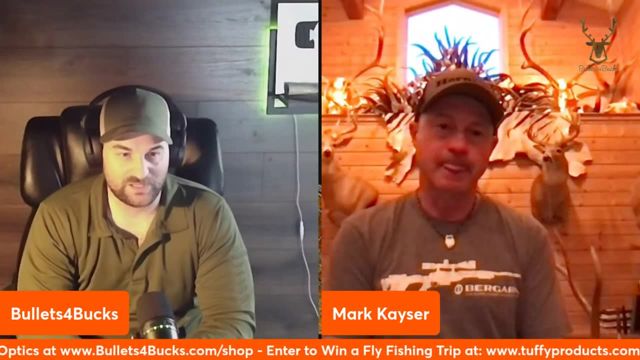 So uh it, it, it shocks them. plenty of time for you to work the bolt, get a second shot in. Yeah, I recommend 300 wind mag. That's that's my pick for that question. uh, all the time. 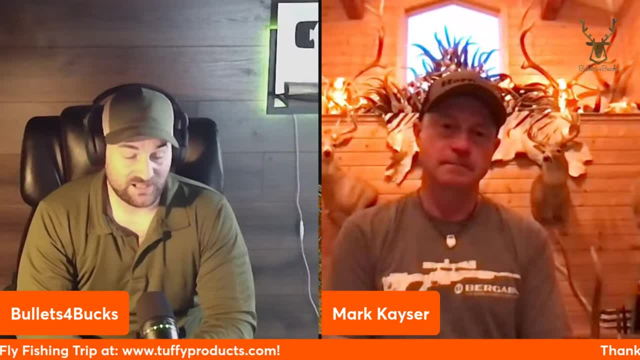 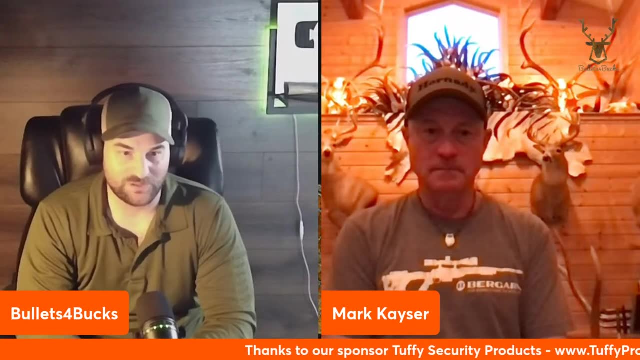 I think, um, I shot, I have shot elk with six, five Creedmoor, And then the more, the more I've hunted, the more mistakes I've made, the more human you realize you are. uh, you know fatigue and environment and weather, uh, has a large effect. 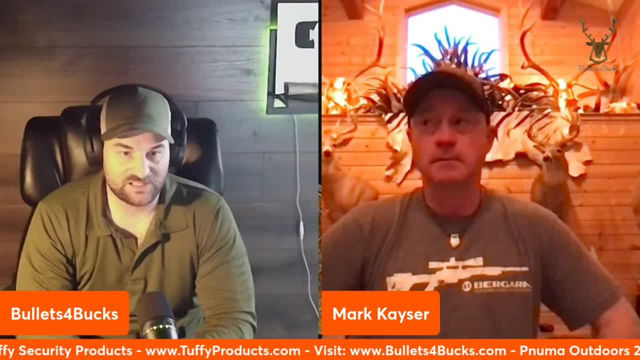 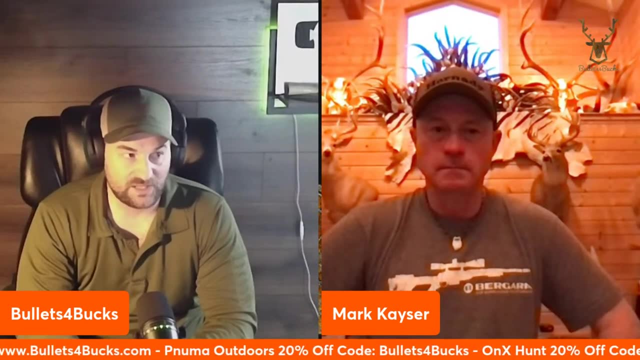 People shooting at the range is different than shooting an animal, obviously out hunting, And so, at you know the more experience I've gotten, it's like no, I want a magnum for everything, basically bigger than a white tail. 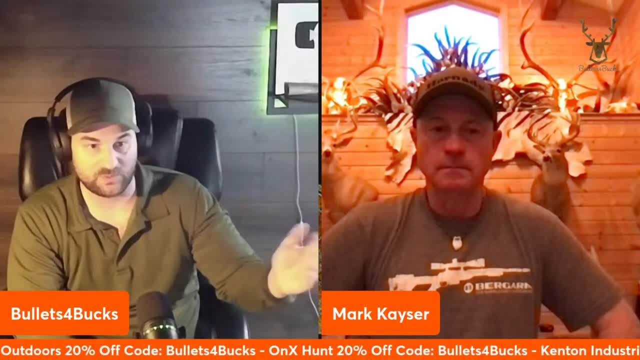 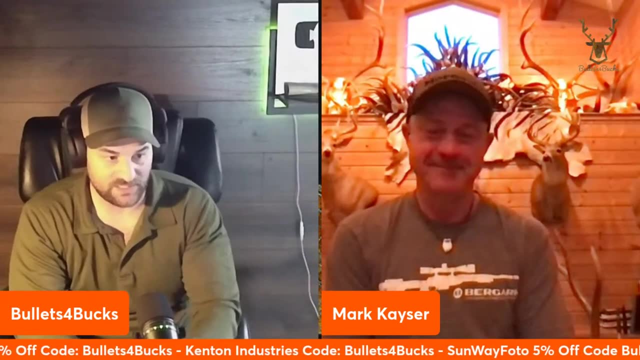 And I'm not, and I've shot uh antelope as well with the 300 wind mag And it's like you can't get more dead. It's not going to hurt it And you can shoot. if you shoot an antelope in the chest cavity anyway, you're probably. 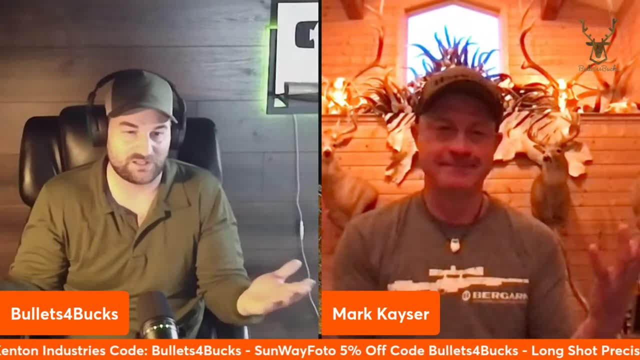 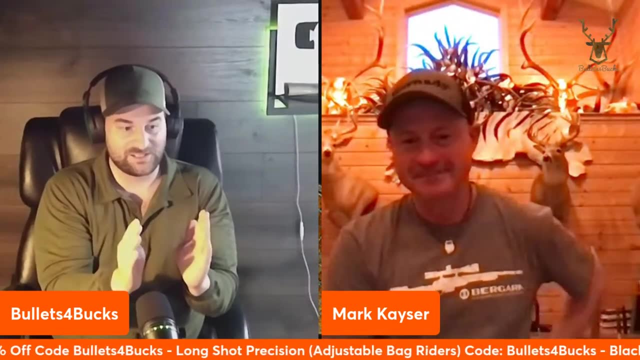 not going to destroy any of the meat. anyway. If it's a 300, it's still not going to destroy any of the meat more than a six, five or a six millimeter. So, and plus if you, if you have one gun that you're using for everything, big game. 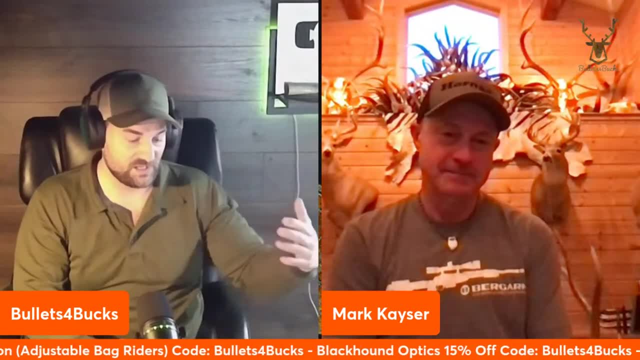 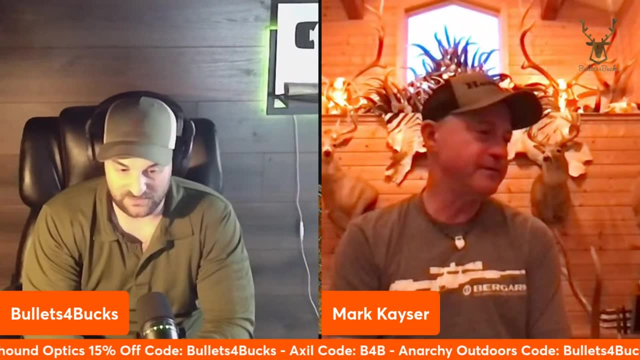 you're probably going to be really comfortable with that one gun too, And so that could also make you more confident and more confident. Shoot better stuff like that. So I totally agree with with you on on that sediment, So, but really good having you here, Mark. 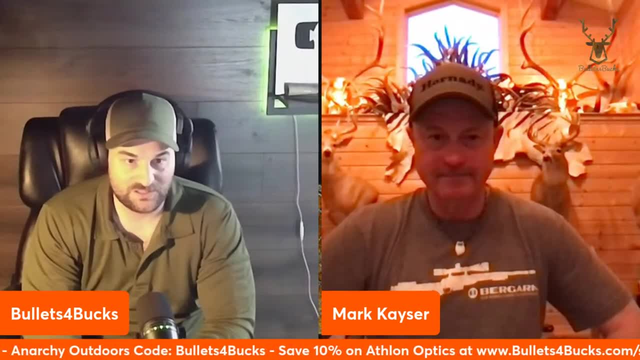 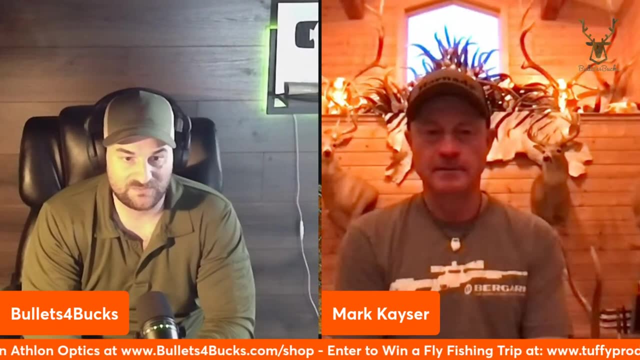 And uh, I look forward to talking to you more in the future. And uh, thank you guys for stopping by and viewing this live stream. Thank you to my sponsor, uh, for the podcast Tuffy security products, and we'll see you. at the next live stream. Have a good night.